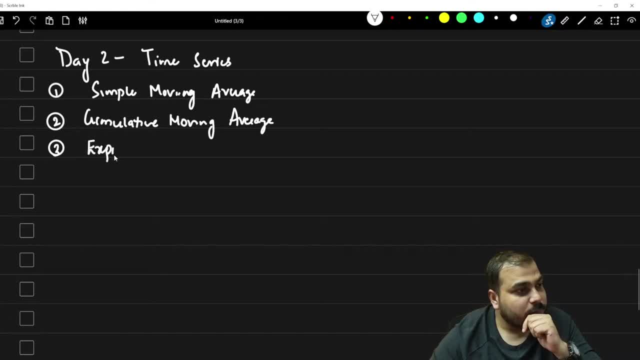 moving average. Then we are also going to see exponential moving, EWMA, moving weighted average, EW: Exponential weight moving average. Fourth one: if this is done, then exponential moving average. These all things we will see with the help of excel sheet plus coding. 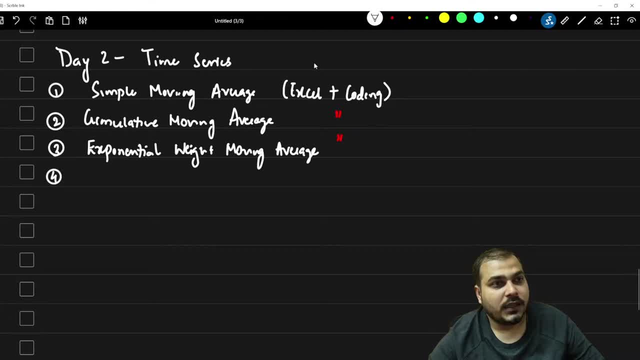 And same thing will basically be for both of them. And then we are also going to see moving average. Moving average- We will separate moving average. Try to see the formula. And probably we will also probably see ACF autocorrelation plot. 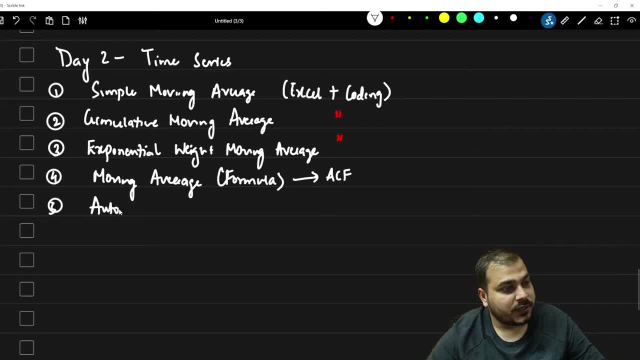 And fifth, we are also going to see autoregressive model, And here we will also see some plots like PACF, partial autocorrelation And then all of these things we have defined in the next lecture. So next let us just see the exponential weighted moving average of EWMA. 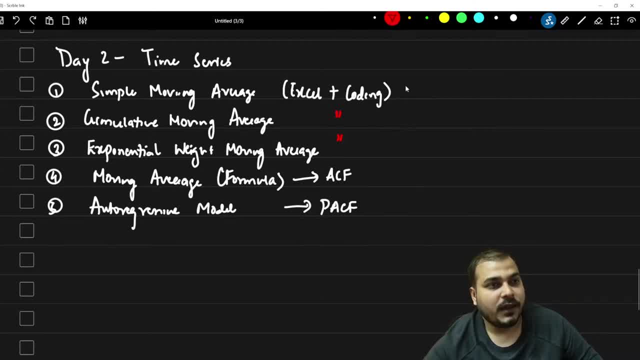 So all these things we are probably going to see today, Because I guess in 1 and a half hour we will be able to calculate this. In tomorrow's session we will try to solve EWMA model, because here only this is my MA- 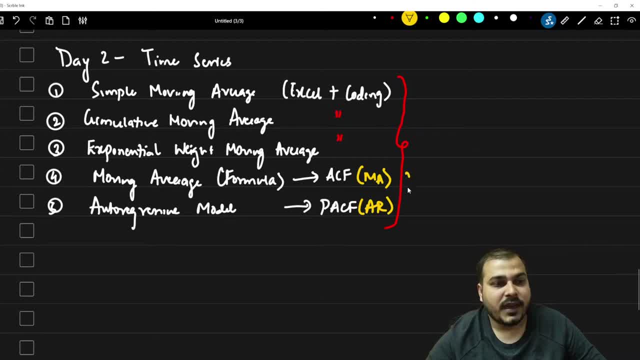 this is my AR model. So if I combine both these things it becomes ARMA model. So in tomorrow's session we will try to see EWMA Plus different, different models like Arimax, Sarimax. so all these models we'll try to see tomorrow. 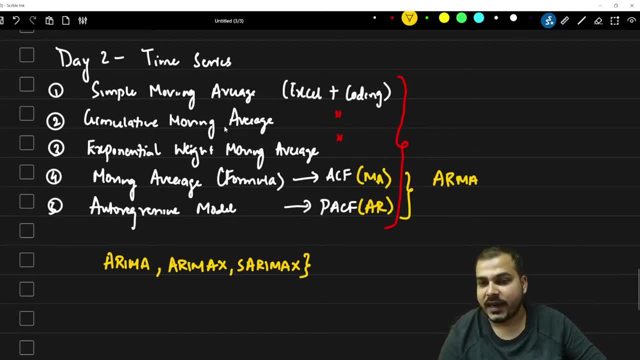 Okay, but here today we are mostly going to understand most of the important things. Probably, I'll try to show you, with the help of coding also, and with the help of excel sheet also, how you can probably be able to do it Clear, Okay, Shiva Kumar says: can you suggest some books for learning time series? 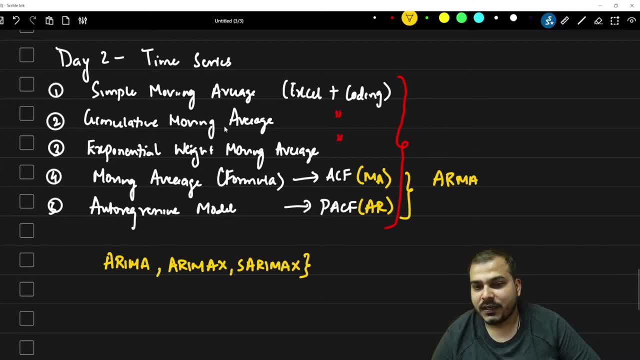 There are many books as such guys I definitely I don't know like which to follow. All are written in a proper way. Okay, so hit like and just let me know whether you are ready so that we can start. Is my volume low? Let me check it out. 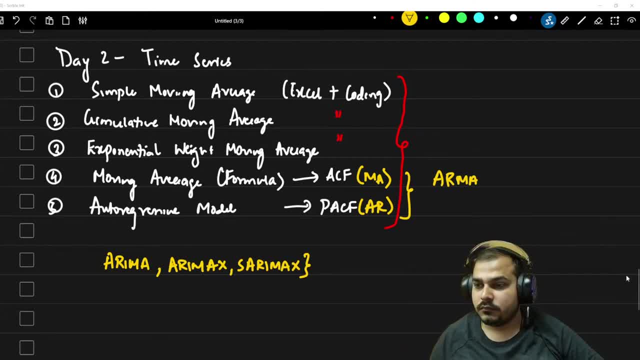 My volume is not low, Fine, Is it? Hello, Hello, Hello. My volume is fine, right, Hello. So, guys, I hope it is audible. I'll just try to reduce a little bit. Fine, I think it is perfect. 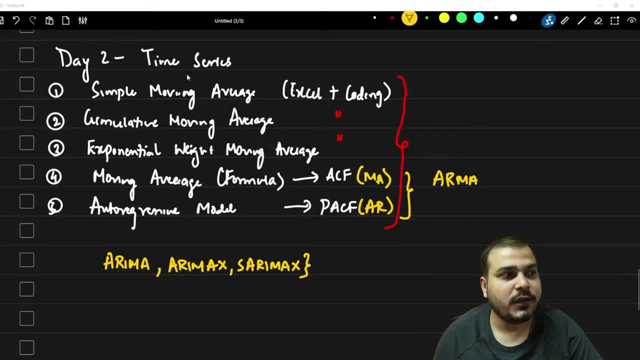 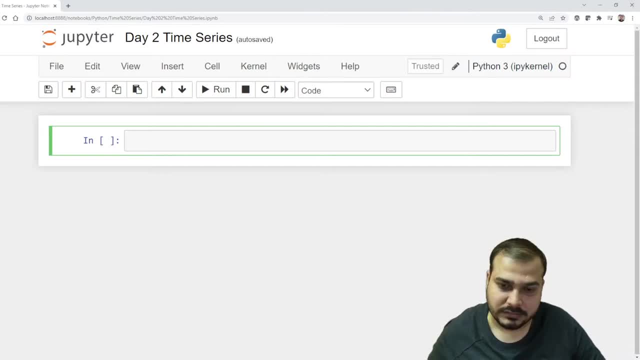 Okay, so let's go ahead. Let's try to first of all see simple moving average. Now, as usual, let's start with. So let's go ahead. Let's try to first of all see simple moving average. In the simple moving average, the first thing. 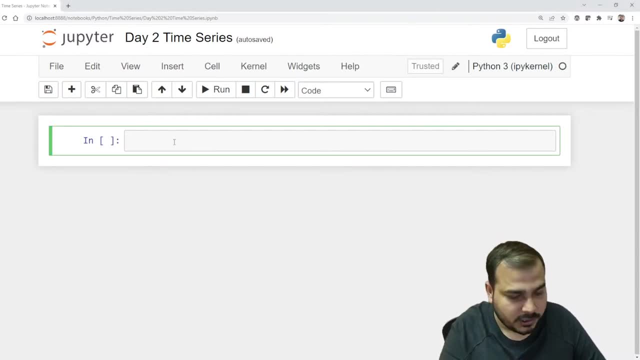 is that again, we will take a specific data set and probably do it. We can take the Tesla data set, what we have actually done yesterday, So I hope everybody remembers which all libraries we have specifically used. But did you do the assignment that I had? 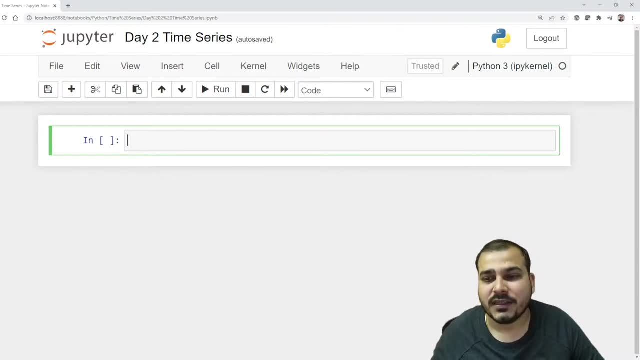 actually given yesterday. Just let me know, Okay, whether you have done the assignment. So till then I'll just import all the libraries. I'll say import pandas, data reader, as pdr and then import pandas as pd and from datetime I'm going to import. 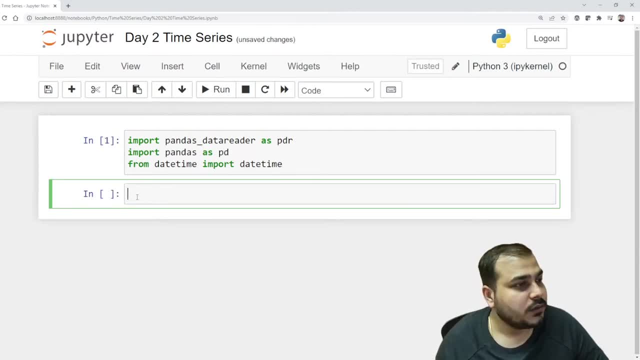 datetime. Okay, So these three libraries I'll definitely require. So I'm just going to read my Tesla data set and I'm basically going to do pdr dot. get data yahoo. I can basically take it from data yahoo. That basically means I'm taking the data from. 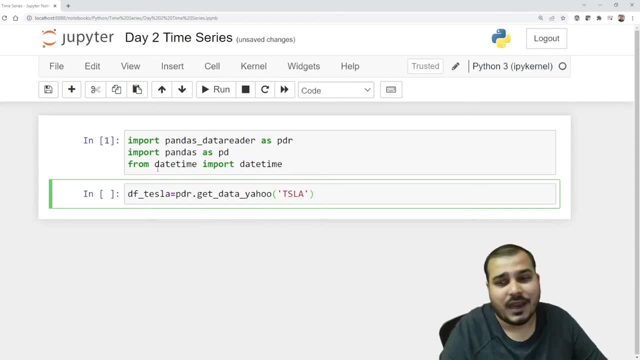 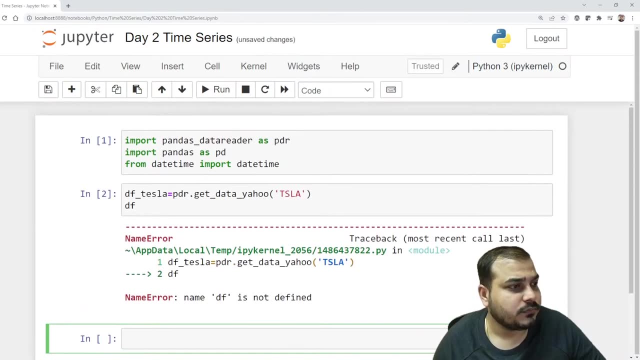 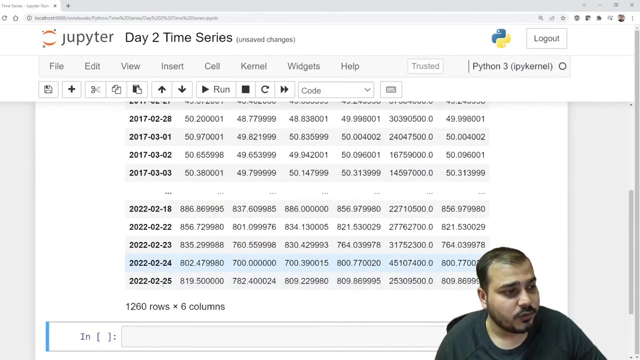 yahoo finance and this will probably give me the last five years data set. So here you can basically go and see df- So sorry, df underscore Tesla- and here you'll be able to see all my data is there from 2022.. Yesterday we were working only till 24. 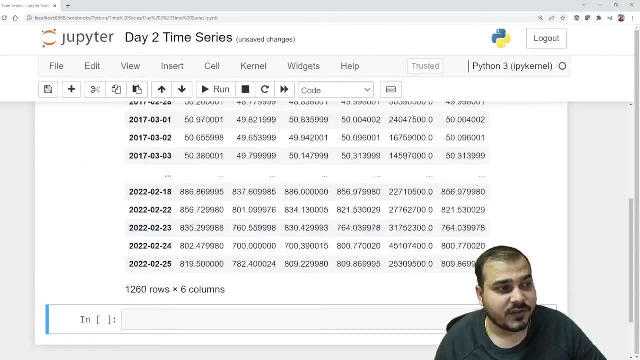 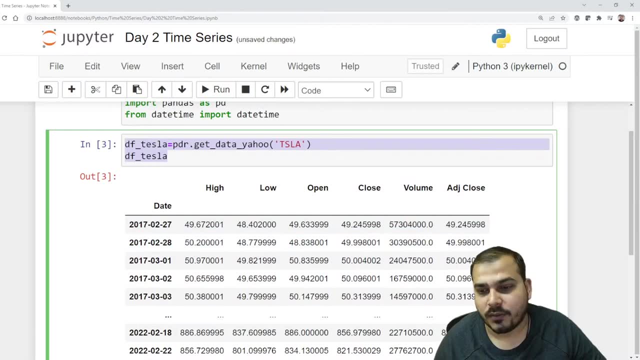 but today we can see till 25, 25th date. we have all the data and today is 26th. Probably in US it is 25th. So here you can see all the data that is required. Okay, Now let's go ahead and let's try. 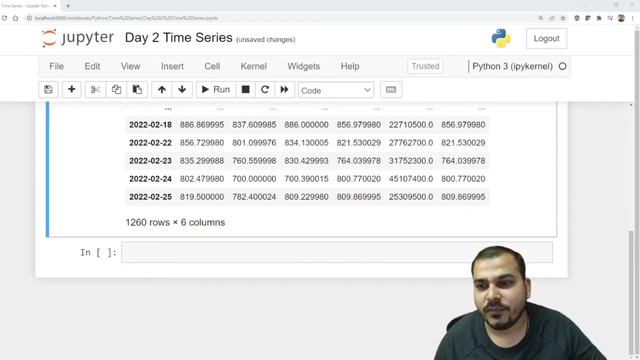 to cover up all the topics that I have written over there quickly so that you'll get an idea about what all things we can basically do. And before that, yeah, we have done the assignment properly. Great, Okay, So perfect. So let me make some cells. 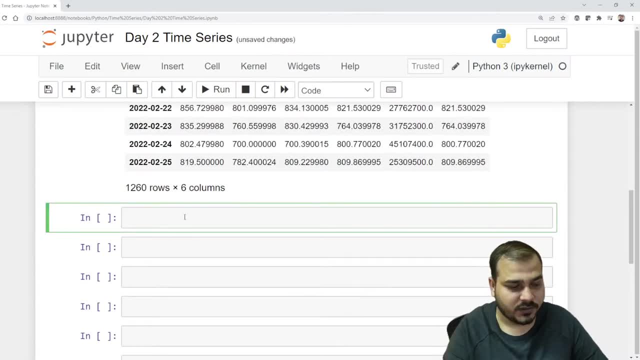 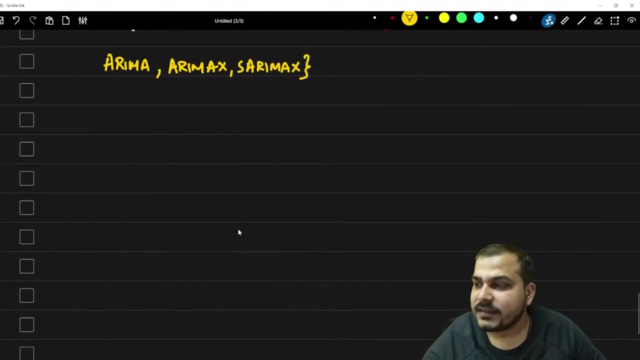 Now, first thing. first, we really need to discuss about something called as simple moving average. Okay Now, what exactly is simple moving average? I'll just try to show it to you with the help of notebook, where I'll specifically write. Let's consider that. 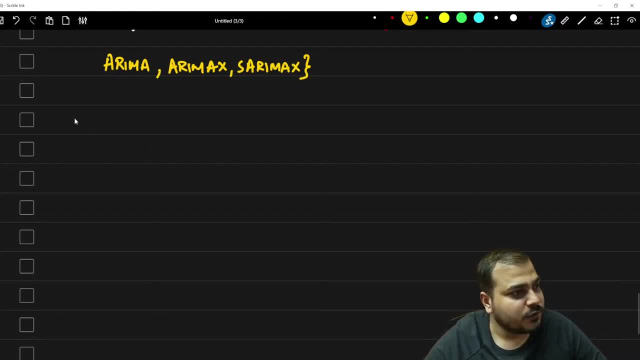 okay, Let's consider that over here. Suppose I have my data sets Right, So I have my open column of my data set. Let's say that I have data's values like 12,, 13,, 15,, 17,, 11,. 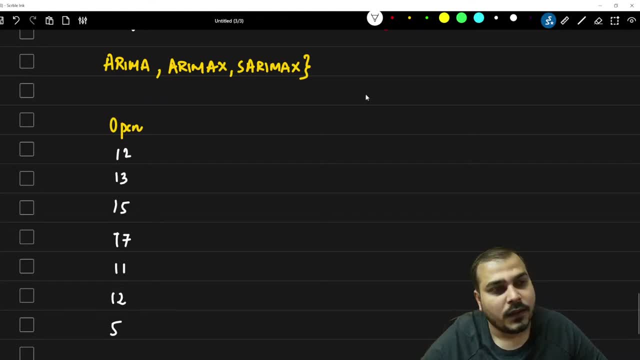 12, 5.. Okay, So yesterday we had used a. yesterday we had actually used something called as rolling function, And many people were actually getting confused. what exactly is this rolling function? Okay, Now, here I'm actually going to say what exactly is this rolling function. 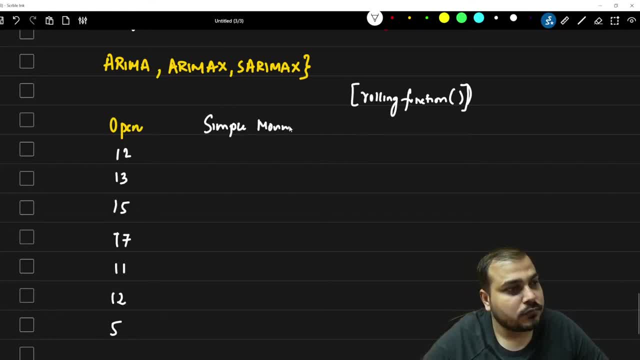 Now, if I talk about simple moving average In simple moving average, let's say that my rolling window, my window size, is 10.. Okay, Now, this basically means that what I'm actually going to do, Suppose my window size is 5.. Let me just 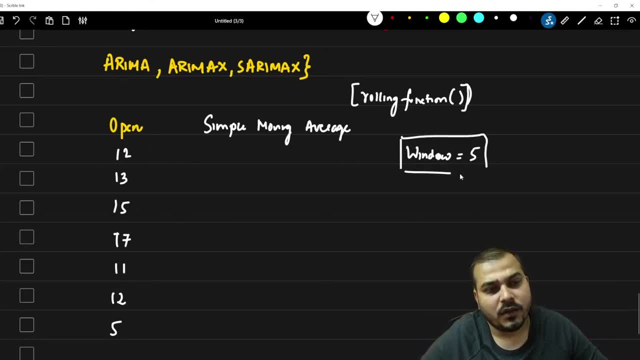 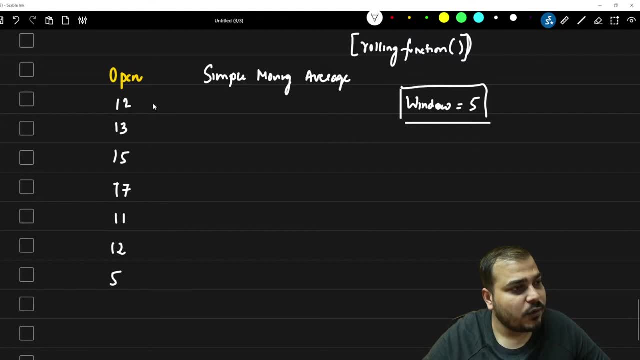 say that, okay, it is 5.. Window size is 5.. Now, with respect to window size is 5, and with the help of simple moving average, What we are actually going to do is that we are going to take this initial 5 data. So this is my. 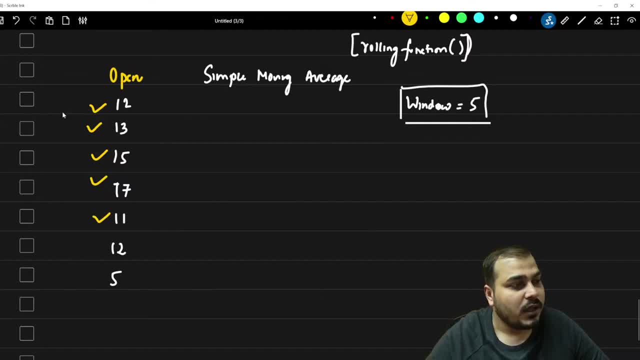 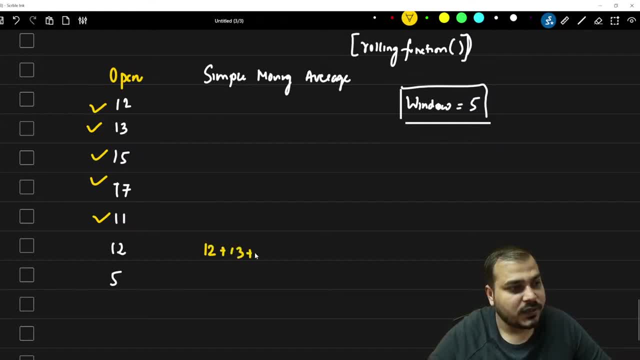 by 5.. So if I probably say it will be 12 plus 13 plus 15 plus 17 plus 11 plus 12.. This entirely will be divided by 5.. Now just tell me what is the answer with respect to this, Because here I have. 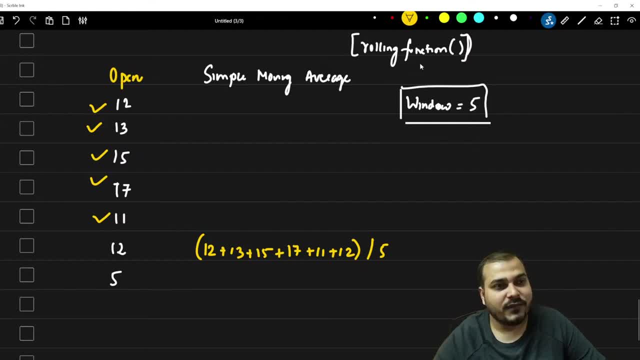 set the window size as 5.. That is the reason. whenever we use rolling function here, all the values will be coming as NAN. Okay, NAN, NAN, NAN. So if I probably try to see this Okay And try to find out the output, 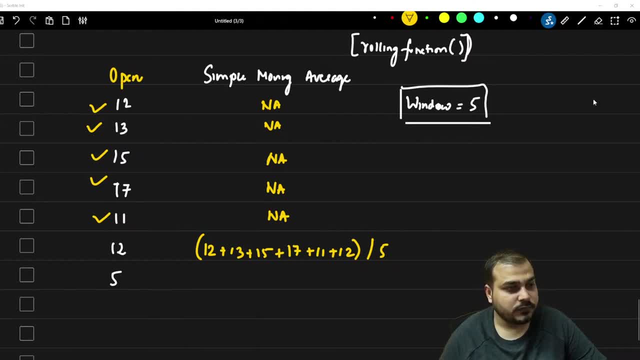 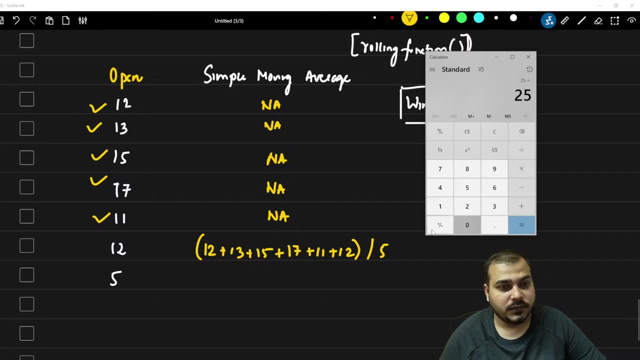 You will be able to see. if I open my calculator, Okay, And if I probably open and calculate, it is 12 plus 13 plus 15 plus 17 plus 11 plus 2.. Okay, And this will be entirely divided by 5.. 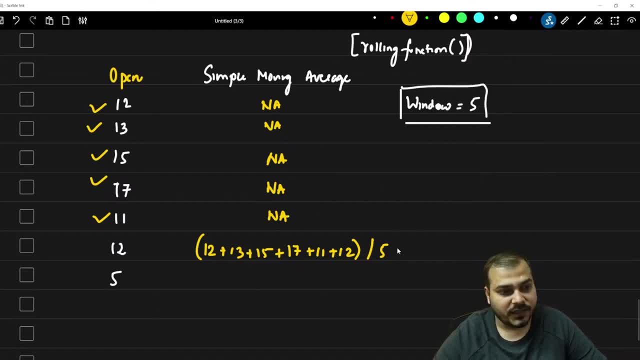 So here you can see 16.. So here, obviously, my answer will be 16.. Okay, Now what will happen next? In order to calculate the roll simple moving average for this line, Then what we are going to do, We are just going to move, Since my window size. 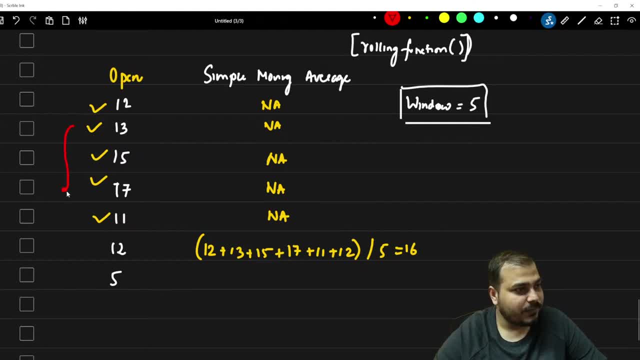 is 5.. The next window size: we are going to just move by one step. That is this, all elements. So it will be 1, 2,, 3,, 4, 5.. Right, So similarly what I will do In order to calculate over here. 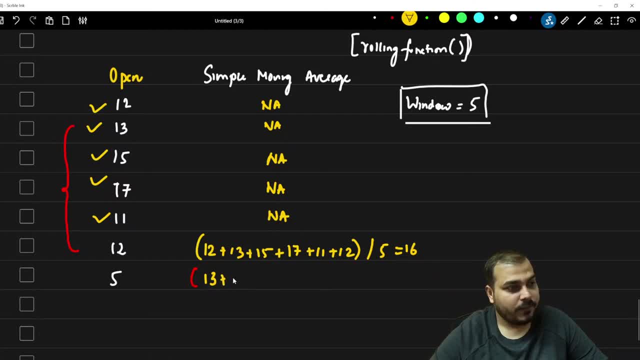 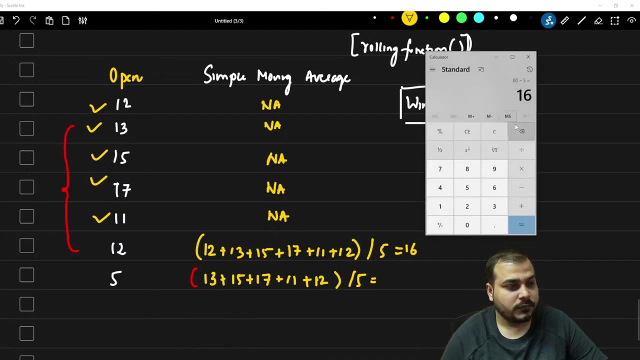 I will just write it as 13 plus 15 plus 17 plus 11 plus 12. Divided by 5. Now if I probably try to calculate it here again, How much it will be So here you can basically see that. 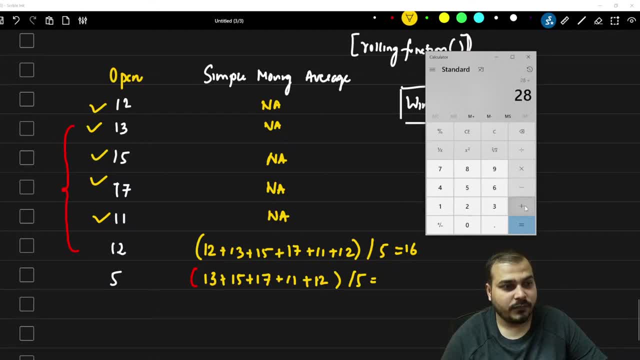 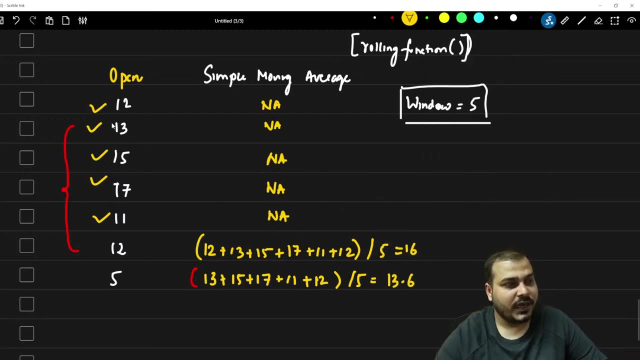 If I probably try to write it down: 13 plus 15 plus 17 plus 11 plus 12 divided by 5.. So here you can see, it is 13.6.. Right, 13.6. So again I am actually. 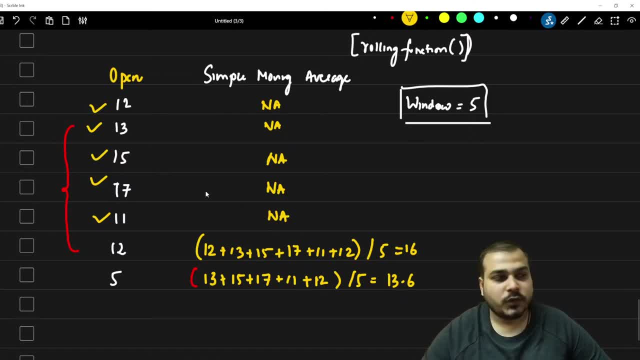 dividing by 5 with respect to this. Okay, Now it will be divided by 5.. See, I am moving one step down, Right, My window size is actually 5.. So when I am actually trying to calculate the simple moving average Considering the 5 elements, 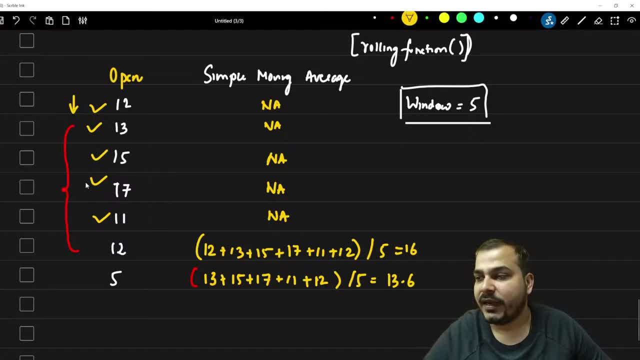 for this row, So it will get shifted one position by that And Okay, And it will probably take this, all things, and it will basically calculate it. Okay, So 1,, 2, 3.. Okay, Just a second: 1,, 2,, 3, 4,. 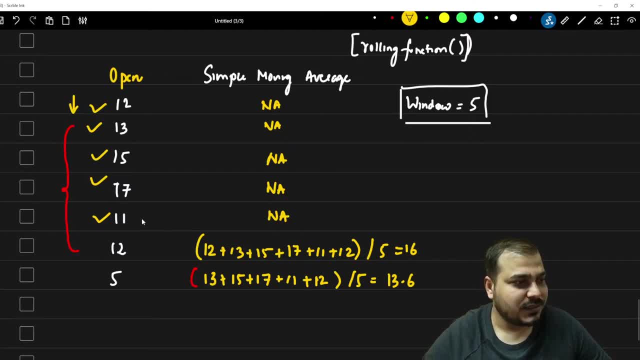 5. Okay, So, if I probably So, this element will belong to this row. This element will belong to this row. Okay, So in this way, you will be able to find it. This is the mapping that will be done. This will be the. 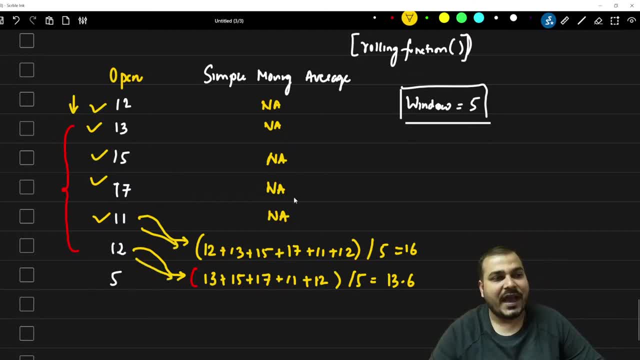 mapping. that will be done, Because before this 11 you don't have any simple moving average over here. Okay, So just this mapping. Consider this mapping, Okay, And probably you will be able to see this over here that I am basically taking this. 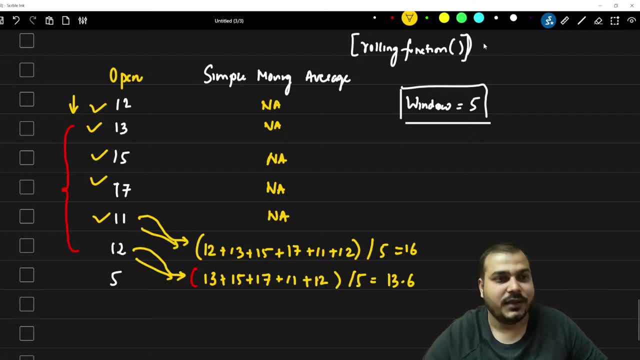 first 5 sum and probably pointing it over here instead of writing the row down: Okay. So again, if you want to consider, this entire thing is just getting shifted by one thing. Okay So, this is perfect and this will get dropped. Okay, This will basically get dropped. 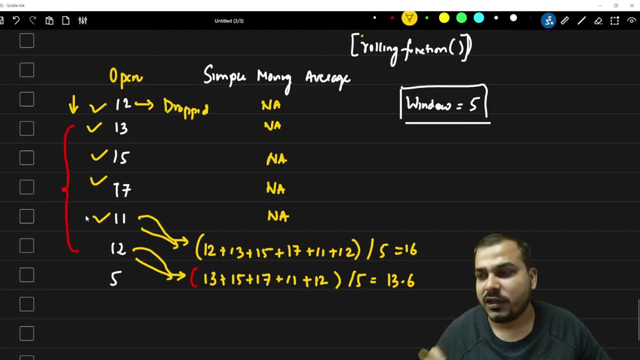 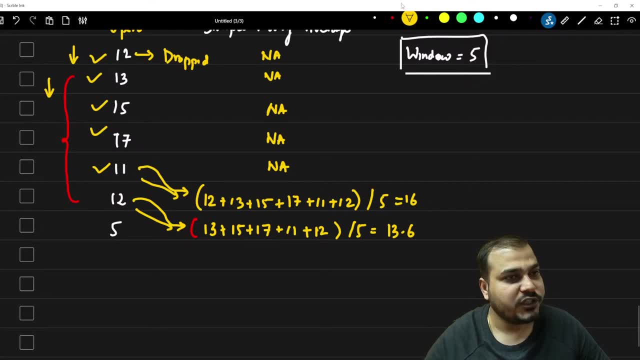 and here we are just going to go towards one position, And this is what simple moving average is all about. Okay, And similarly, you will just go and keep on doing it. Then the next element: again, you will move one position down and the next. 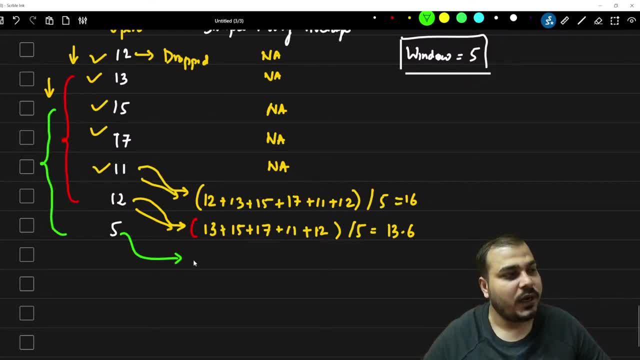 position will be this: 5 elements, which you will probably calculate, and just tell me how much it will be coming: 15 plus 17 plus 11 plus 12 plus 5.. Okay, Divided by 5.. So what will be the output? 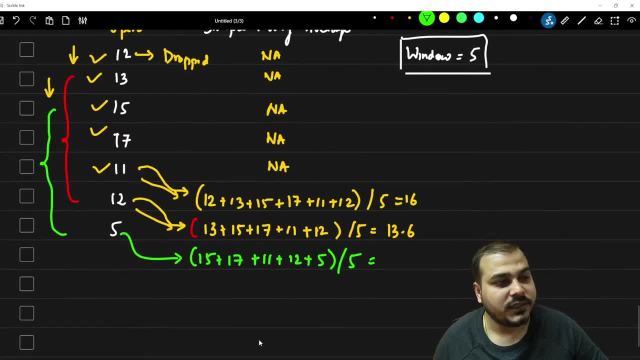 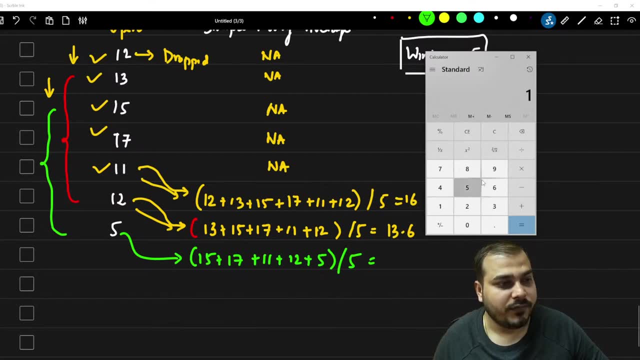 over here. Okay, What will be the output over here? Just tell me So, if I probably try to calculate with respect to the calculator. So it will be 15 plus 17 plus 11 plus 12 plus 5.. Okay, And 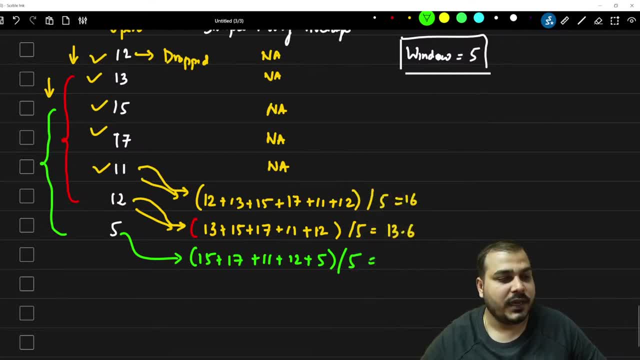 here. if I probably divide by 5, it will be 12.. Okay, So finally I am actually going to get 12 as my output. So like this, we can calculate the entire simple moving average. It is very simple, Based on the window size we are just trying to calculate. 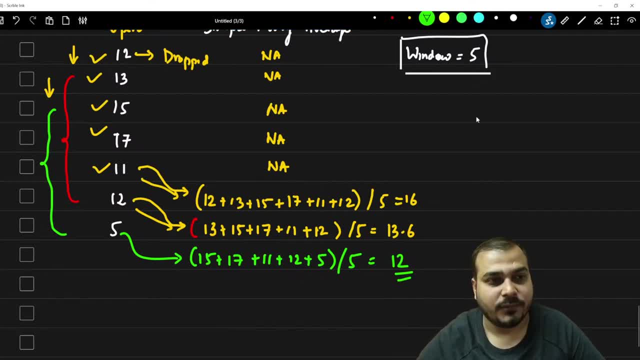 it and we are trying to plot that specific diagram. So suppose if my graph is something like this, Suppose my graph looks something like this, where it is having lot of zigzag, and probably like this: If you are trying to apply simple moving average, you will be able to see that we will be getting a. 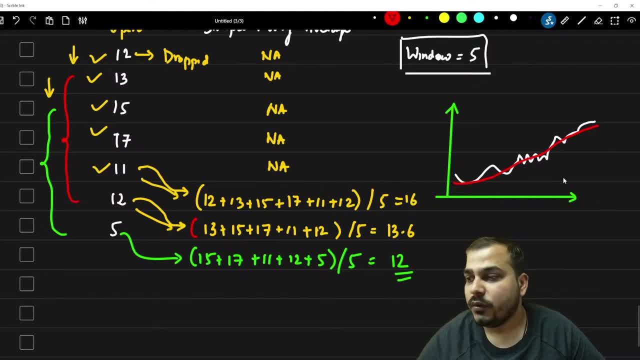 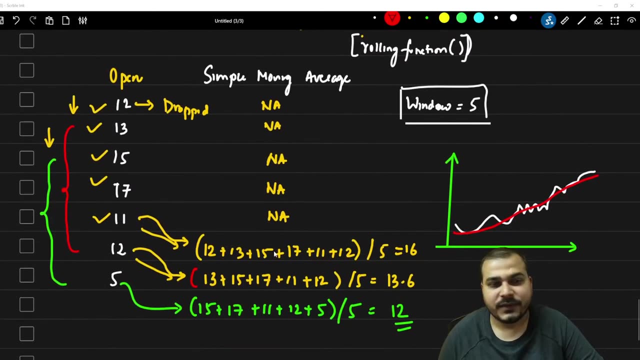 smooth graph which will actually help you to. uh. Okay, I am going to hide you because I think you should not join the session, okay, Okay, So this is clear everybody. Can I get quickly? Yes, I hope everybody is clear. So, in short, you are actually. 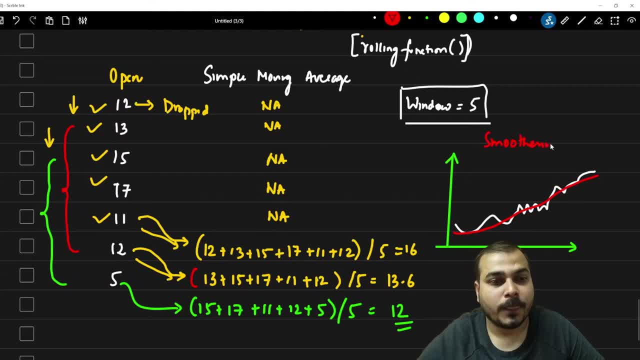 smoothening the curve. In short, you are actually smoothening the curve. Yeah, Yes, Simple, moving average. Yes, Absolutely right. Yesterday, whatever code we had actually written First equation- please look at it. Which first equation? 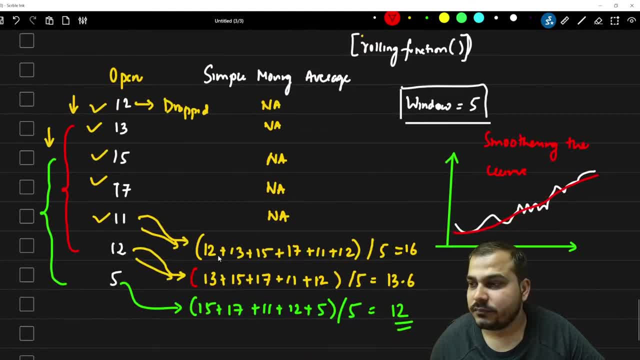 I have not written any equation over here, Okay, Sorry, So this will be plus 11.. Now, this is fine, Right? No, Does it called as moving average? No, It is called as simple moving average. Okay, So this entire. 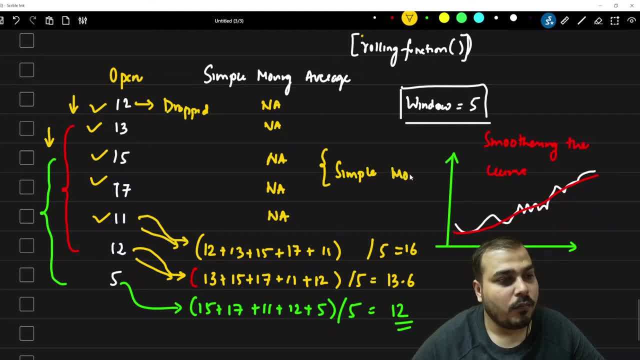 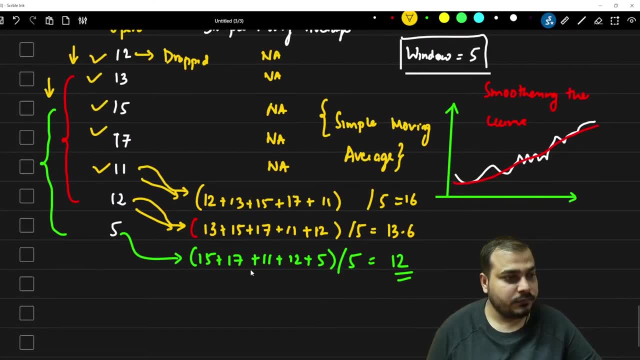 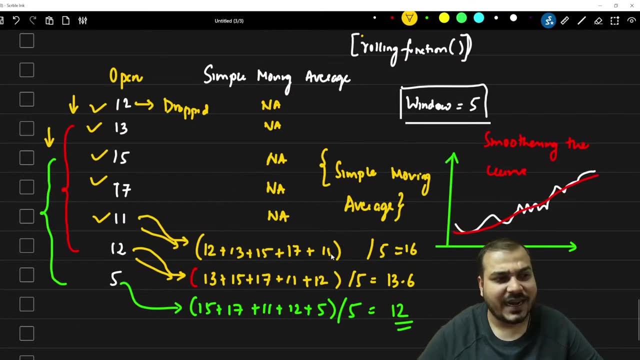 thing is actually called as simple moving average. Okay, Moving average is completely different. We will talk about it. Okay, So here you have 5 elements, and then here you have next 5 elements. So probably what you are doing over here. I just added one. 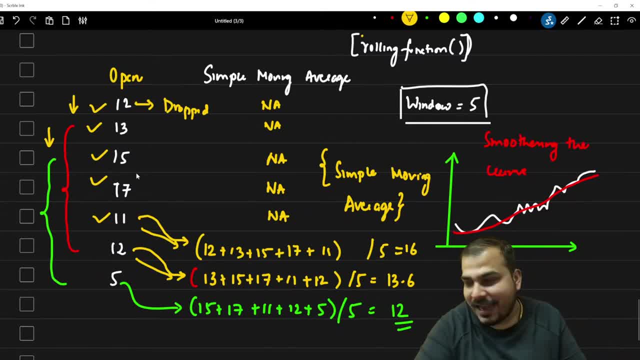 more element. but understand the concept, guys. Calculation is not that important. Okay, Calculation is not that important because with the help of code, you will obviously get perfect solution. Okay, Fine, 12 was not there. You can, I can say that. okay, change the window size. 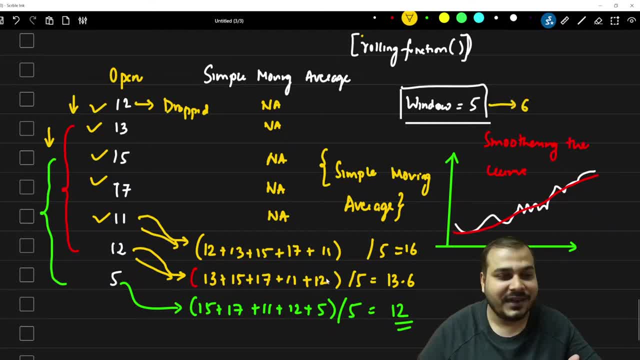 from 5 to 6, then probably you will add 12.. You will try add the next element. Okay, But it is okay. Try to understand what I am trying to teach you. Do not focus more on the calculation. This is a live session. 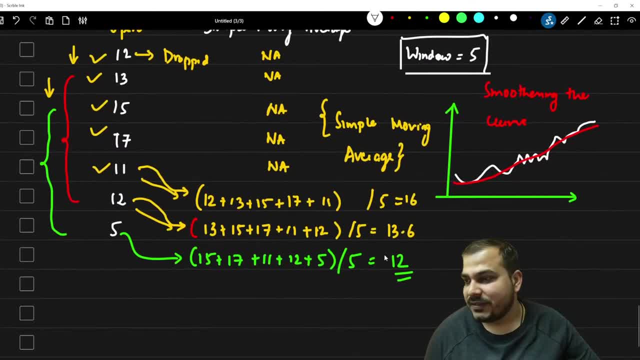 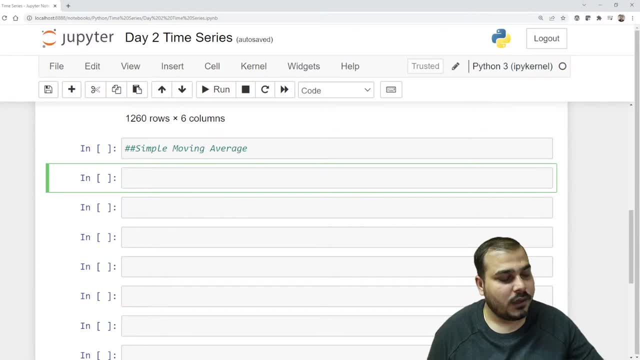 So it is okay, We can go ahead, Okay. So I hope everybody has got that Okay And you are able to clear this. Now let us go ahead and do it with the help of coding, Okay. So what I am actually going to say, 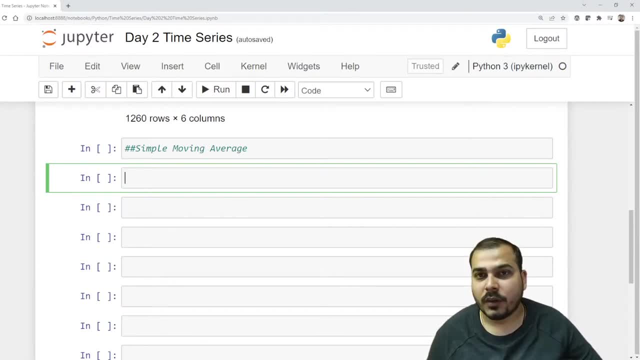 over here is that I will just try to. Okay, Why simple moving average? It is basically just to do some kind of smoothening of the graph. Okay, Whatever graphs you have Now suppose, if I say df of open dot plot. 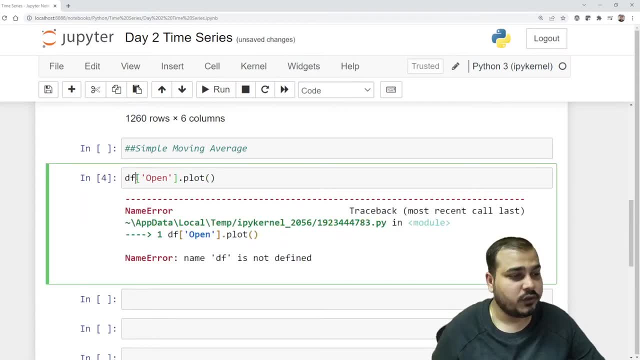 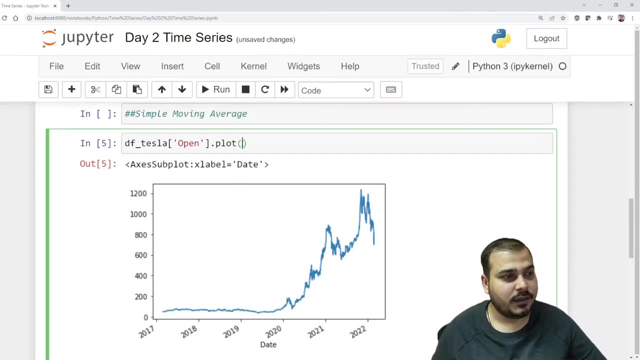 If I try to just create this plot. Sorry, df underscore tesla. Now here you can see that obviously this plot looks quite lot of zigzag movements are there Probably. I want to put with some kind of figure size. Let us say I am putting figure size as. 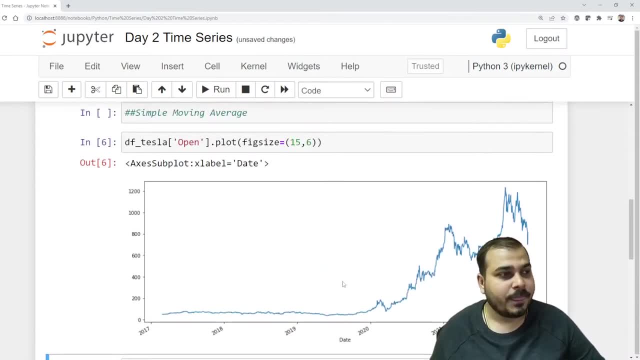 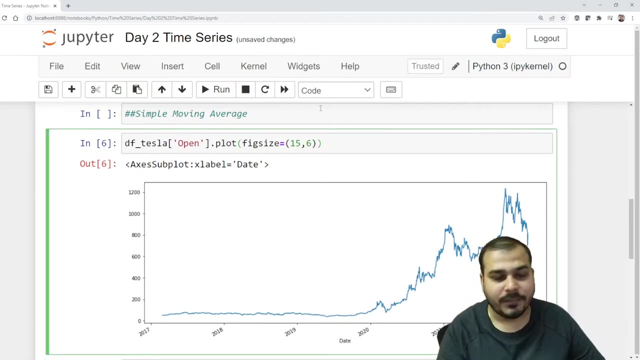 15 from a 6.. Now, here you can see this entire graph. Okay, Now what I am going to do is that I am just going to create a simple moving average of this specific graph. You can also provide your x limit, y limit, That is fine. 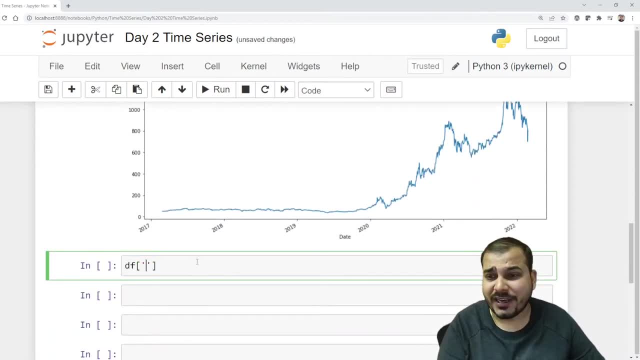 But in order to create a simple moving average, what I am actually going to do, I am just going to create a column. Say that for open. this will be my 10 windows 10 days rolling. Okay, So this will be my 10 days rolling, and here. 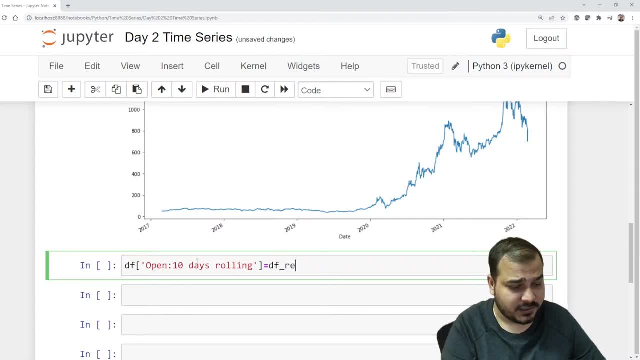 I am going to just say that df underscore tesla. So here also I am going to write df underscore tesla. And here I am going to just take my open column, dot rolling, and here I am just going to specify: See, in rolling you have something called as window. 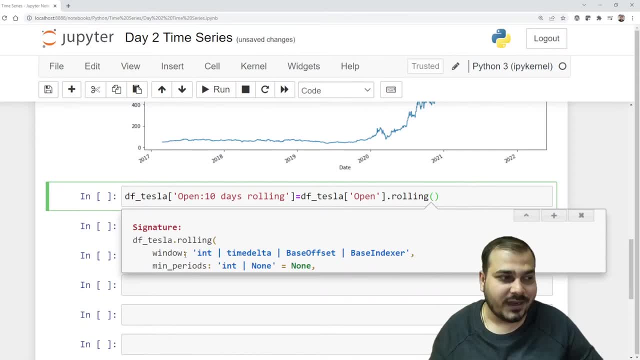 Like whether you want 10 windows, whether you want 20 windows, what should be your window size? And in window there is also one specific thing. Okay, If I probably consider this. Okay, What we can also do is that I will just try to write it down in front of you. Okay. 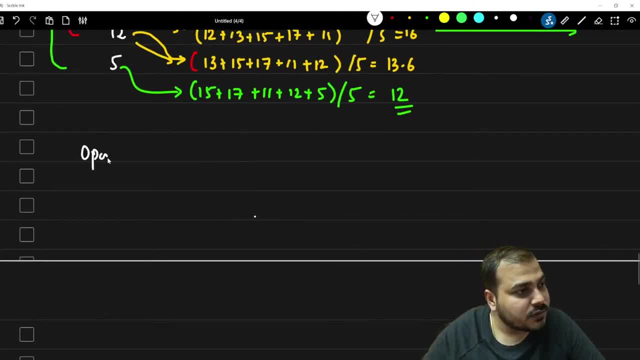 Suppose this is my open column. Okay, Suppose this is my open column. If I probably say okay, find my window size is 10.. Okay, So, which is obviously given over here You can see the first parameter in the rolling. So here I can say that window size. 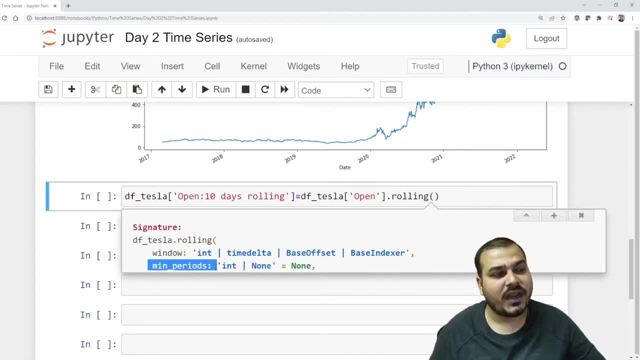 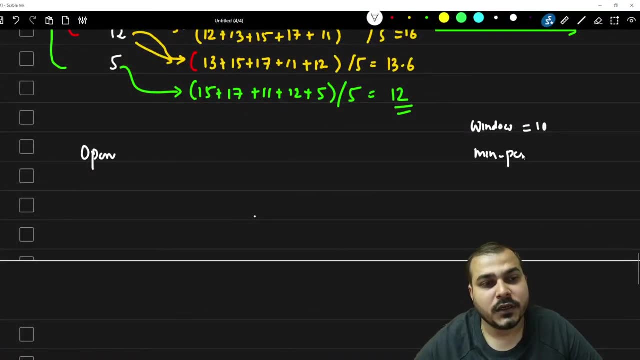 is some specific size. And there is also one more parameter, which is called as periods. Okay, Now, with respect to this particular period, if I say my minimum period is equal to 1.. Okay, So what will happen is that- suppose I say I have some values? 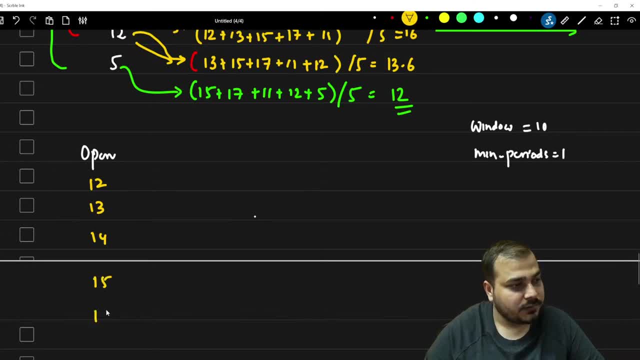 like this: 12, 13,, 14,, 15,, 16,, 11.. Okay, If I say my window size is, let's say 5.. Okay, Let's say my window size is 5.. So, and with respect to this minimum period, Now see, 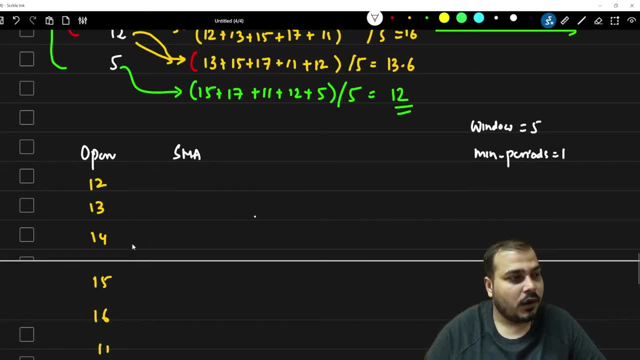 if I am trying to calculate this simple moving average. Okay, Obviously, you will be able to see that for calculating the first 5.. Obviously, to calculate the first 5.. I will obviously get the answer over here. Okay, But this all values will. 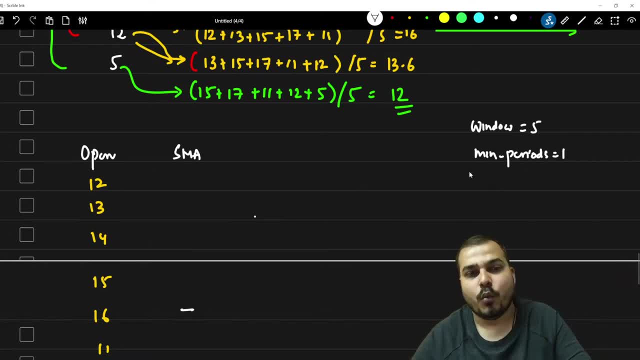 never be NAN. Okay, Because we are just going to keep one value as NAN over here And remaining all values will be the same values. Okay, That is what this specific thing says. If I say minimum period is equal to 5. Then it will probably put. 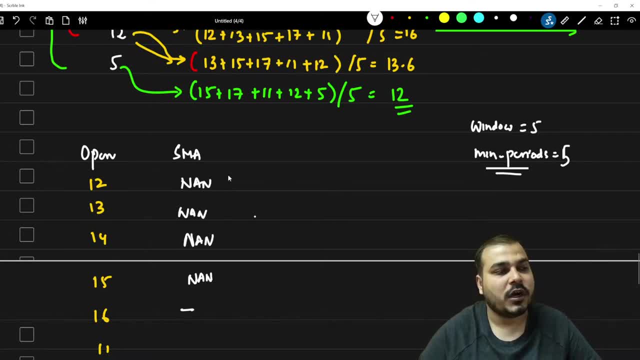 all the starting values as 5 NAN. Okay, So this is what it is basically done, Doing it with the help of minimum periods. Okay, Since I don't want to put NAN, Because if I don't put NAN, If I just say that my minimum. 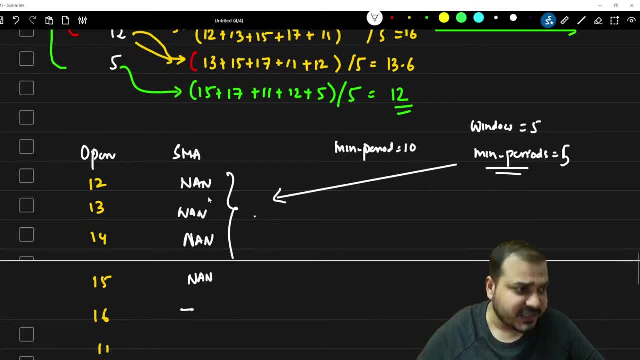 periods is 10.. That basically means my starting 10 value will all become NAN. Okay, I don't want to do that because I want to make sure that the line starts from the starting, Because if there is NAN, then the line will not probably start from. 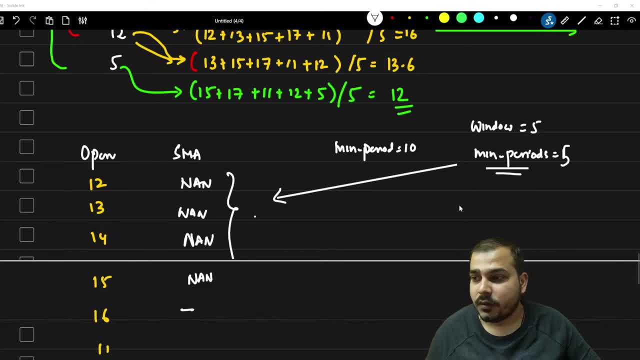 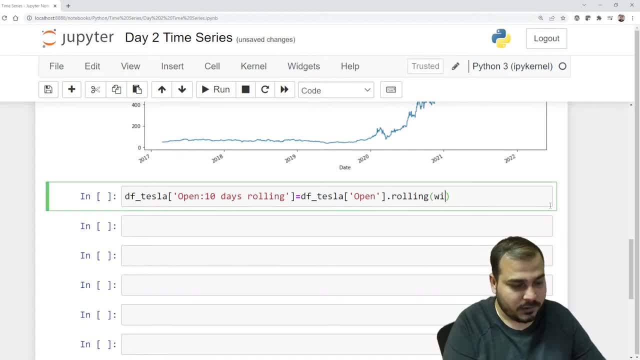 that point of time. Okay, So that is what I am actually planning to do. Okay, So let's go ahead and let's try to do this. So here I am actually going to say my window size will be probably 10. Because I am. 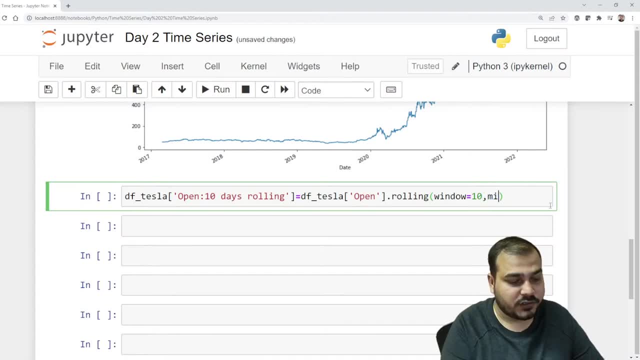 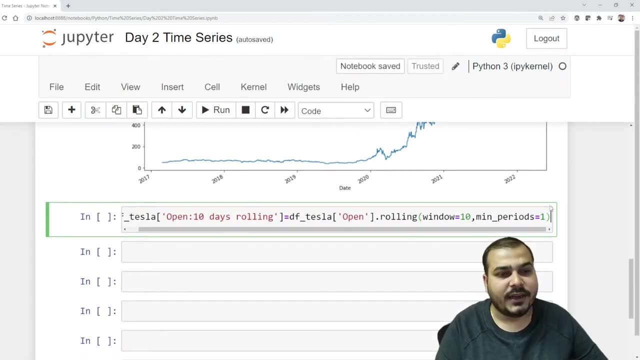 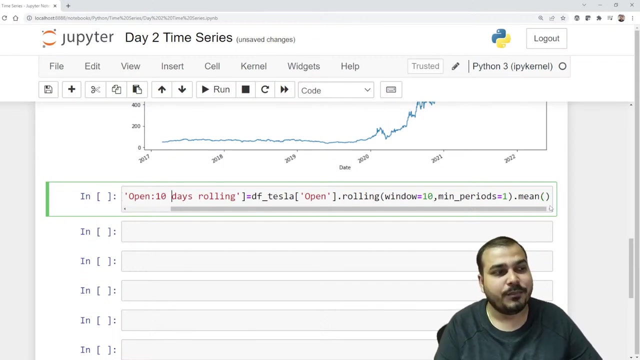 making 10.. And then I will also say: my minimum periods is equal to, let's say, 1.. Okay, So if I try to execute this And after this I have to use an aggregative function to find out the mean value, Okay, Because we are doing a simple. 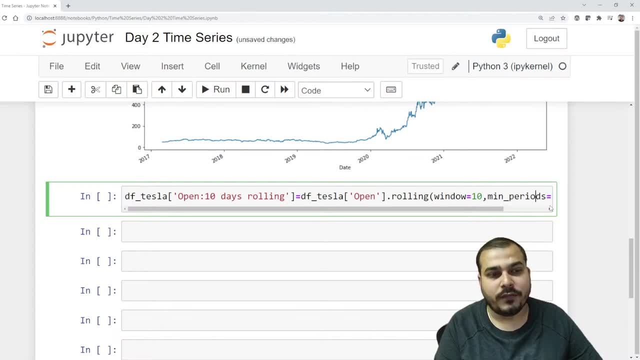 moving average. Okay, So here you can basically see dot rolling of window 10 and minimum periods is equal to 1 dot mean. So if I execute this, you will be able to see my df of open 10- sorry, df underscore- tesla- open. or let me just 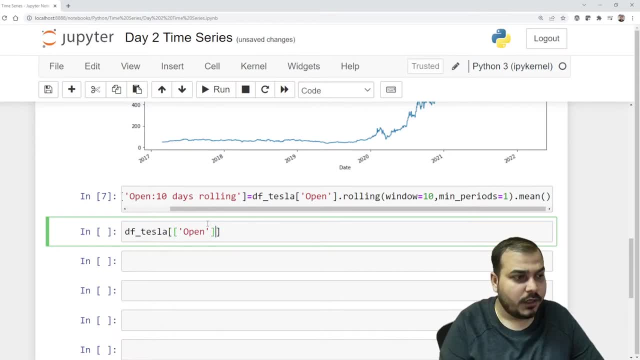 directly plot it Okay. So here I am actually going to plot two important features. One is open and the other one is open 10 days rolling. I am just going to copy this And paste it over here. It's not about deciding the window size, guys. Still. 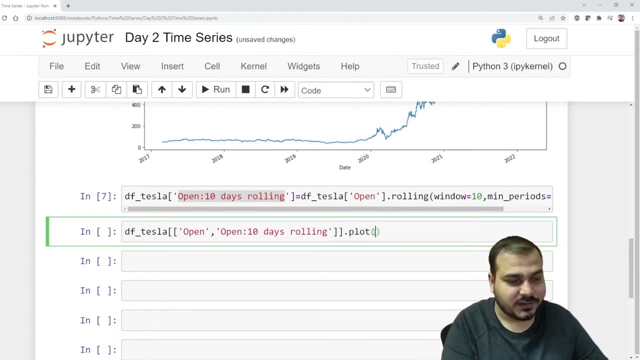 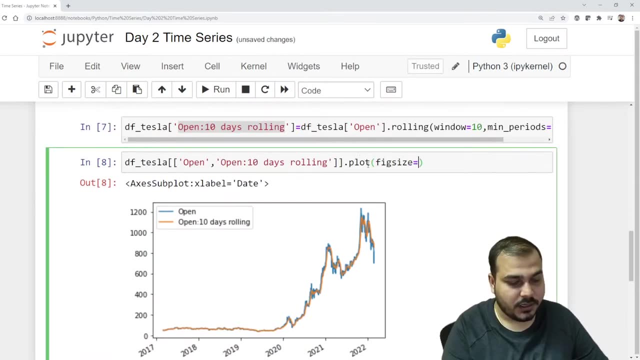 we are in the analyzing state. Okay, You don't have to decide anything over here. So if I try to plot it Now, here you will be able to see. let me make my figure size little bit bigger, And here I am actually going to specify. 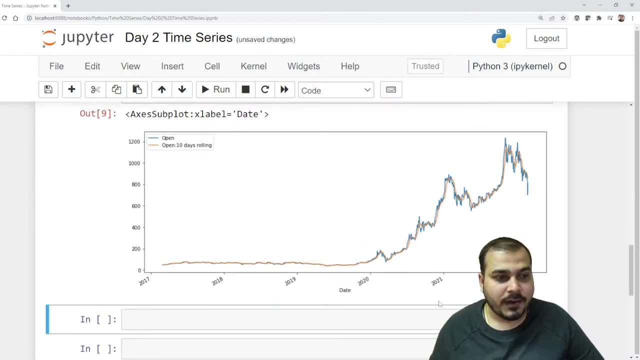 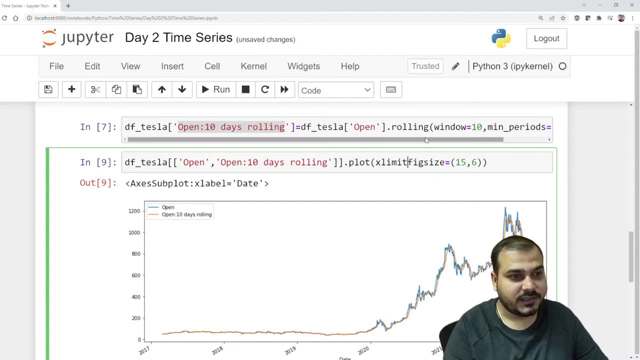 15, comma 6.. So my figure looks quite good. Now, with respect to the orange line, I know you are not able to see the line properly, So I am actually going to keep some x limit, So let's say my x limit. 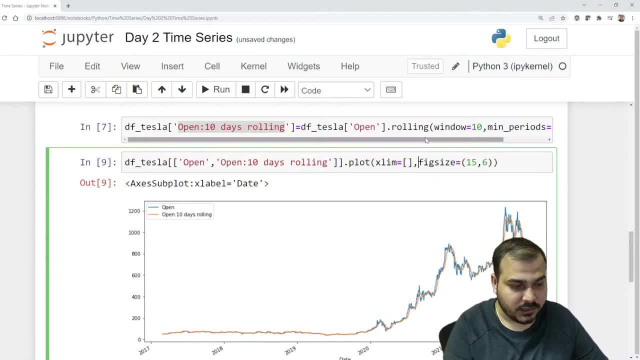 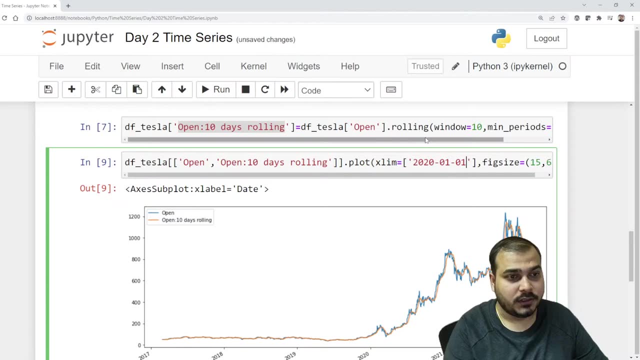 is equal to- and again, I can give this in the form of list- It will probably start from, let's say, from 2020 01 01 till 2021 01 01.. So I am just focusing on probably the first year data from 2020. 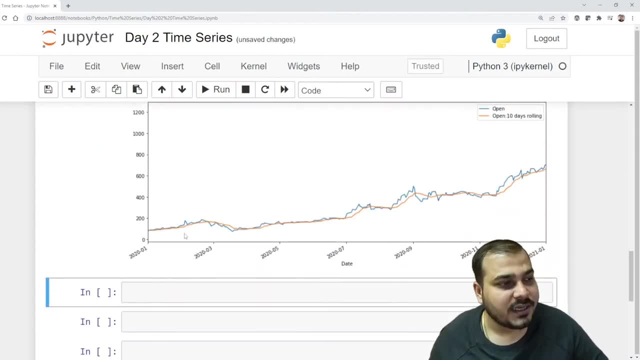 to 2021.. Okay, So if I execute it Now, here you can see, based on this graph, we are able to get this simple moving average. Now why specifically this is getting used, Why people are using this. If I probably open this image in new. 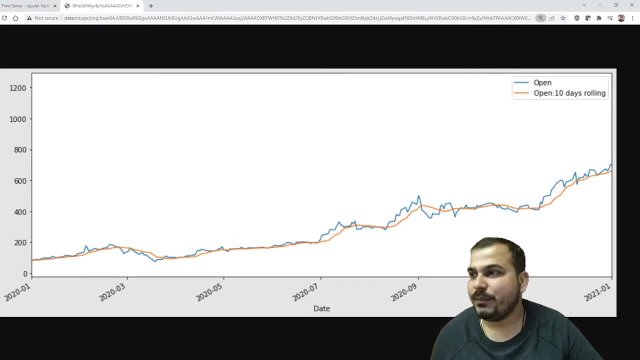 tab, If I zoom in right, Why specifically people are actually using this. I will also show you that, So let me open my epic pen. Okay, Now in financing, right In financing. why do they probably use specifically in stock markets, Right In stock markets? 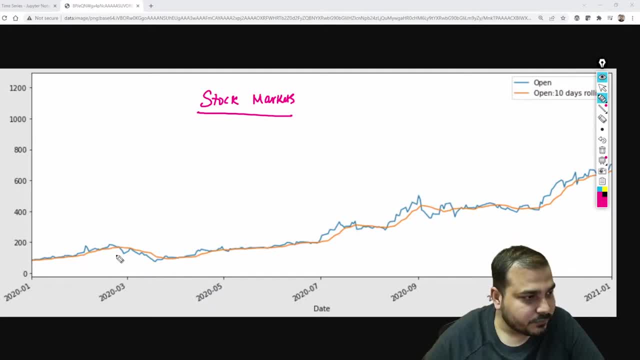 Right, You will be able to see that at one point of time, when this specific line crosses, Okay, Or probably when the line actually touches and when this line is below this, you know. So this can be a buy situation for the people. This. 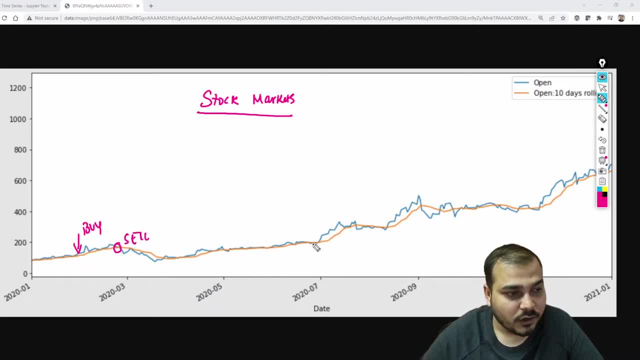 can be actually sell situation for the people You know. Over here also, you can see that after the line is basically touching, it is then going up. So this can also be an indication to probably say that, okay, this is a buy time for you. Over here you can. 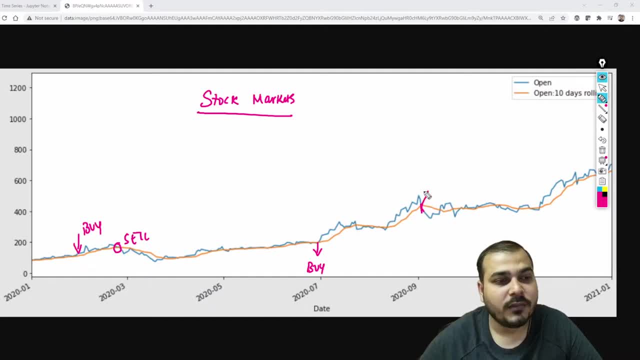 specifically see that when this line crosses, it is probably the time to actually sell your stocks. Okay, So this smoothening, This smoothening method, right With the help of simple moving average for a short term, For the short term, is also extensively 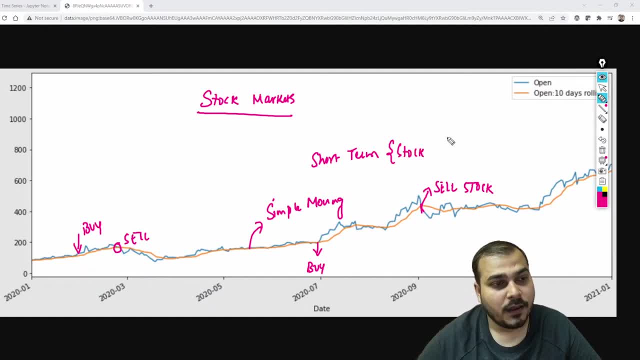 used in stock markets. Okay, Now what you should basically do. You should just not depend on this 10- 10 rolling window. Instead, you can create any number of rolling windows: 10,, 20,, 30,, 40, 50. 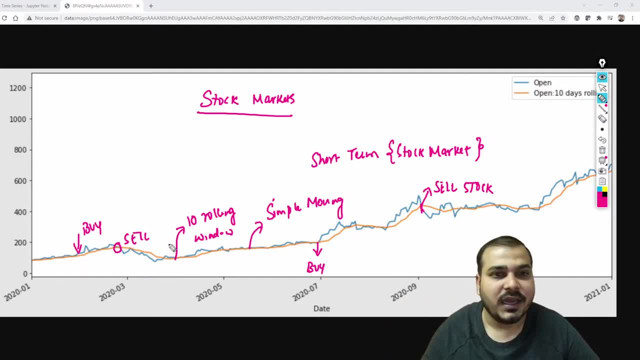 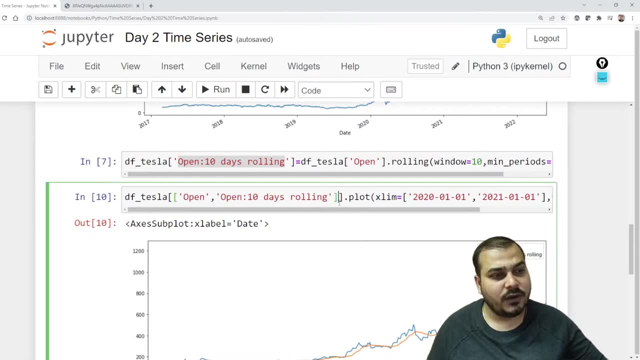 and try to probably create that specific graph and try to see that how this specific thing is actually working. Okay, So I hope you are actually able to understand what I am actually trying to say. So, similarly, what I will do is that I will create. 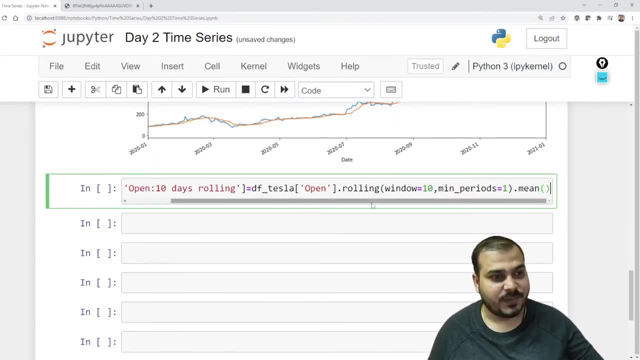 lot of different, different rollings. So here I am going to basically specify this. This time my rolling will be 30. Let's say I am going to do it for 30. So here you will be able to see 30. And similarly. 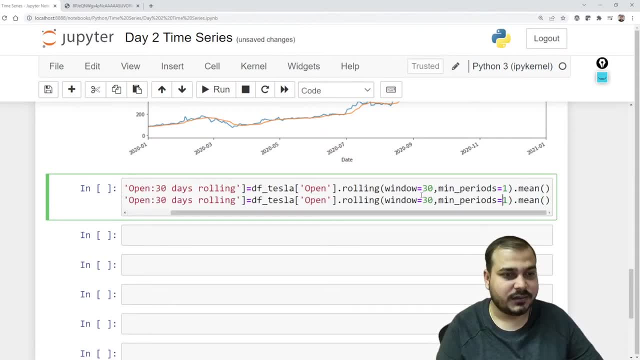 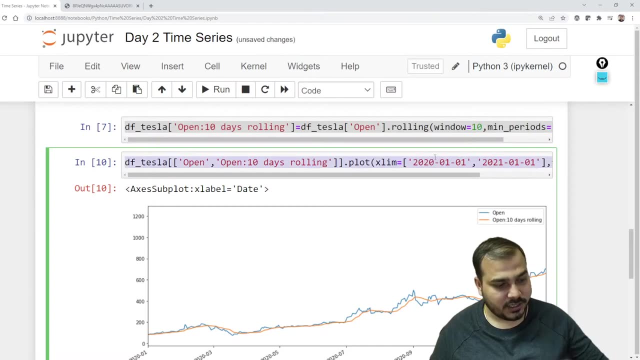 what I can do is that I can also make it for 50.. Let's make it for 50.. And different, different rolling part I can actually make, And then I can also make sure that I plot all those things and then try to compare. 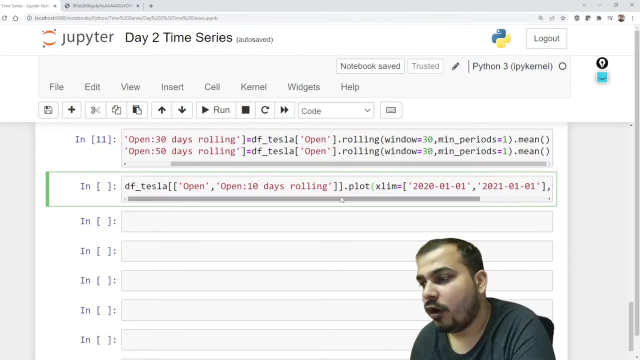 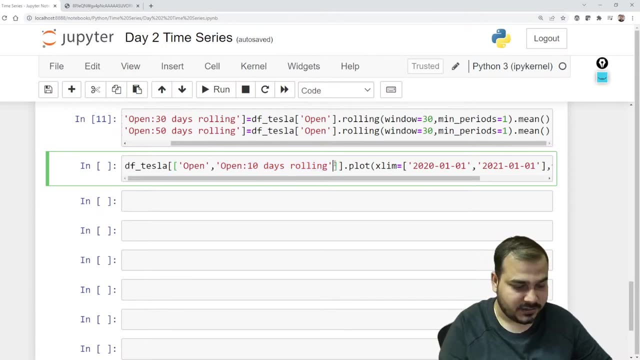 Okay, Try to compare. So I am going to basically plot it for: open 10 days, Open 20 days, Okay, Open 20 days. Open 30 days, Like this: Open 20 days, Right, And similarly I can do it for open. 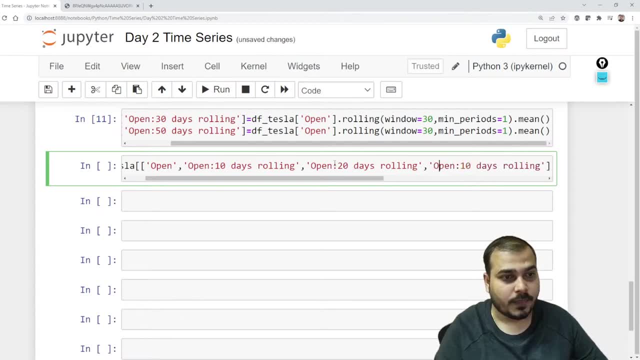 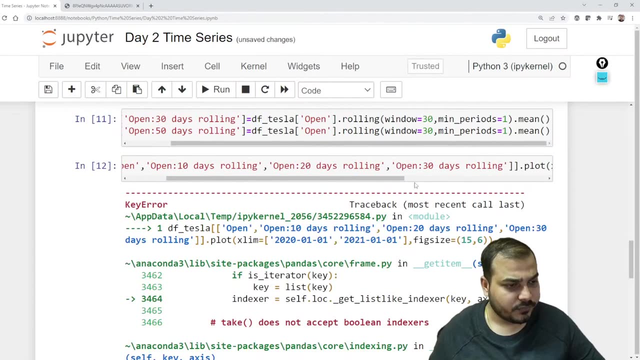 30 days: Open 30 days. Right, I can actually do all this thing for different different days and just try to plot it. Now, see I am getting an error. 20 days rolling is not there. Okay, 20 is not. 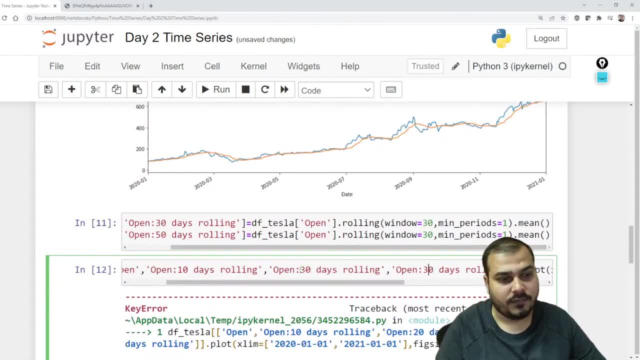 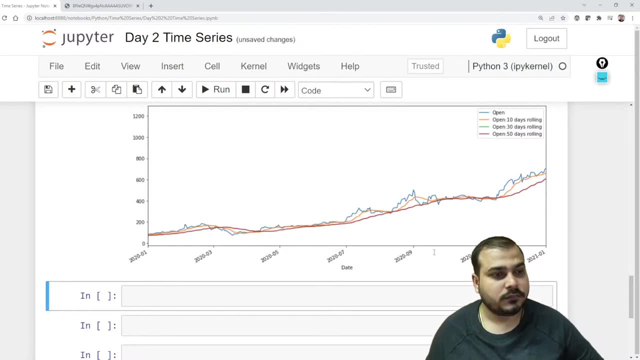 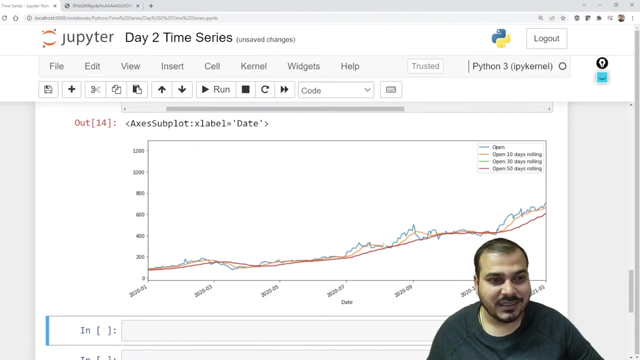 there 30 and 50. are there Right, 30 and 50. So if I execute, sorry, not 40, it's 50.. Okay, Now here you can see that how this graph looks like The open 10 days actually, when it is providing the smoothening. 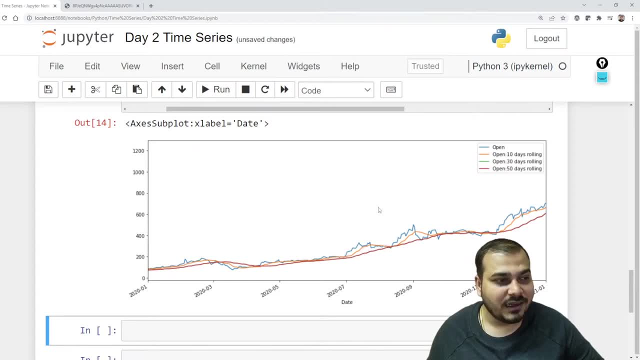 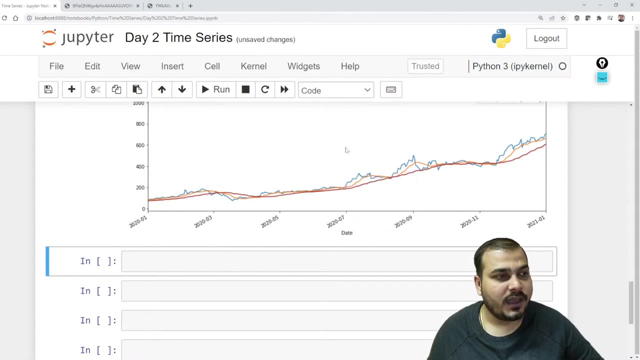 you can see there is a difference Right With respect to the green color: open 30 days rolling and 50 days rolling. you can also see something Over here. lets me open the image in new tab so that we can zoom in The green. I don't. 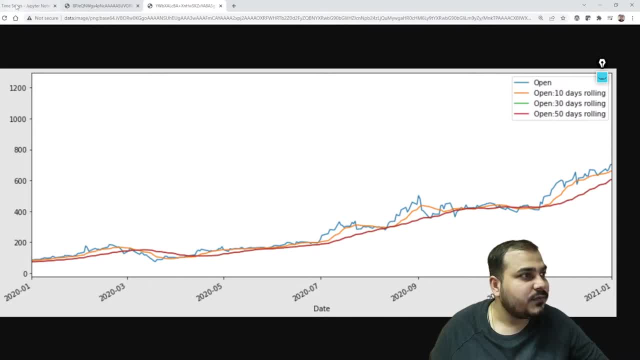 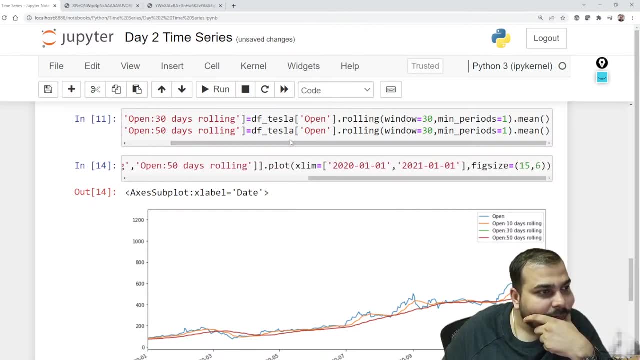 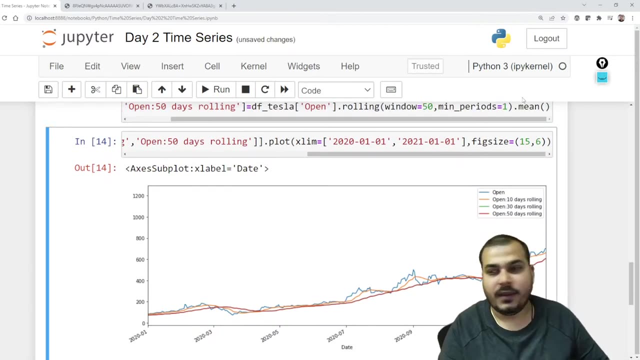 see the green one. Why Specific reason for the green one? I don't see it. Open 10 days, 30 days, 50 days, dot plot: 30 days. Okay, Both are same, So here I am going to just make it for 50.. 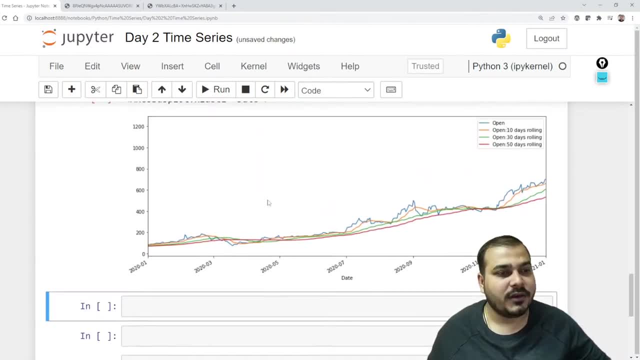 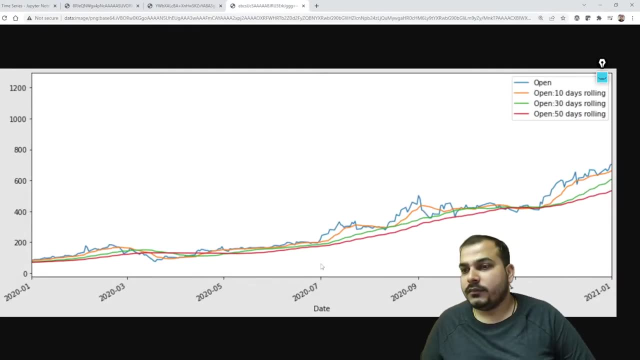 I did not change it to 50. So now you will be able to see that I am able to see this in the image tab in an amazing way, Right, So I hope you are able to understand this. Till here, everybody is clear. No, red was not. 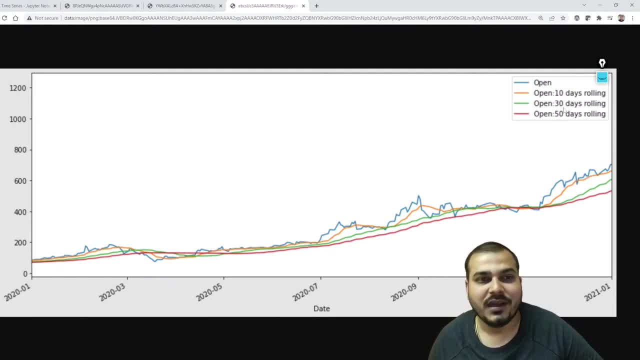 overlapping the green because I had for 50. also, I had kept the rolling sizes 30.. Okay, Everybody clear? Yeah, So this is how powerful a simple moving average is, and you can definitely do anything with respect to the smoothing. But see, initially my graph was lot of zig zag. 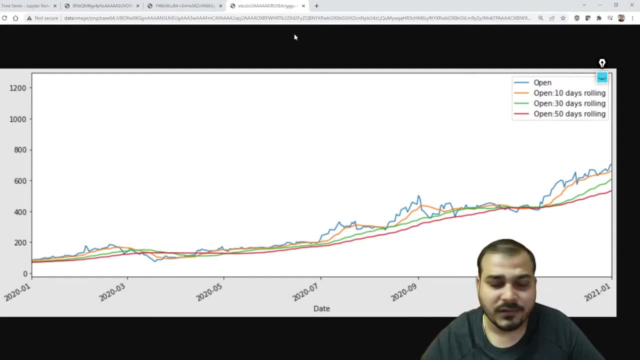 now I am actually smoothing it and I am doing it. Now there is some disadvantages with respect to the simple moving average. Okay, Lot of disadvantages. Now what is the major disadvantage with respect to simple moving average? See, I am just going to talk about 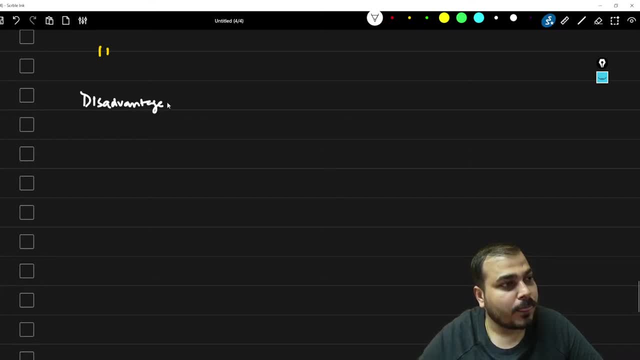 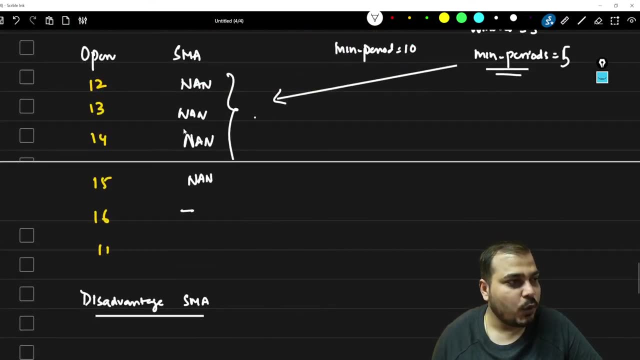 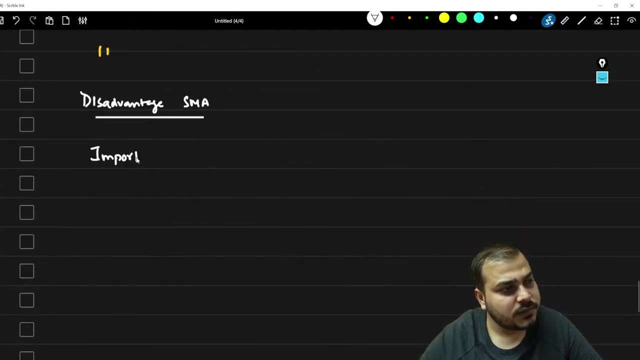 disadvantage of simple moving average. Disadvantage of simple moving average. Now see, one thing is that whenever you are probably trying to add up or trying to find a simple moving average, you are giving importance to all the data. You are giving importance, and what kind of importance? Similar importance. 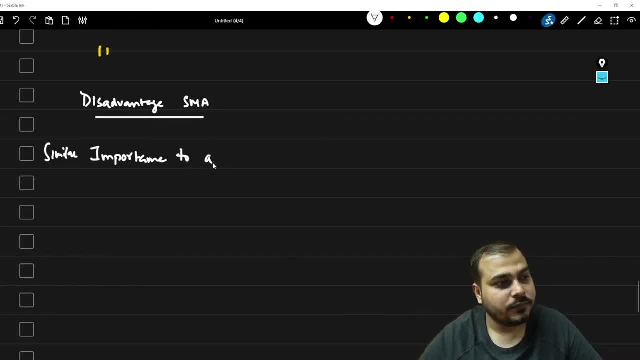 Similar importance to all the data, because when you are calculating the average, you are just doing x1 plus x2 plus x3 plus, like this, till xn divided by n. You are always doing in this way itself. Right, It is always. you are actually trying to. 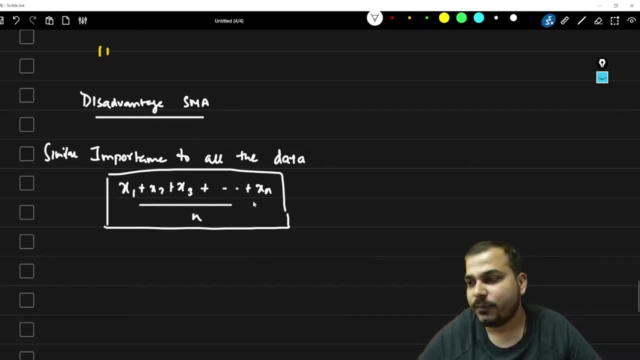 always provide this specific formula to all the data points based on the window size. Okay, Where n probably may be your window size, Right, You are doing this Right. So what is the problem with respect to this? Because see in time series data. 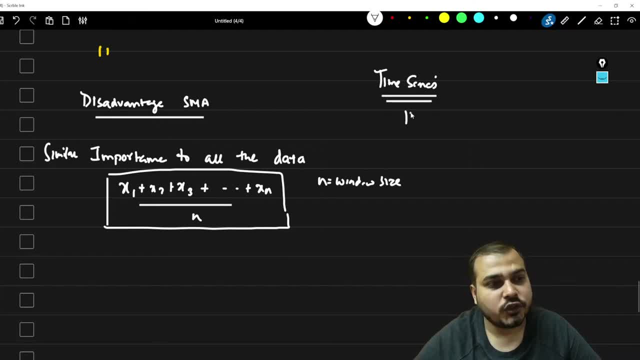 our main focus should be given to the recent data. a lot Right And based on that, we should definitely do the predictions. Okay, Please don't this to Rabindra Guys. this need not be used in stock markets. and all Again, understand, I am teaching. 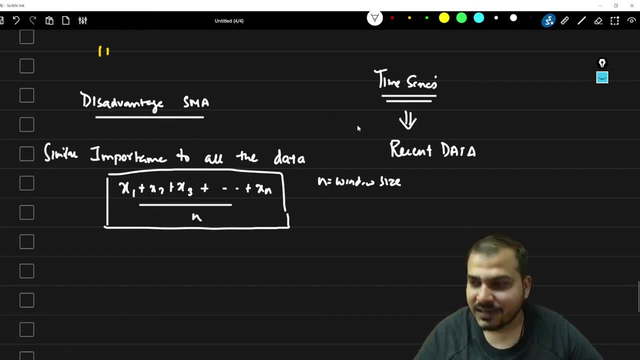 this for a purpose, so that you can clear the interviews and do something. Okay, Please don't do that. Okay, Don't go and invest your money. Please note: you will not become a millionaire by stock. You will not become a millionaire. I have greatly 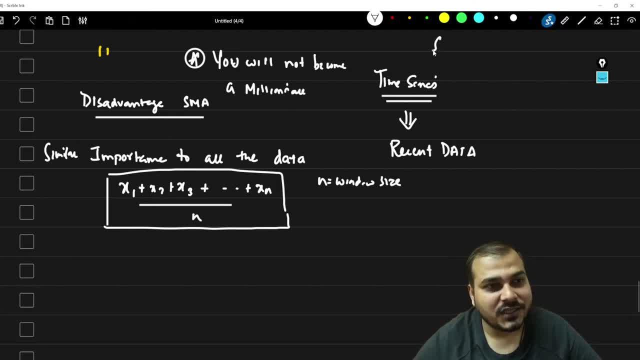 written from all these things. This is just for educational purpose. Educational purpose- Okay, I know everybody wants money without, without doing any kind of hard work, Okay, So with respect to this, you know, what I really want is that I want to give more importance. 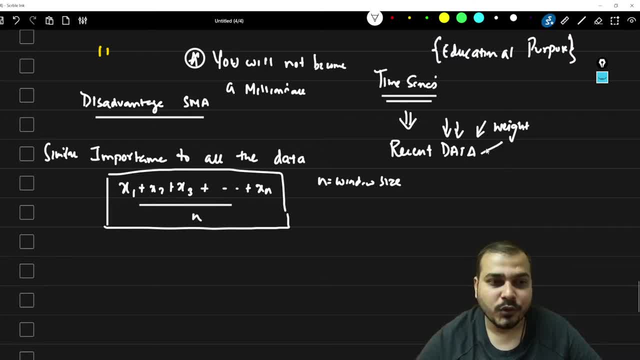 or I can definitely say more weight, more weight to the recent data. Okay, More weight to the recent data. and that weight is basically provided by some parameters which we are probably going to see in something called as EWMA. Okay, Exponential Weighted. 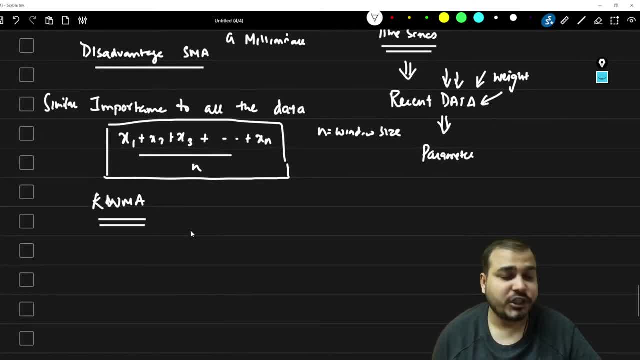 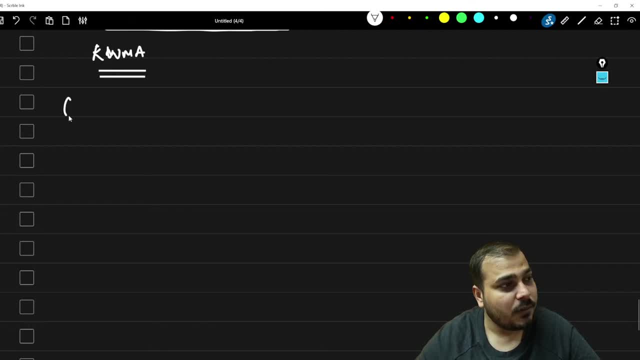 Mean Average. Okay, Sorry, Moving Average- Exponential Weighted Moving Average- We are going to see over there, But before that, let's go and focus on something called as Cumulative Moving Average, Because we really need to cover all these things, and this will. 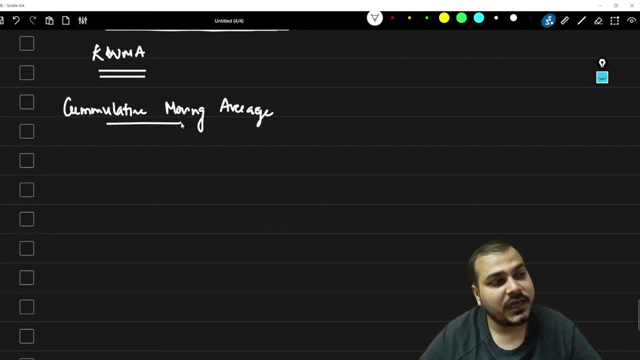 actually help to. this will actually help us to become a perfect thing in when we are discussing EWMA model. So we require all these things, guys. So let's go and discuss about the Cumulative Moving Average. The Cumulative Moving Average is pretty much simple. 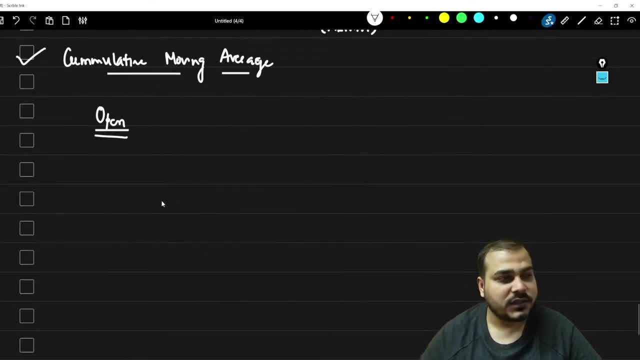 So suppose, if this is my open column, Okay, Suppose this is my open column and I have probably values like 12,, 13,, 11,, 15,, 16,, 10, like this, Right In Cumulative Moving Average that is. 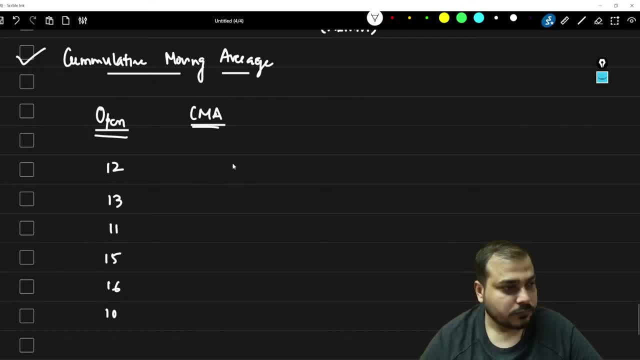 CMA, what we are specifically going to do. Okay, What we are actually going to do, Suppose, if I want to find out till here what is the Cumulative Moving Average. So what I will do, I will just try to calculate the average of this, Okay. 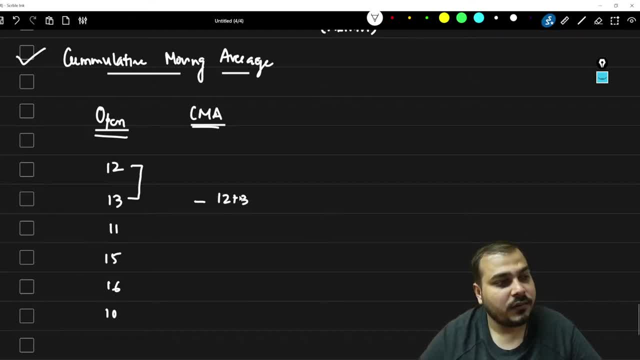 So both of this average, what is 12 plus 13, divided by 2. What it is? So it is somewhere around 12.5.. Right Then, with respect to this specific data, what I am actually going to do, I am going to basically: 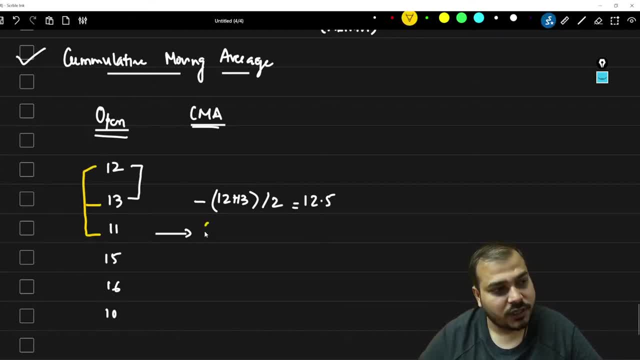 find out the average of this 3.. Okay, This 3. So it will be 12 plus 13 plus 11 divided by 3.. So what it will be So if I try to calculate with the help of calculator, So here you will be able to see. 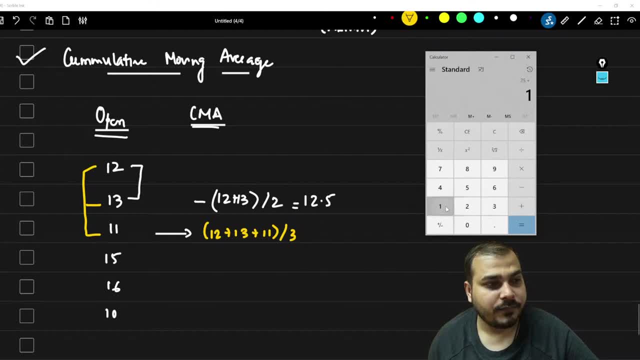 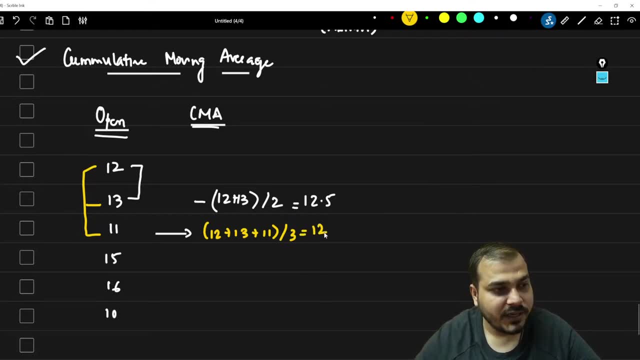 12 plus 13 plus 11 divided by 3.. So here I am actually going to get 12. Right. So this is specifically 12. Right. Similarly, the next Moving Average, that is Cumulative Moving Average, What I am actually going to do, 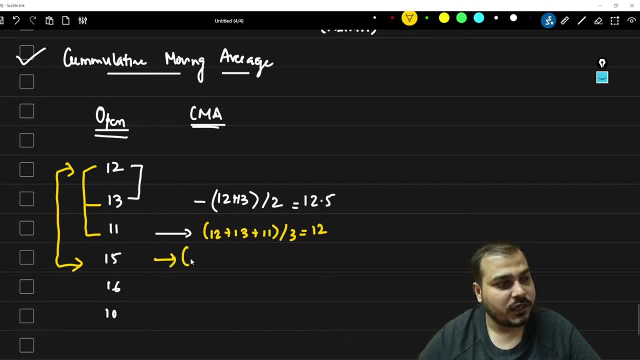 This all, 4. Sum and Average. I have to actually do So. here you will be able to see 12 plus 13 plus 11 plus 15 divided by 4.. So here you will be able to again go and calculate it with the. 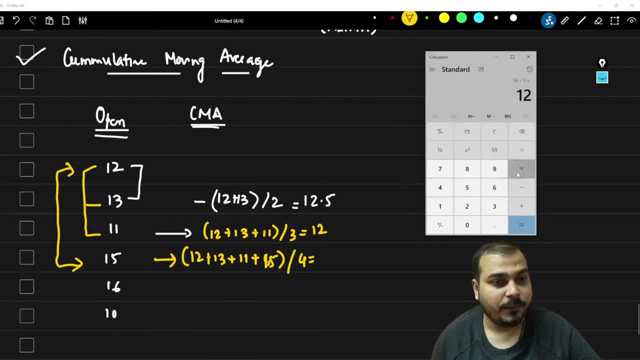 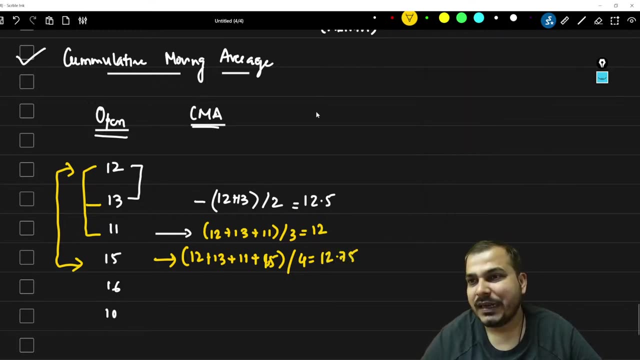 help of calculator. So it will be multiplied by 3 plus 15 divided by 4.. Similarly, you are going to do this, So here you are actually going to get 12.75.. Okay, So in this way you will definitely be able. 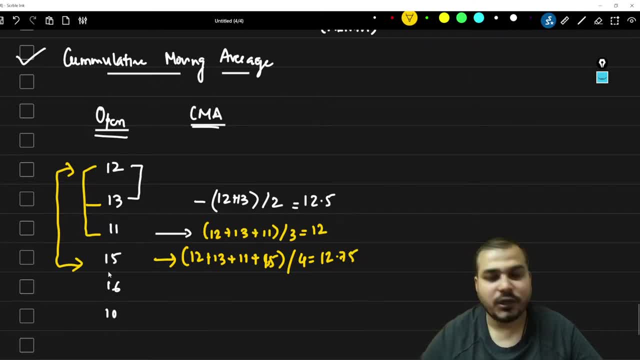 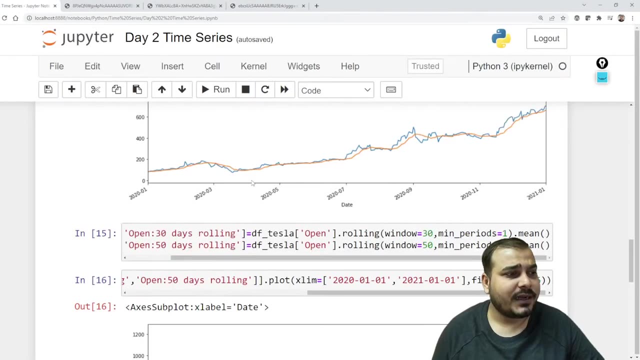 to get the cumulative moving average. Okay, So here what you are doing: as you are going down, You are actually calculating the cumulative, cumulative mean of all the values that are present in the previous date time stamps. Okay, So, in order to do it, practically what? 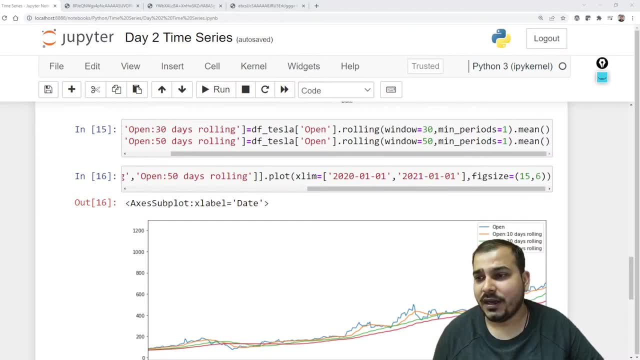 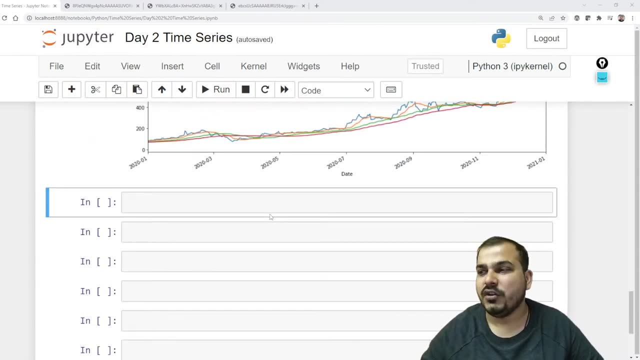 I am actually going to do is that I am going to basically write a code In simple way, And over here you will be able to see that it's very, very simple. You can just directly use expanding. So expanding is a function which can actually help you to find it out. 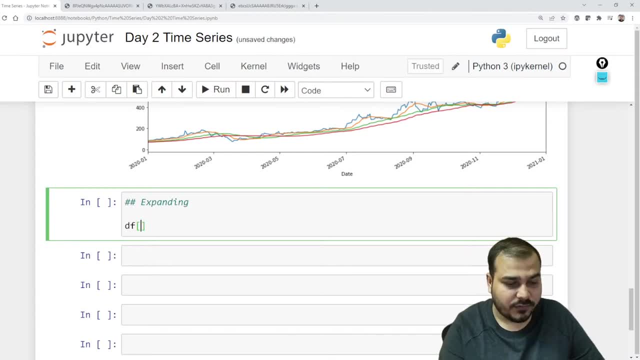 So expanding Okay. So if I write df of open, df, underscore tesla of open, Let me just write it down over here. So if I write df of open, Okay, Dot, There is a function which is called as expand, Expanding Okay. 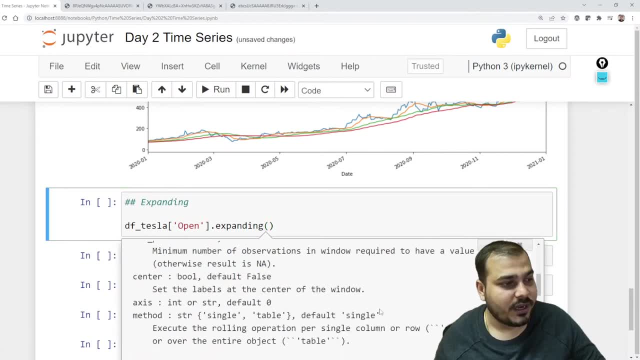 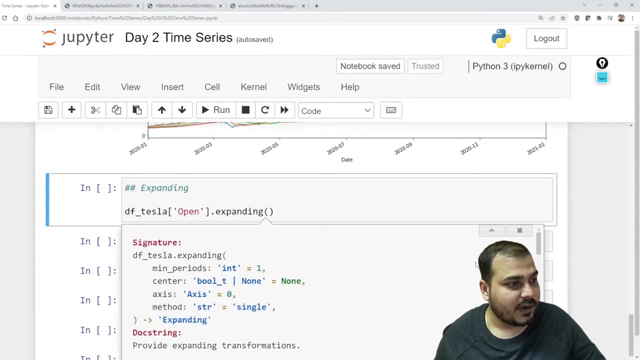 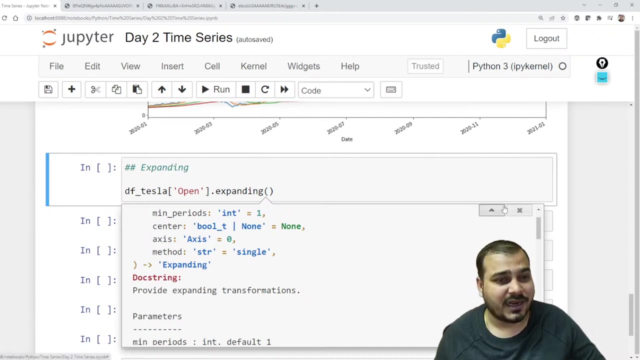 So if I press shift tab here, you will be able to see: minimum period by default is one. It says that The definition is not given Provide expand, Expanding transformation. it is basically saying: but definitely you will be able to find out what exactly is this. Okay, So if I probably 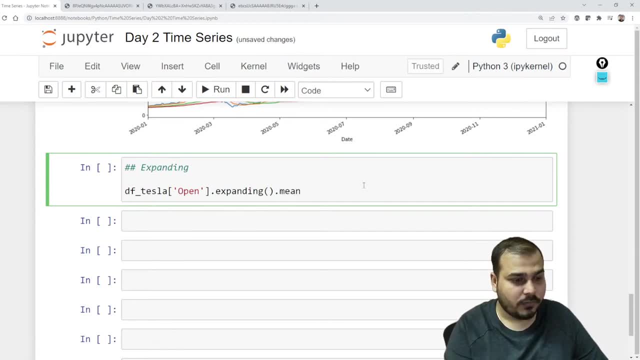 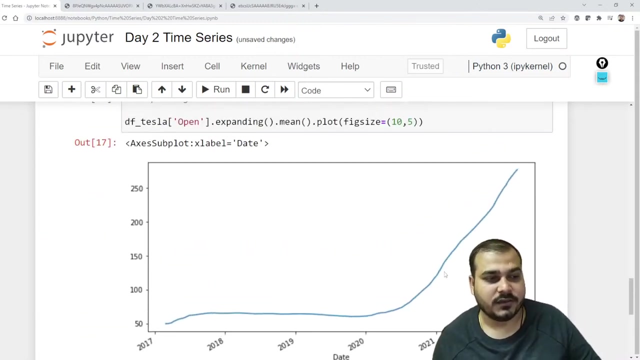 try to do just dot mean on top of it And probably say dot plot in some figure size, with 10 comma 5, let's say. Then you will be able to see that I am actually getting a plot which looks like this: Okay, 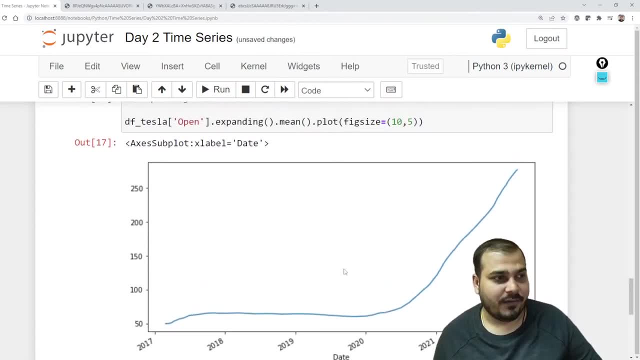 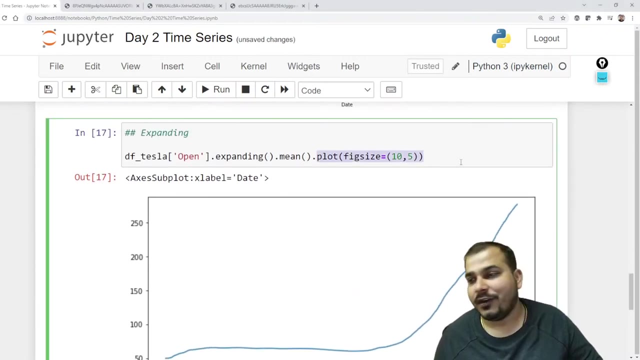 So this, as we go ahead, is this the moving, cumulative moving average of the open stock with respect to different, different years, which you are actually able to see over here. Okay, Okay. So here it is, and if you probably try to find out the dot head, 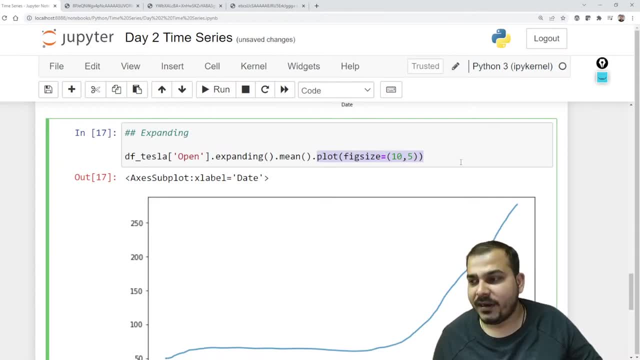 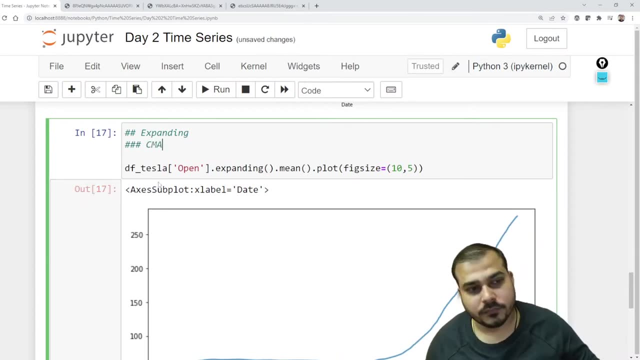 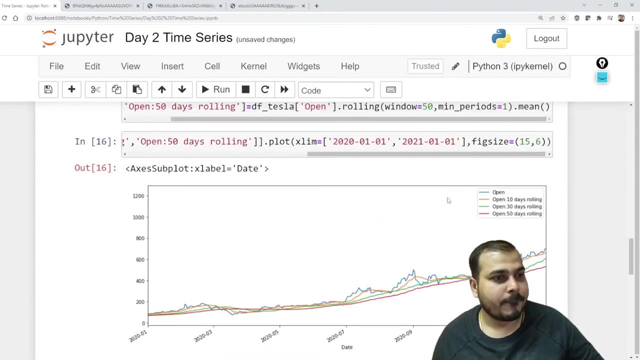 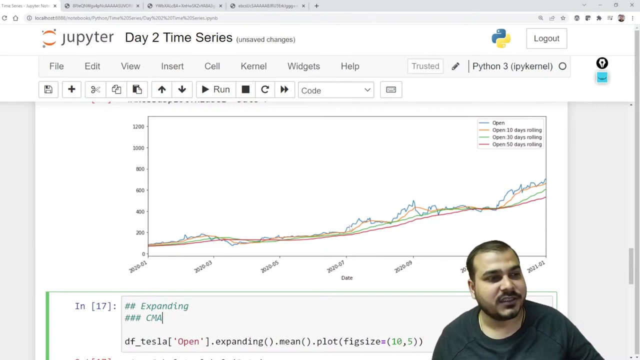 you will be able to see that. Okay, Okay, Everybody clear with this. So this was, with respect to cumulative moving average, Clear. So this is my entire things. with respect to rolling, This is my cumulative moving average. This is my simple. 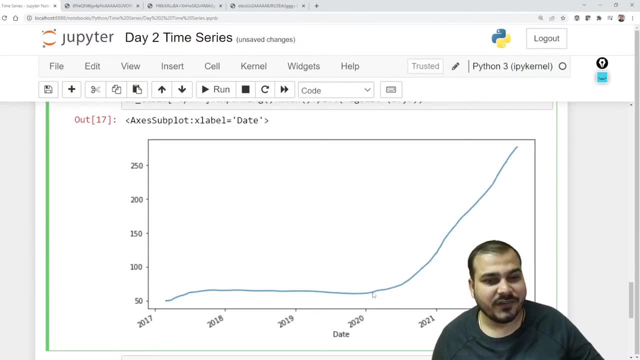 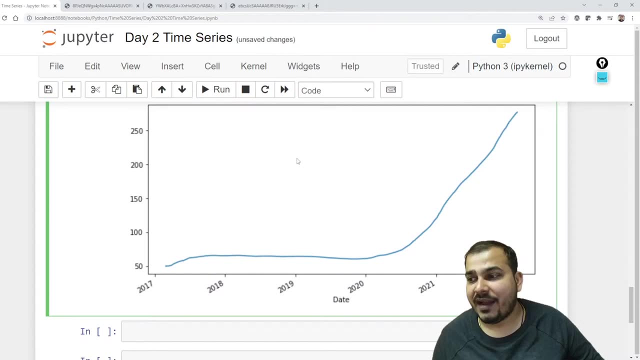 mean average. Okay, This is just to give you an idea like how the summation is basically happening. Okay, Here I will basically use mean. The average is getting calculated and here you can definitely see that the average is increasing. That basically means the stock price. 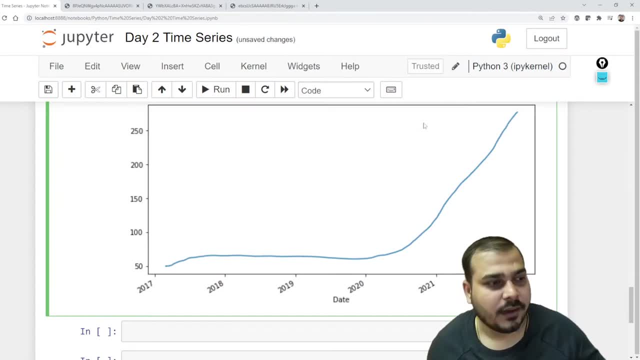 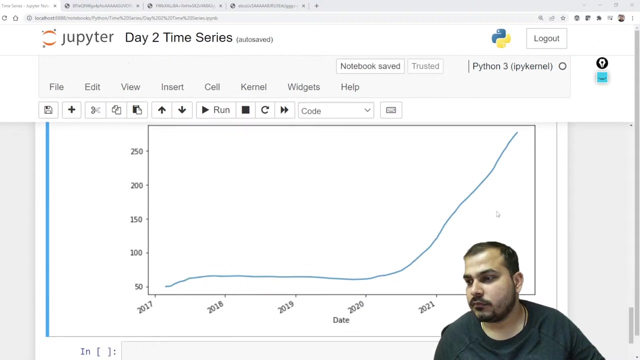 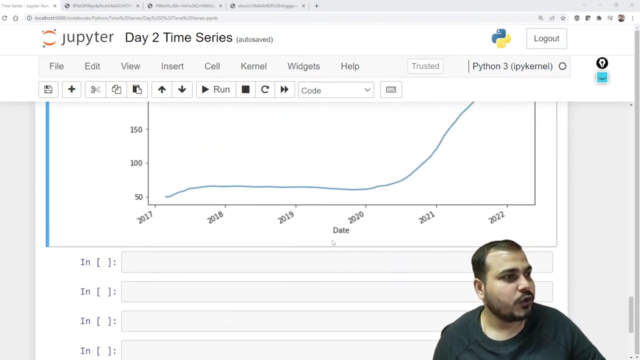 is also increasing. Yeah, It will calculate from the stock first index. Okay, Everybody clear, Everybody clear. Shall I continue. Okay, Now let's go to the next step. As I said that, with respect to the simple moving average, there will definitely be a lot of 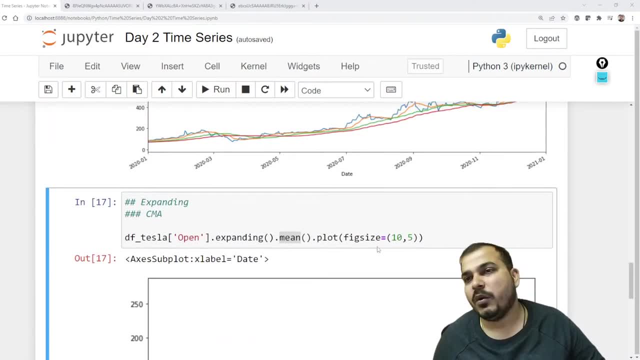 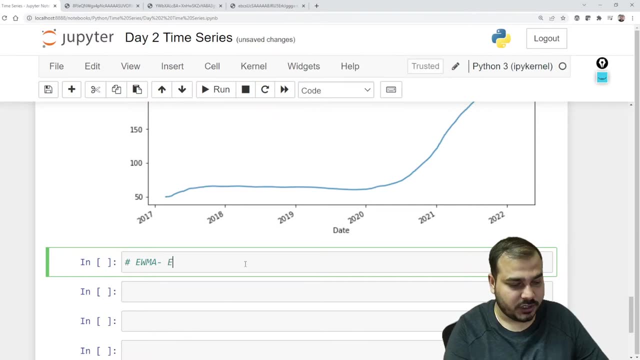 lags Right. We need to try to find out an amazing way. as an example, Exponential weighted moving average. Okay, Exponential weighted moving average. So this is what we need to do. Till then, just write down the code, Everybody. 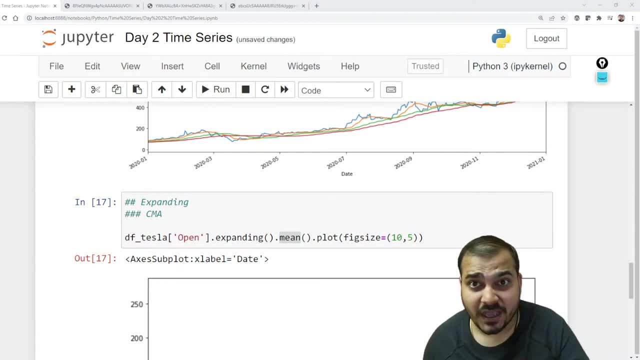 Exponential weighted moving average. Exponential weighted moving average Now in exponential weighted moving average. as I said, that our focus should be more on the current upcoming data or just on the recent data that we are actually getting, So that we can do the projection properly. Okay, 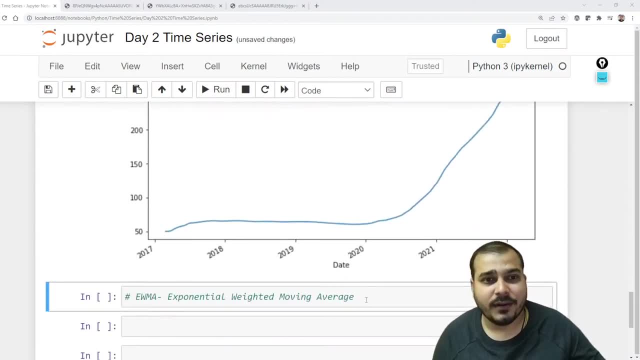 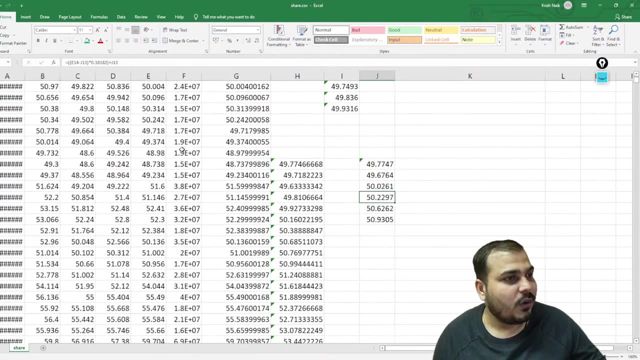 So for that we use something called an exponential weighted moving average. Let me just show you one formula, one amazing formula, with the help of a CSV file. Okay, Now, everybody, let's just focus on the CSV file. Everybody is able to see the CSV file. I will also give the 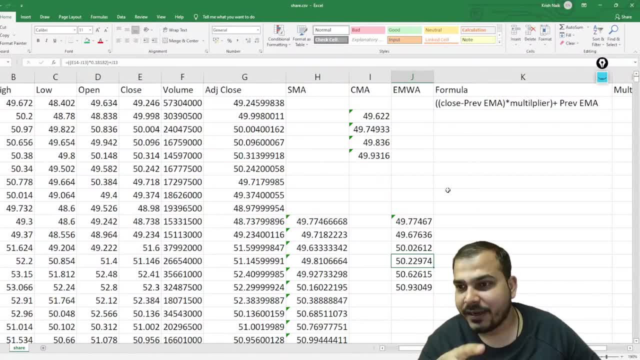 CSV file, probably in my, in my GitHub, so that you will be able to see this. Okay, Everybody is able to see this. Just let me know. Okay, Yes, Yes, everyone. Just give me a yes, Quick yes, Okay, Perfect So. 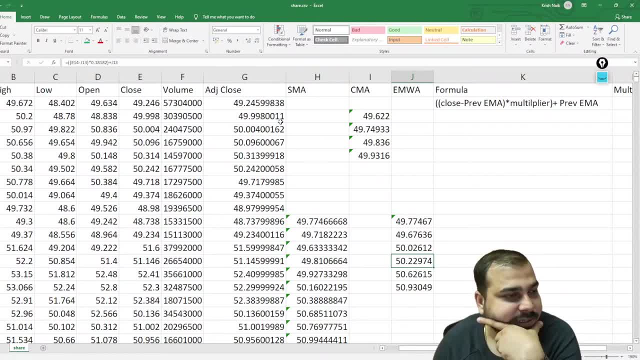 people are saying, yes, Perfect. Now what is happening over here? Let's see With respect to simple moving average. So this is my closed columns. Okay, So this is my closed column. Let's consider that this is my closed column of my stock data And 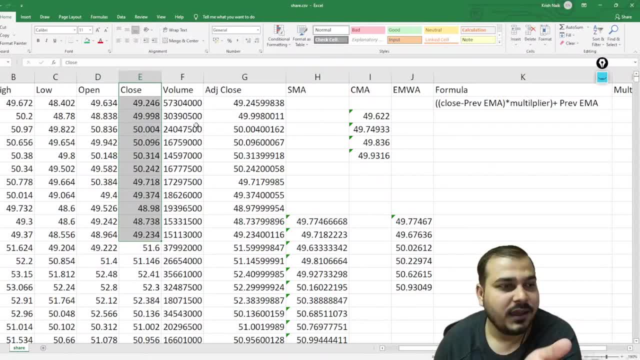 how did I create this stock data? With the help of the same thing. What I did? I just took that data set, I just did .2 underscore CSV and converted it. Now, with respect to simple moving average, Let's say that my window size is 10 initially. Okay, 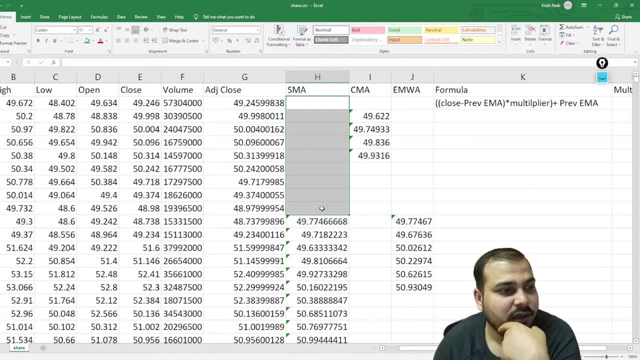 So this is my window size. Whatever window size, I have taken over here, What I am actually going to see the formula that I have done: Average of E2, colon E10.. Okay, Everybody is able to see the formula: Average of E2, colon E10.. 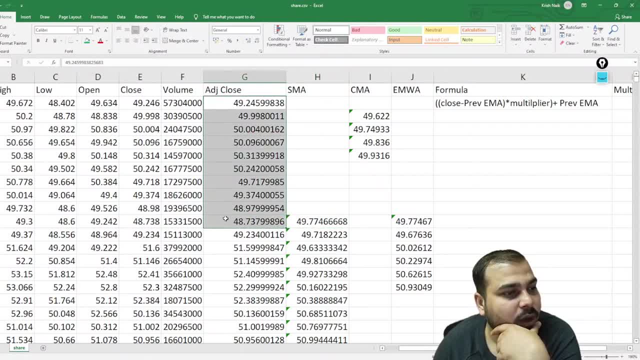 That basically means my: this entire average will probably give me the values of this specific simple moving average, Right? So here I will be able to see that I am getting the simple moving average over here. Similarly, all the formulas E3 to E11 will basically give me this: 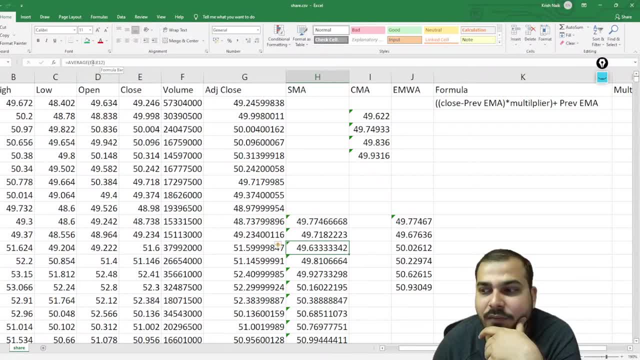 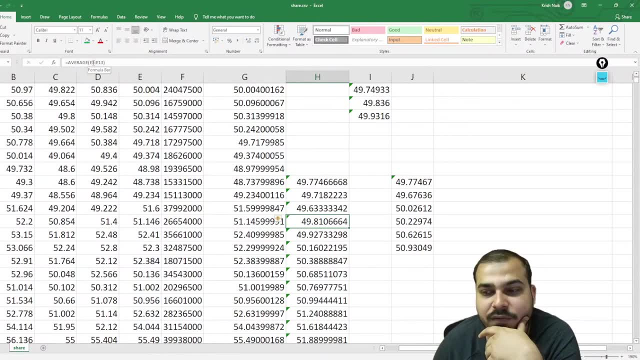 E4 to E12 by applying an average formula will be: basically give me this And probably you will be able to see 49.81. I am actually able to get the average of E5 to E30.. Right, So this is what we have done with the help. 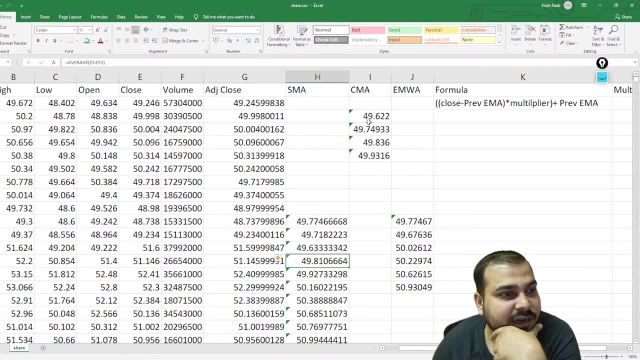 of simple moving average. Now second, cumulative moving average. Now see, with respect to cumulative moving average, what I have actually done. Suppose if I really want to find out the cumulative moving average, Then initially whatever for this specific row. If I want to calculate I have to basically do the submission. 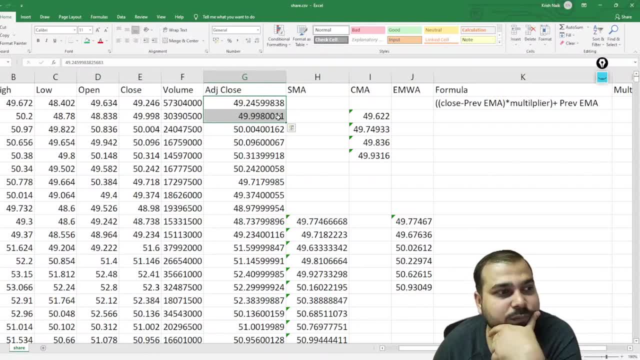 of both of this Right. Once I do the submission and average of both of this, then I will be able to see this. So here you can see E2 to E3.. I am actually doing the average and I am actually getting it Okay. 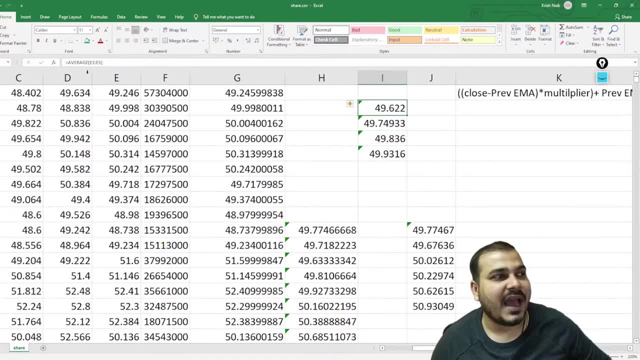 So formula is not visible. Don't worry, Formula is simply a simple average function in excel sheet. I cannot expand that. Okay, Simple average function. So here, if you want to see Here, you can see average E2, colon E3.. Okay. 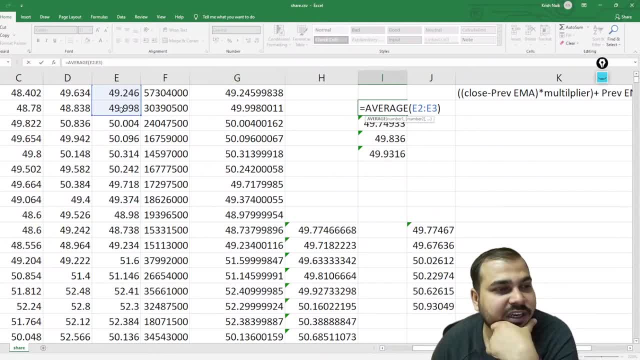 That basically means this two- Sorry, this two- E2 colon E3.. Similarly, if I go and probably open this Average E2 colon E4. So this is all three data. I am actually going to do the average and I am able to go. 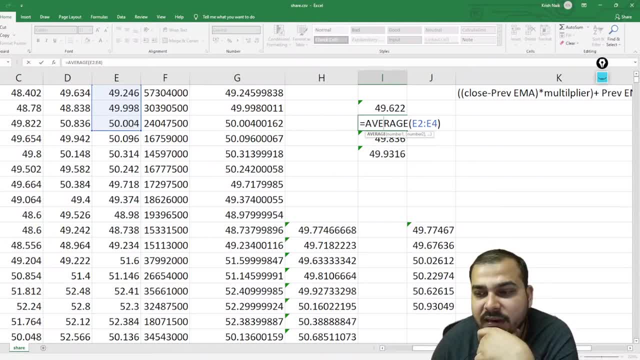 to find it out. Okay. And similarly, if you probably go and open this, it is E2 colon, E5. Right Average of this. And similarly, if I go and see E2 colon, E6. So this is nothing but cumulative moving average Clear. 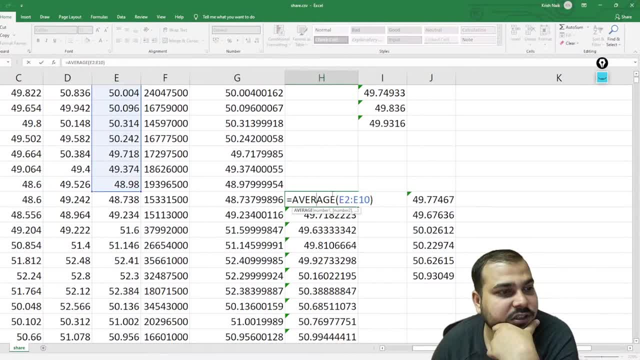 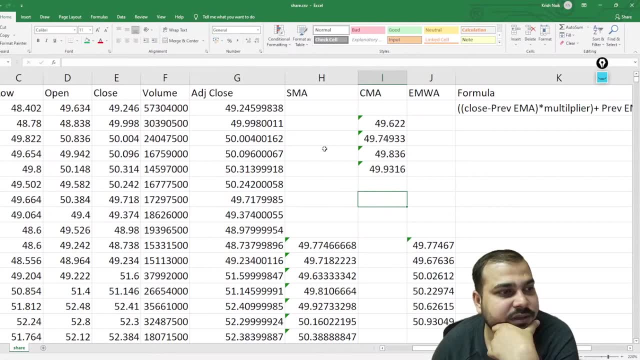 everybody Similarly over here. for the simple average, you can see: E2 colon E10.. E3 colon E11 and E4 colon E12.. So this is very, very simple, very, very easy. Do you want to show? Do you want me to show, like how the 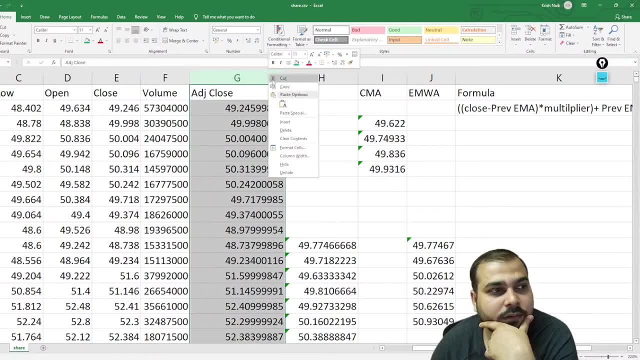 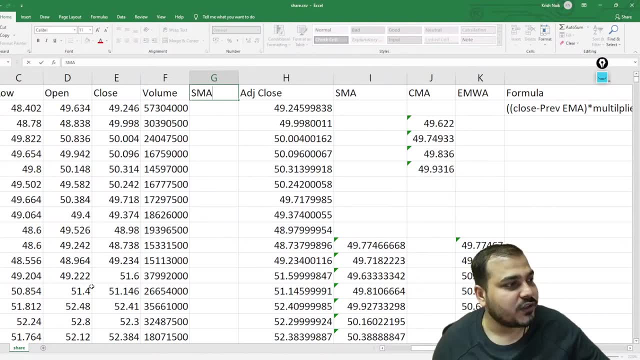 calculation is basically done again. Everybody is interested in excel, So let me just show you. If you want to calculate the SMA, Let's say my window size is 10.. So for this 10 my previous data will not be there, Okay. 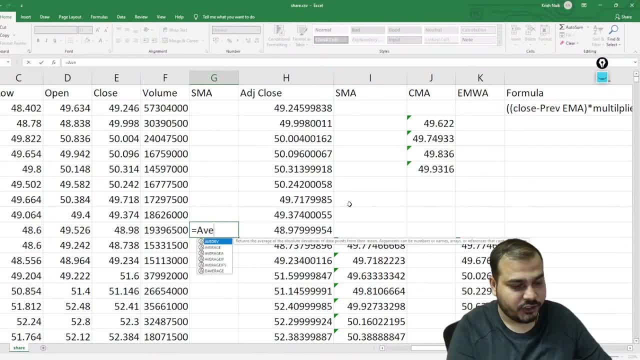 And here I am actually going to just write average, And here I am basically going to specify what should be my first value from here till here. Right, It should be colon. So this is just like E2, colon, E10.. So once I calculate this, 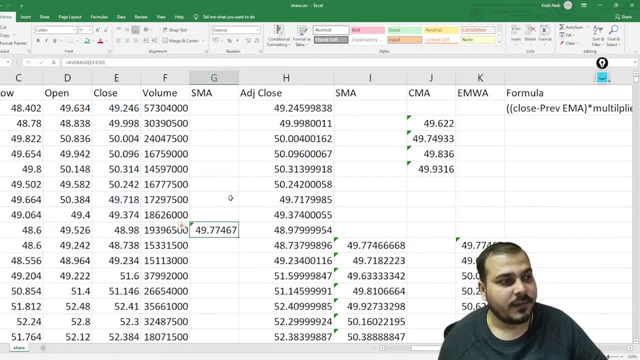 so this will basically be my average Right. Then, in order to calculate this again, I will basically write average and here I will specify what next one data till this. So E3, colon E11.. If I execute, I am actually being able to see this values. 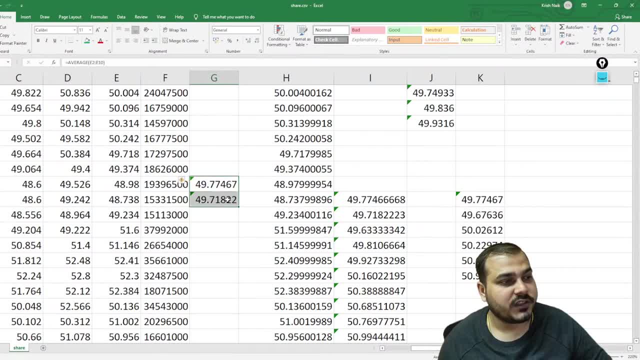 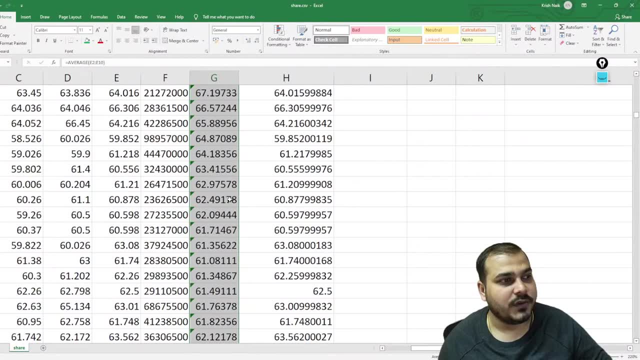 Okay, And now what I am actually going to do. I am going to select both of this and continue doing whatever I want to do for all the other columns- And here you will be able to see all the values- will automatically get done, Okay. 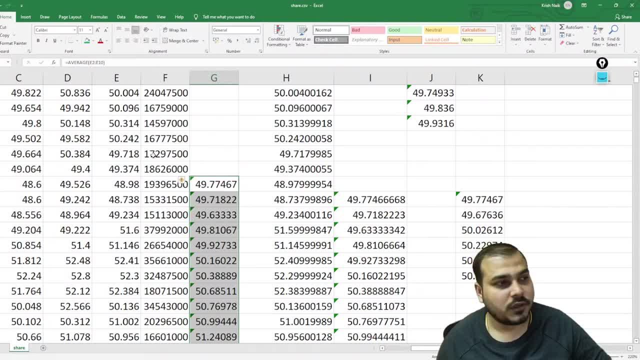 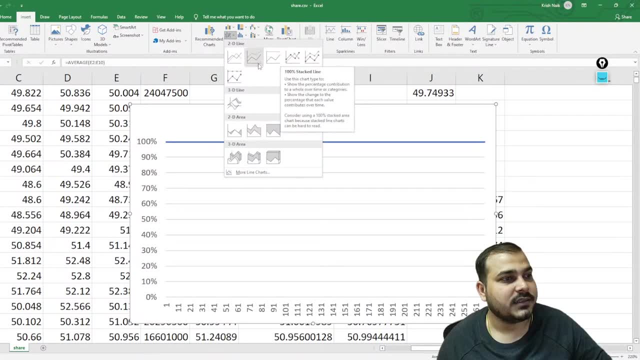 So you should know excel, Okay, And then you can insert any kind of charts that you want. Probably create it like this, Like this: See over here, Here is one chart, Here is one chart. Suppose I want to create this chart. 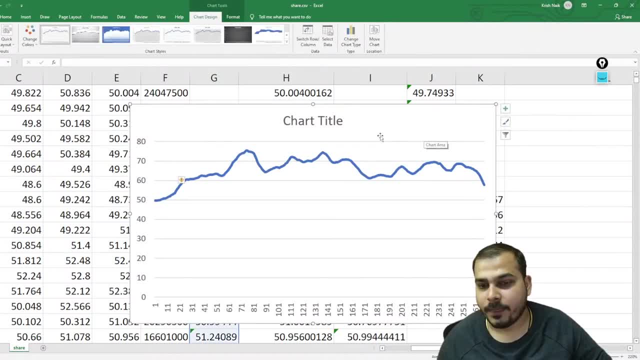 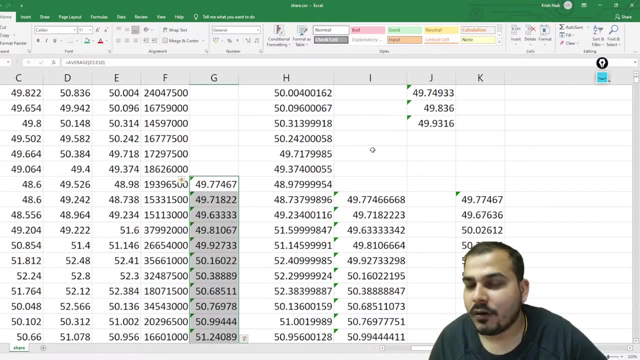 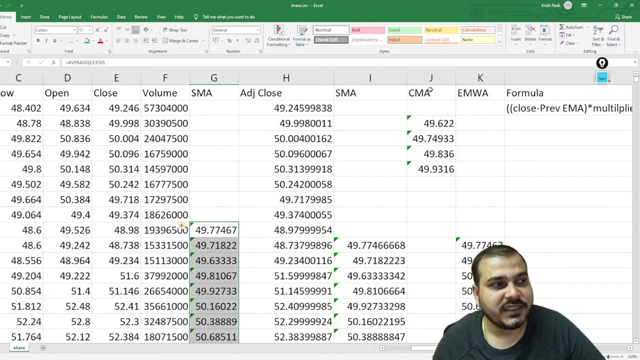 You can also create this Right. So please, as a data scientist, you should also know how to use an excel sheet. It is always better. Okay, Your work will become very, very easy. Now, quickly do it for CMA guys, If you can. 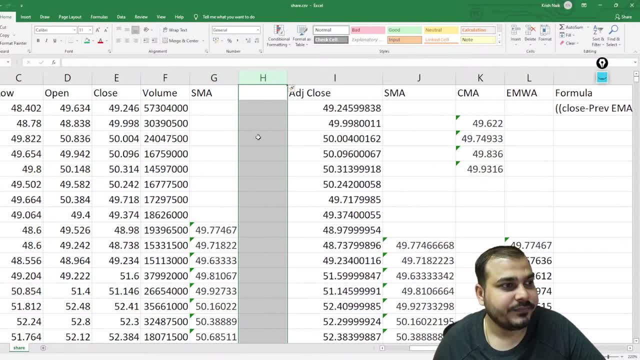 CMA is very simple again, In order to do it, just create a new cell. Okay, Suppose this. I say: this is my CMA. Okay, And for CMA, what I have to do, Cumulative sum, Right. So here I will basically write: 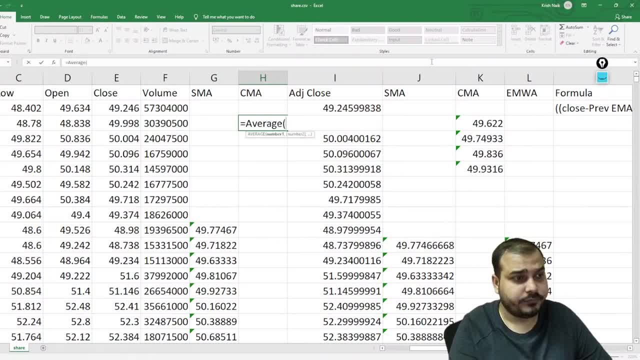 is equal to average, And here I am going to specify for, let's say, average for open. I want to do it, So I select this and this: Done: 49.23, Okay, But then next one, also again. I can do like this only. 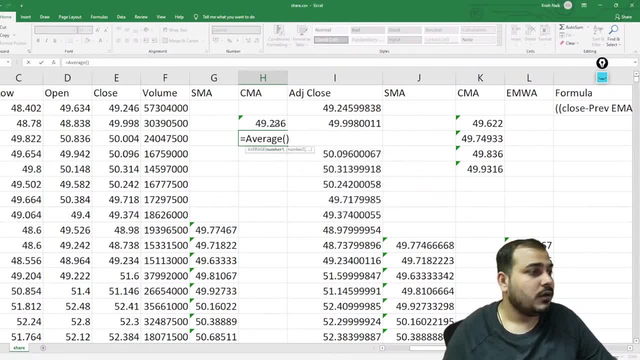 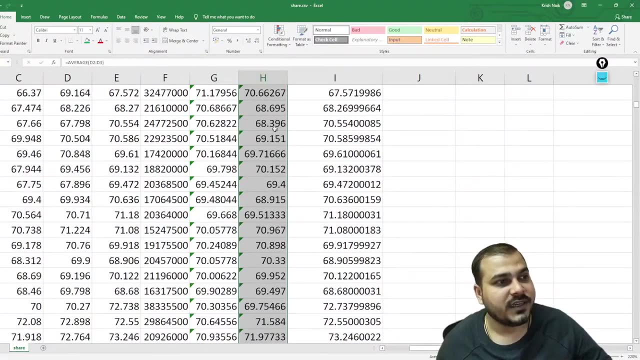 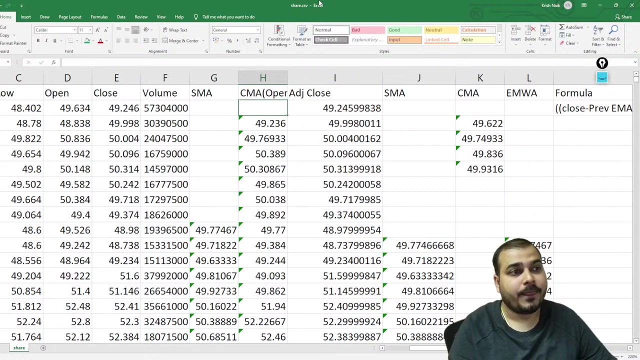 Average. So here I am actually going to take this to this Right And then you can probably do it for all the rows: Average open. This is basically for cumulative open Right. Previous one was for rows. Okay, Now I can also go. 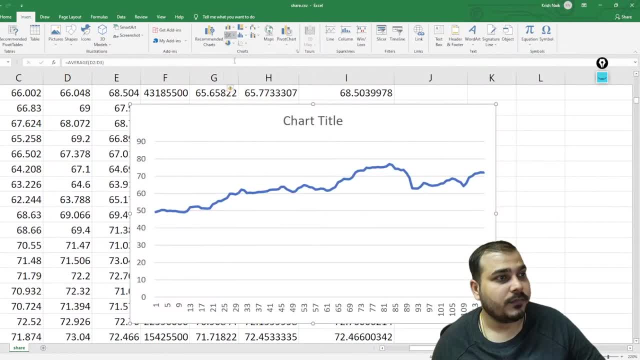 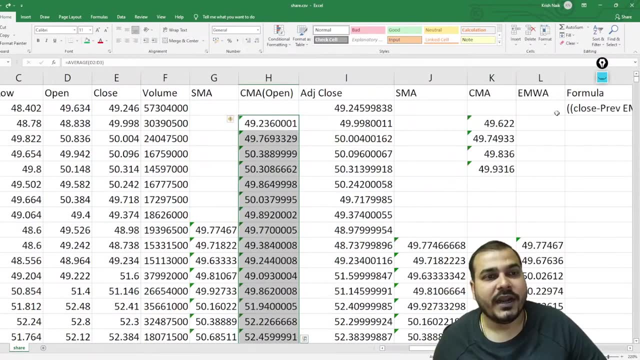 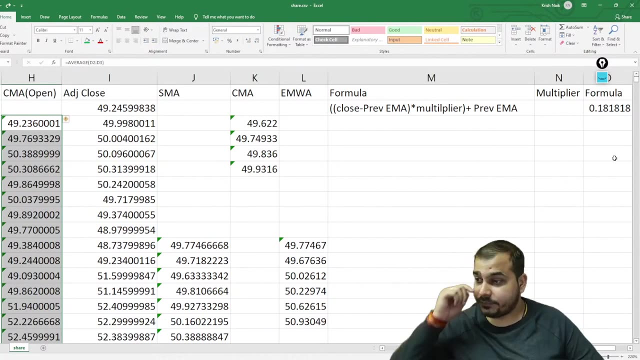 ahead and probably insert any kind of diagrams that I want. Okay, So this is how it looks like Very simple. Now let's go ahead and discuss about the EWMA: Exponential Weighted Moving Average. Now the formula is quite simple, guys. 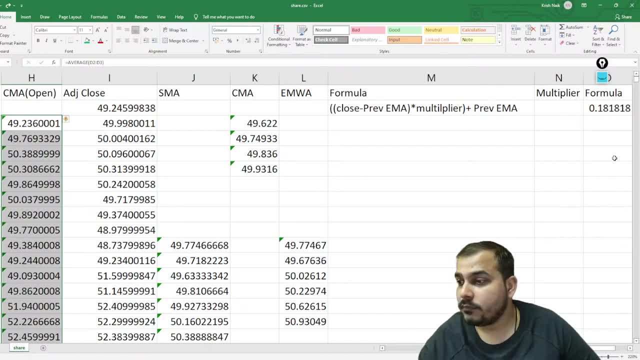 Okay, CMA formula: CMA formula: Average formula only is the CMA formula, Okay, Okay. So everybody ready for the next one where I am specifically discussing about this specific formula: EWMA- Exponential Weighted Moving Average. So in Exponential Weighted Moving Average. 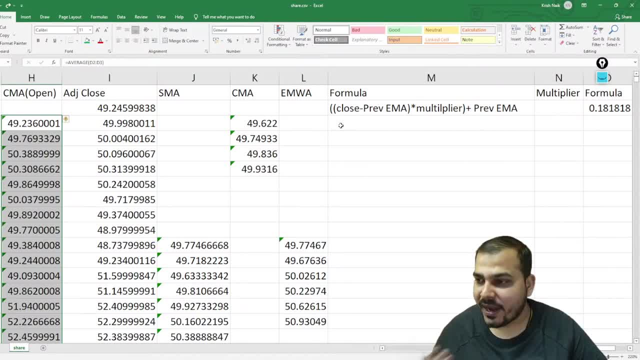 as I said that we really need to provide weights to the recent data. Okay, We really need to provide weights to the recent data. So here one example I am actually giving of the formula: What happens with respect to Exponential Weighted Moving Average? The Exponential Weighted? 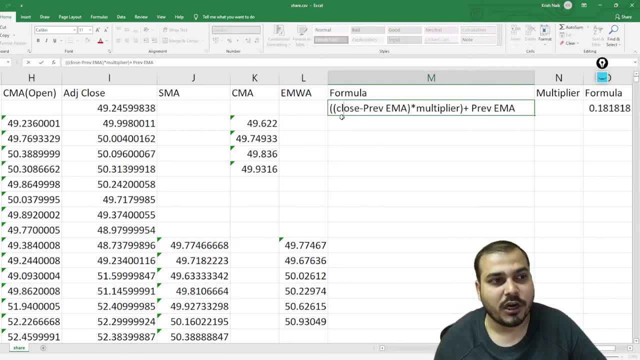 Moving Average formula is something like this: Whichever column you want you can take over here, like: close open Minus previous Exponential Weighted Average multiplied by a multiplier. What is this multiplier? I will talk about it. Okay, Plus again previous EMA, That is. 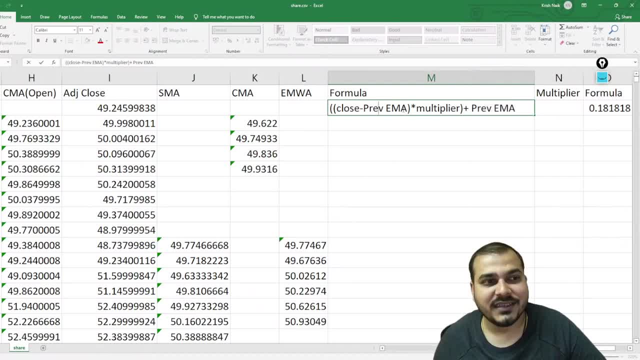 the Exponential Weighted Average. Now, what exactly is this previous EMA? Suppose I am just going to create a cell. Okay, Let's say this is my EMWA And suppose here also I want to keep my rolling window as 10.. 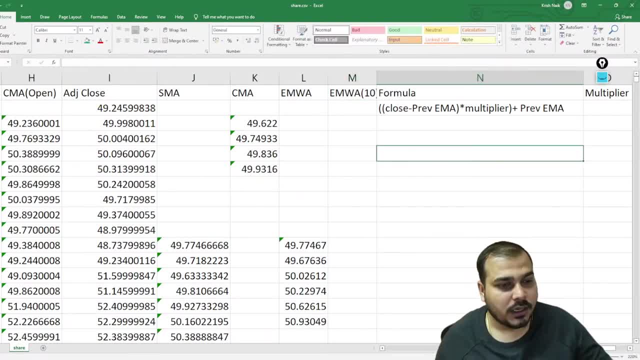 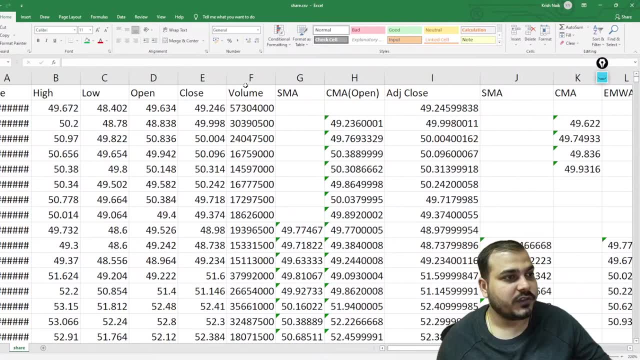 Let's say, my rolling window is 10.. Okay, Let me do one thing. Let me hide all these columns because I don't require it. So I am just going to select volume, volume: this, this, this, this, this and this, Let me hide it out. 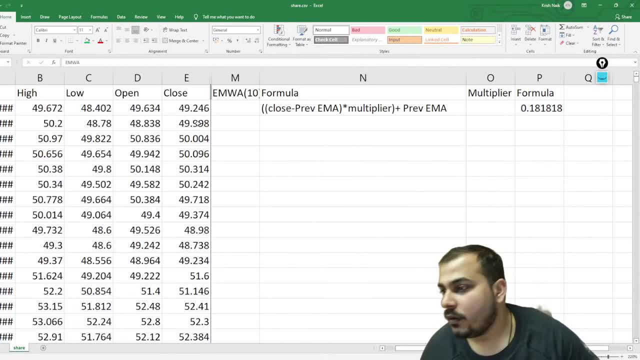 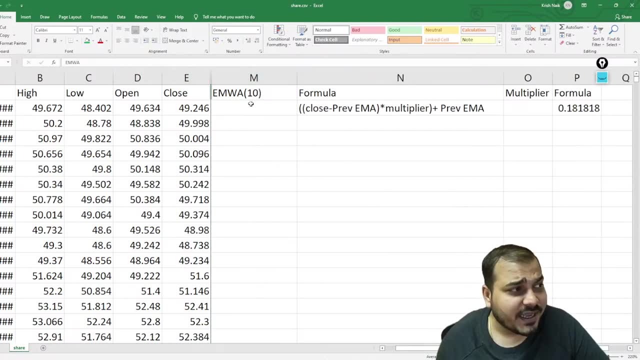 So this is hidden. Okay, So this is hidden. Now let's focus on this. Okay, Everybody see this. If I say that I don't have data for probably, My rolling window is basically 10.. That basically means for the first 10 records, If I probably. 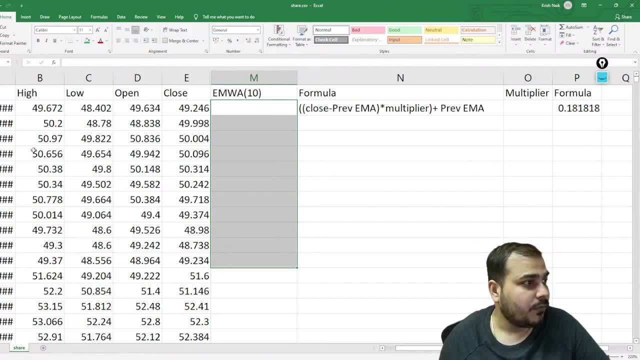 see, This is from 2 to 11.. Okay, So for the first 10 records I definitely will not have any data. Okay, And if I want to calculate the EWMA for this data, I obviously have to be dependent on the previous EMA, Right? 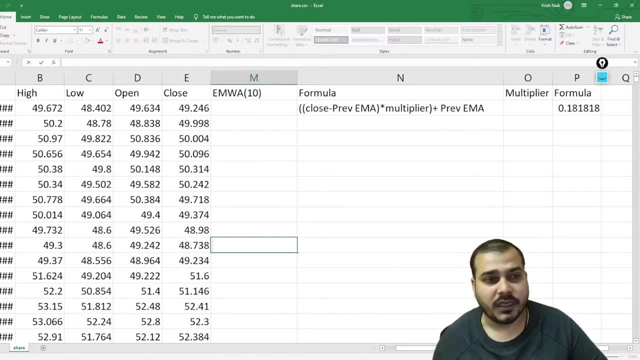 Previous EMA, But I don't have previous EMA, Right, Sorry, EWMA, It should be EWMA. Okay, Just a second Exponential Moving Average. Exponential Weighted Moving Average. Let me just verify the formula once, guys. 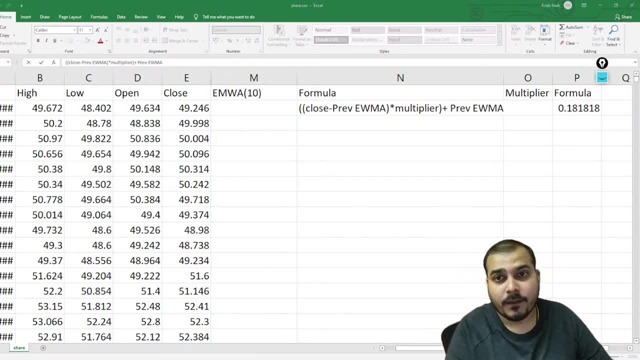 Because this formula is little bit weighted moving average formula, But an amazing one. I am just checking out the formula, Guys, Whether it is absolutely fine or not. 1 minus a, Okay. So this formula will change to something like this: 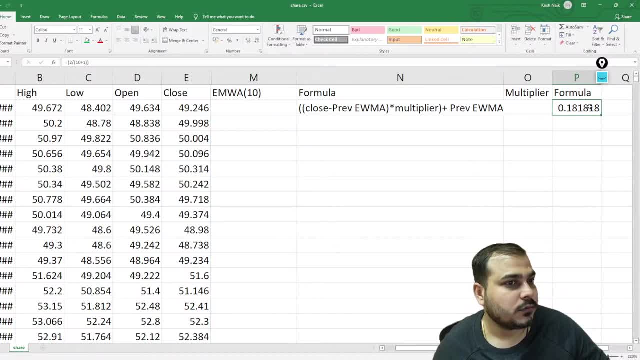 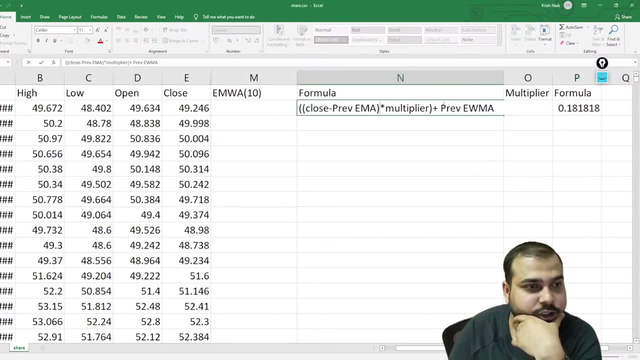 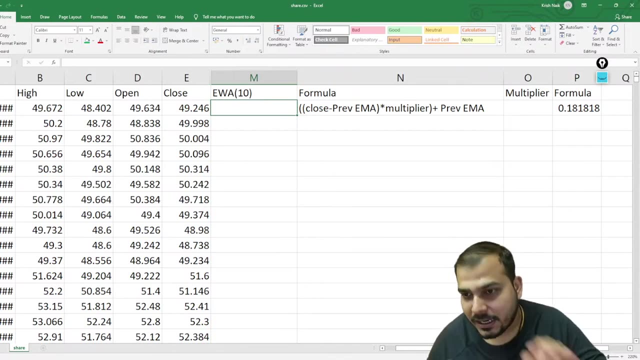 This formula is basically for Exponential Moving Average- Okay, Weighted one. I will discuss it. Okay, So this formula is basically for Exponential Moving Average. Exponential Moving Average- Okay, So this is just a change for it. I will discuss. 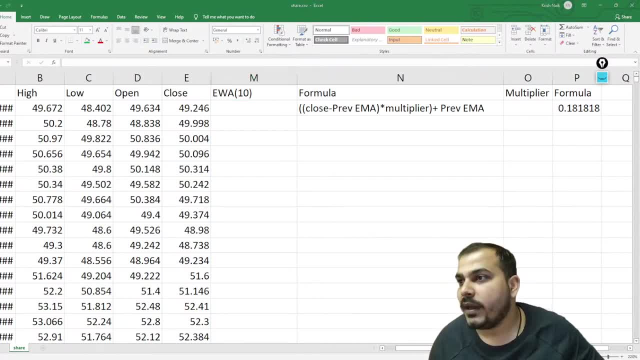 about Exponential Weighted Moving Average also. So don't worry, Okay, So, Okay, Perfect. Now everybody see over here, So here also I am going to write it down as EMA. Fine, Now see, Let's discuss. with respect to: 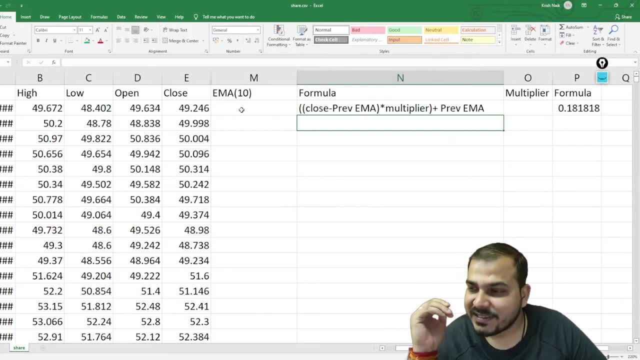 this Exponential Moving Average. Now, Exponential Moving Average basically says that I have to really focus on the recent data by providing some values or by multiplying it from some values, And based on that, Okay, We will try to see what are the values we will be getting. Okay. 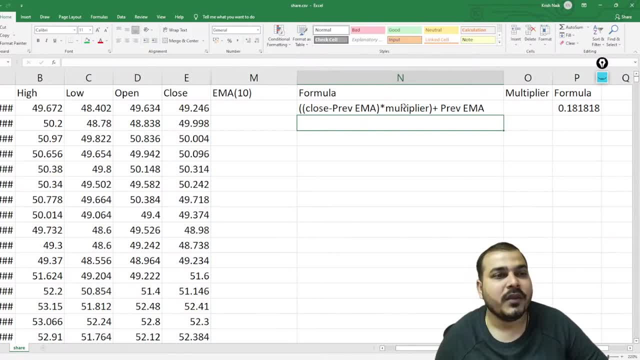 So here you can see that my formula is close, minus previous EMA. multiplied by multiplier plus previous EMA, That is the Exponential Moving Average. Now, obviously, when I say my 10 is the rolling window over here. Now for the first one, we cannot calculate EMA. 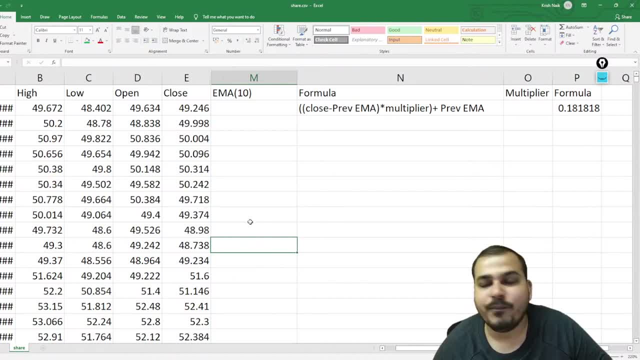 because this is the formula of EMA And for that we require previous EMA, And we don't have the previous EMA. Okay, Now, in order to get the previous EMA, what we should do is that we should start with the Simple Moving Average initially. 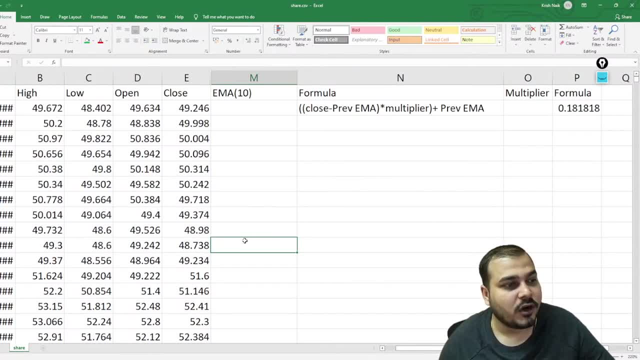 So if I probably talk about over here for the first 10 records, I will just try to calculate the Simple Moving Average. So I will say Average and here specifically I will write over here as this value. Let's say I am doing it for close. 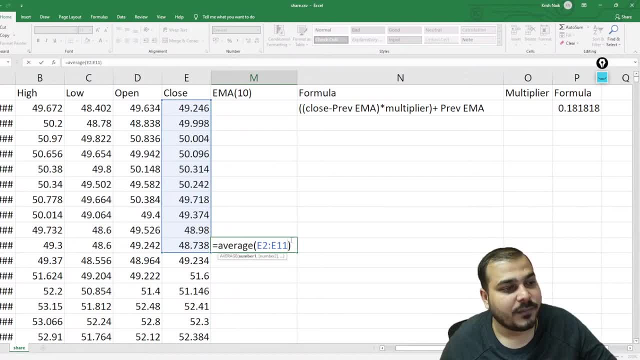 till this value. So this value will basically give me my average. Okay, Now, here I am actually getting the first Simple Moving Average, Because obviously I cannot calculate the Exponential Moving Average, because this is the formula for doing that. Now, the next thing, what I am actually going to do, is that 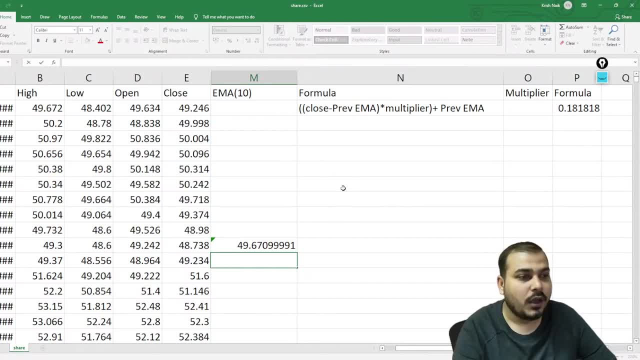 I am just going to apply this specific formula. Now, in order to apply what I will do, I will just write equal to, and this will basically be my brackets: Close minus What is close value over here. Close value is this one Minus What is the previous EMA. 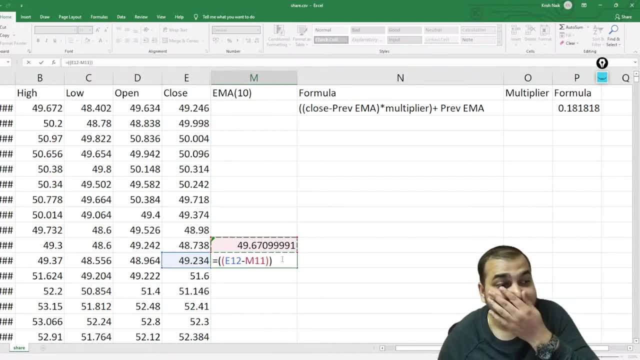 Now I have my previous EMA Right Multiplier is also there. Now, what exactly is this multiplier? I am also going to talk about it. What exactly is this multiplier? Multiplier is given by a formula Very simple And it. 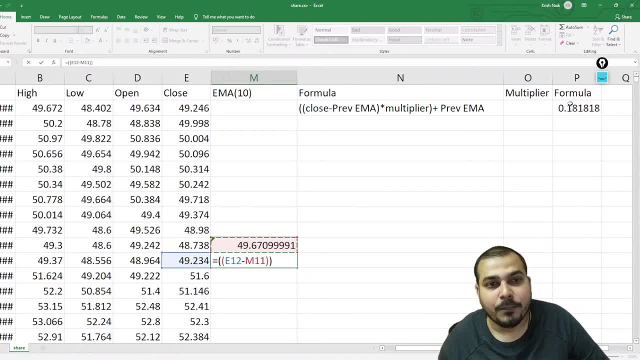 is based on the rolling size Right now, I have calculated the multiplier over here. Okay, Now, what exactly is this multiplier By default over here? I have calculated it as point: one, eight, one, eight, one, eight. I guess I am right. One, eight, one, eight, one, eight, Okay. 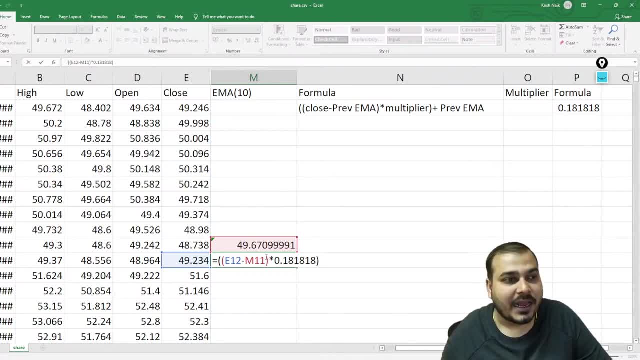 I will tell you what is the formula of this multiplier and how you are actually getting it. Then I will just say plus and my previous EMA- Let me show you my previous EMA- will basically be this specific value again, And I am just going to. 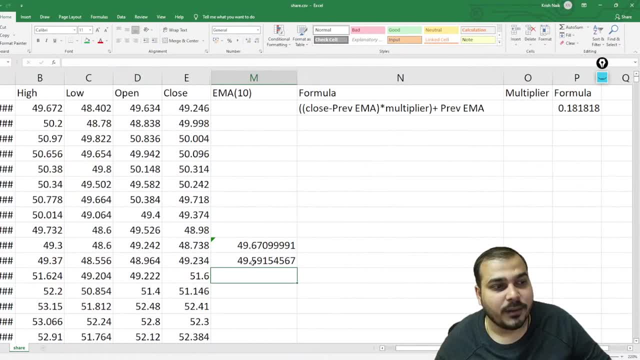 close this bracket and press enter. So here you can see that I am actually able to find out the exponential moving average over here. Now what is the formula of the multiplier? Multiplier is nothing, but the formula is very simple. It is nothing but two divided by ten. 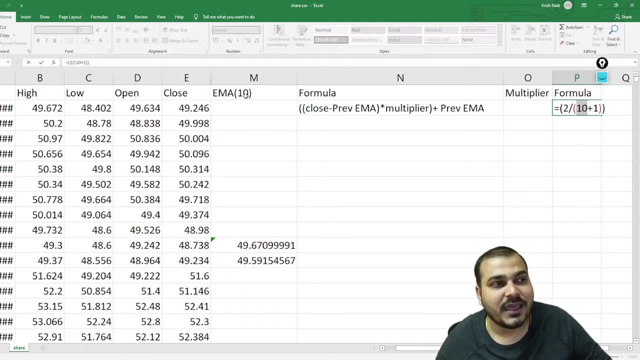 plus one. What is this ten? Ten is nothing. but whatever is my EMA rolling window size, I am actually going to get it as ten and this will be plus one. Okay, So by this particular formula we calculate the multiplier. Here we are not assigning weights. 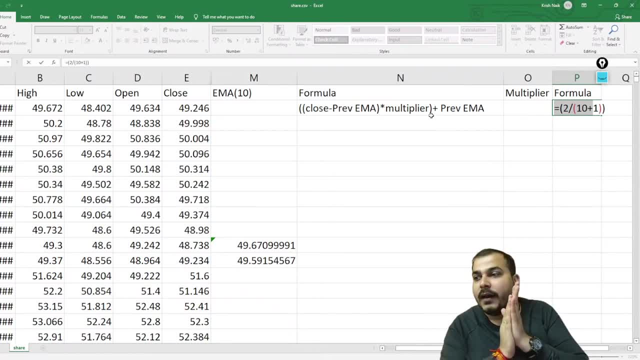 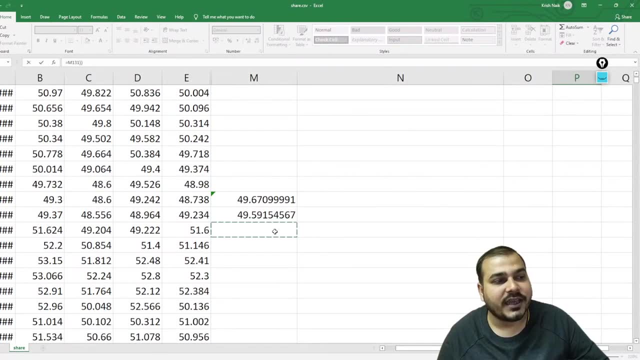 yet Okay, Here we are just focusing on using exponential effect in order to do the smoothening part. Now, similarly, I will go and calculate the next part over here And in the next part, what I am actually going to do. Just. 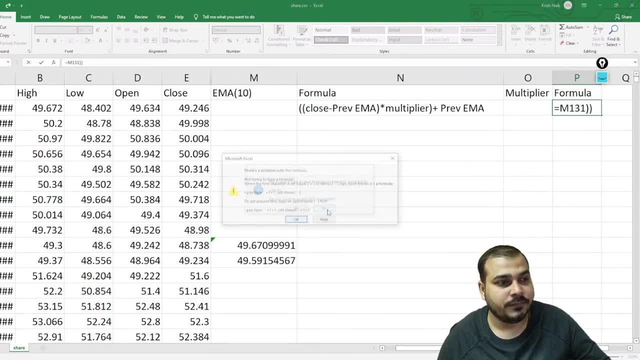 a second. Okay, this have actually gone. I don't know where it went, but here I am just going to write two divided by ten plus one. So this is the formula of it. Okay, Now the next thing that I am actually going to do. 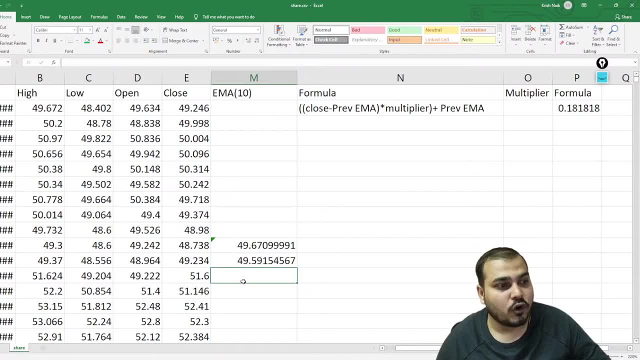 calculate it for this particular cell again. Again, close minus. here you can go ahead and calculate it. So here I am just going to write what is the close Close value. is this? Okay, I will just say equal to, and here I am just going to basically: 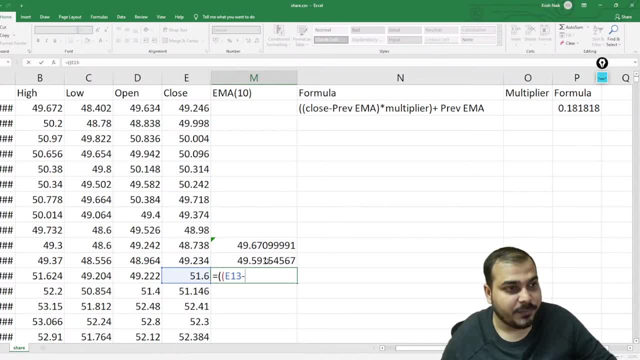 say close, minus previous EMA, and this I am just going to multiply by the multiplier. Multiplier is nothing but the same constant value, that is 0.818, Okay, 0.81818. and then I am basically going to say: plus previous EMA, Okay. 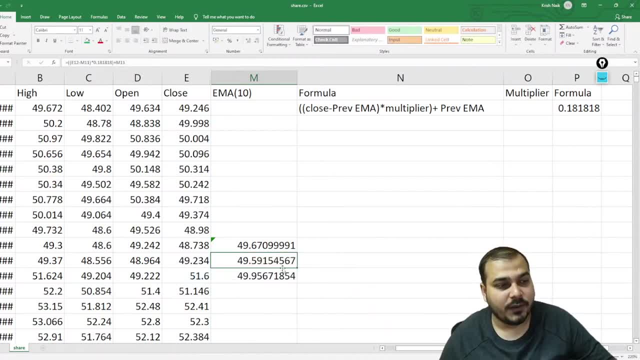 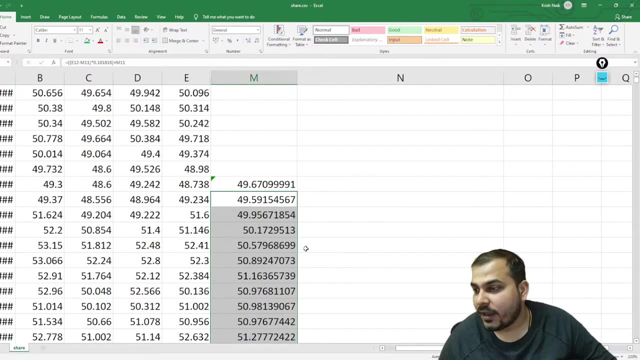 So previous EMA is this value, and I am just going to compute it Similarly, what I am actually going to do. remaining, all the computation will be done like this and I will be able to see my values like this: Okay, And this way also, we will be able. 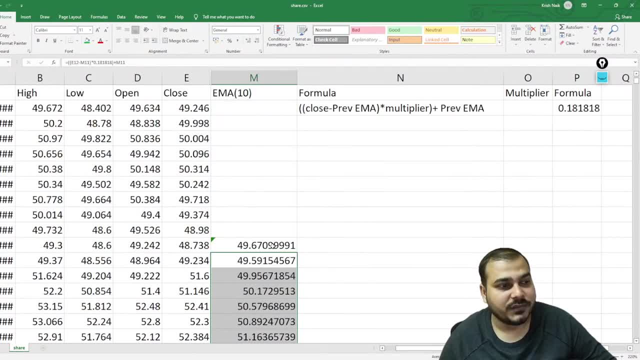 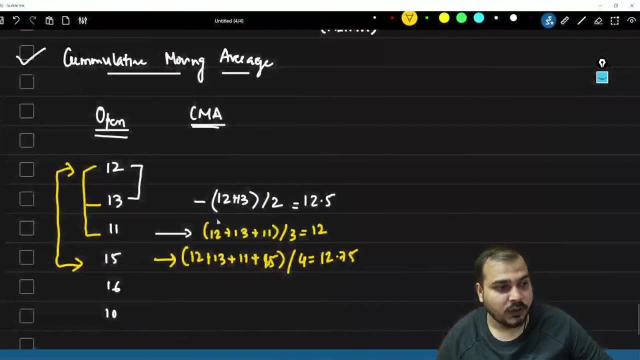 to see this With respect to all the values that we have calculated. Still, we are focusing on exponential moving average. Okay, But when we try to calculate exponential weight moving average, the formula will change little bit. Now how does my formula change with respect to exponential? 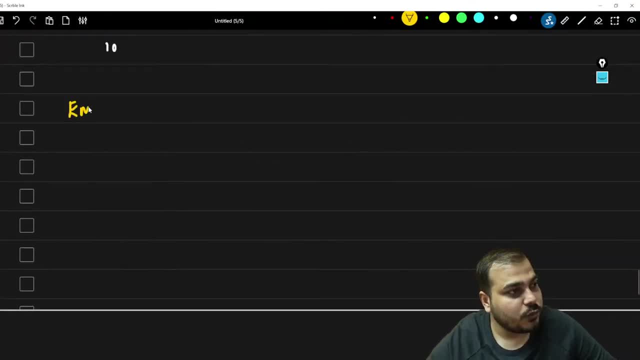 weight moving average. So here is what I am actually going to do. with respect to exponential weight moving average, The formula is very much simple. if I really want to calculate EWMA with respect to T, Then I can write A multiplied by X of T. 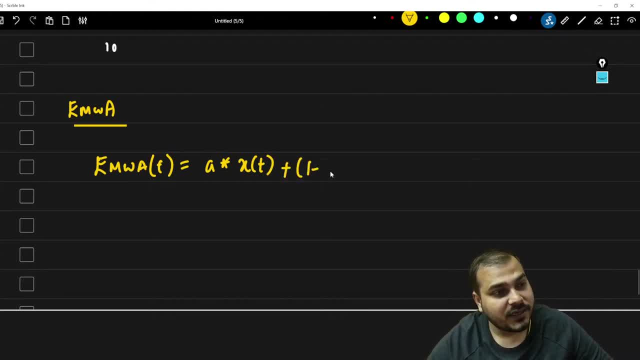 with some specific time stamp, plus 1, minus A with respect to the previous time stamp that I am actually trying to calculate, the EM WA T minus 1.. Okay, So here, what I am actually going to do is that this is specifically my weight, that I am giving. 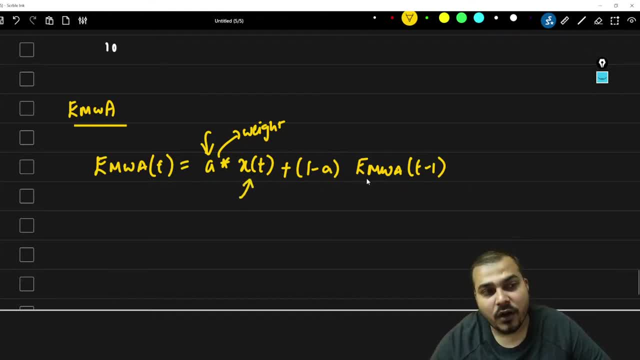 the priority to my first data instead of the previous one. Right, And this is specifically done to prevent any kind of lags. Okay, To prevent any kind of lags. Now, you should understand that. fine, Krish, this is very good, I know like. 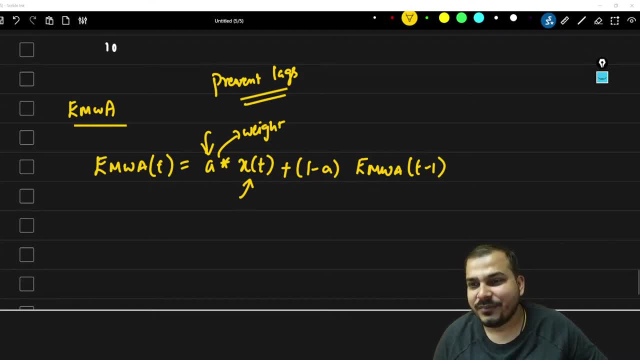 many people will hate equations and all, But we should have this kind of ideas how to basically do it. Okay. Now let me just show you exponential moving average. how do you write a code? Okay, So first of all, I will just try to. 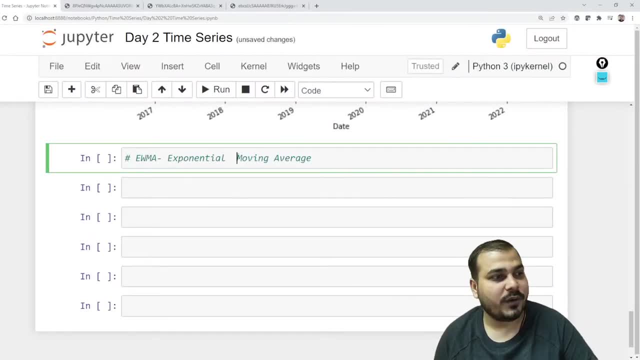 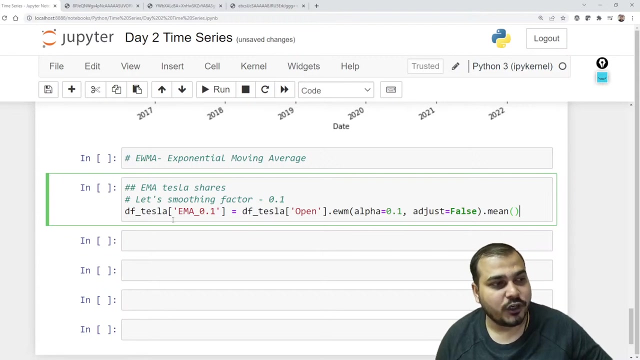 minimize this and let me remove this with respect to weighted moving average, and let me just write the code with exponential moving average. It is very, very simple Here. I am just going to copy the barcode and paste it over here. See this With respect to what I am actually doing with. 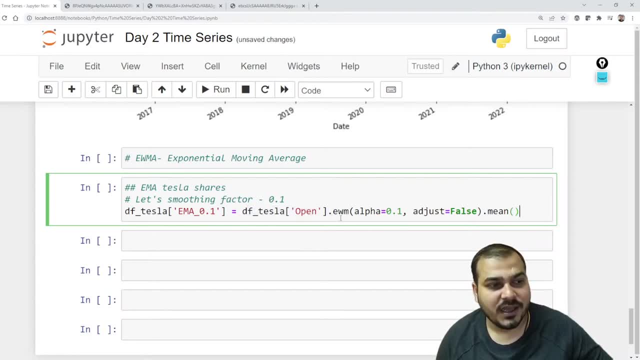 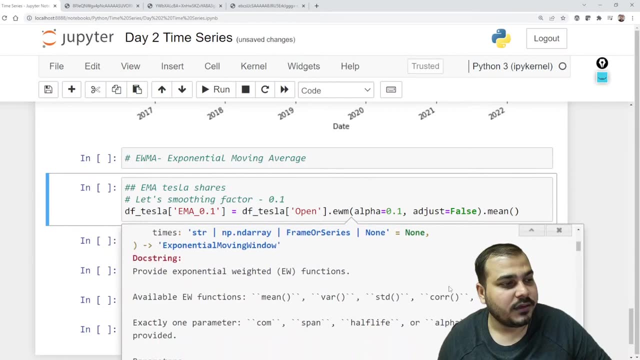 respect to exponential moving average. I have written df underscore. tesla dot open. There is a function which is called as EWM And if I probably press shift tab, you will be able to see that Here you will be able to see provide exponentially weighted functions. 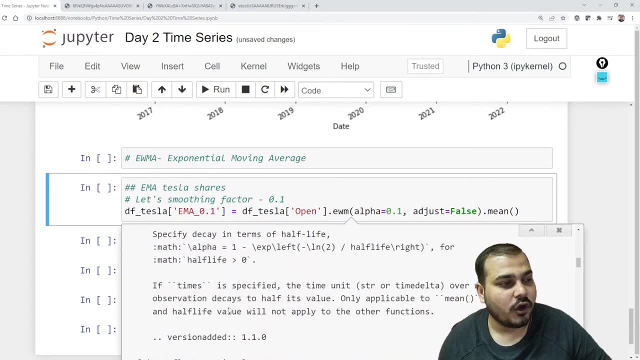 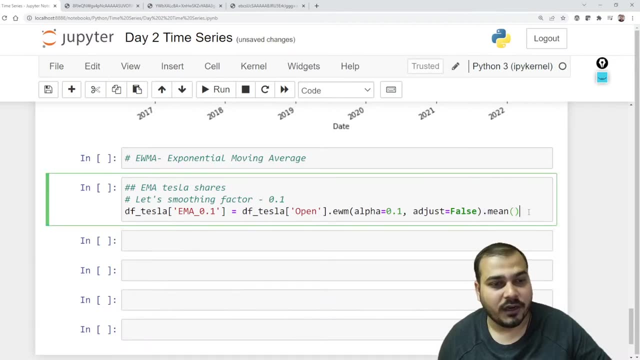 Here you specify one alpha parameter. This alpha is just like your hyper parameter, which is just indicating the smoothening factor. Okay, And then you basically just try to calculate the mean. So if I execute this and if I plot it with the 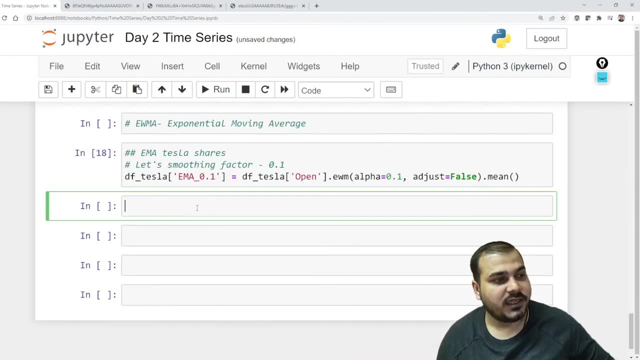 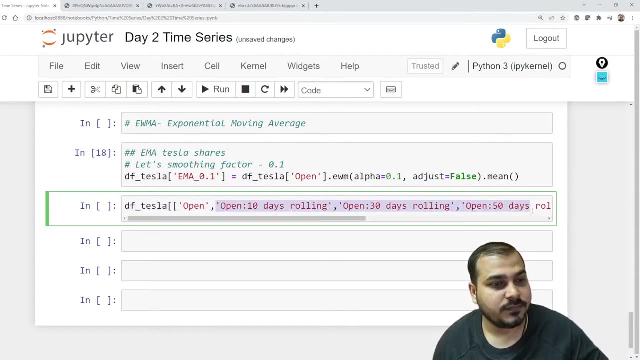 help of the same code, you will be able to see, the smoothening will be pretty much better without any lags. Okay, So here I am just going to remove all these things. I am just going to remove all these things, Okay. 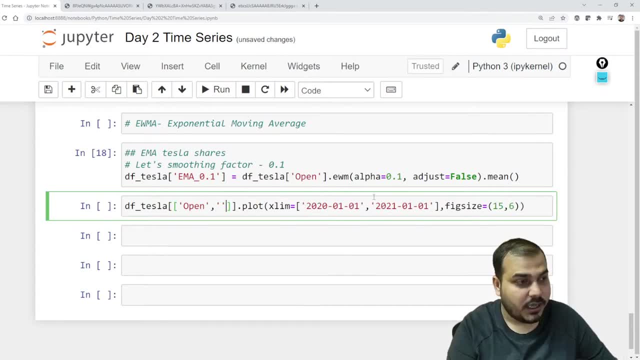 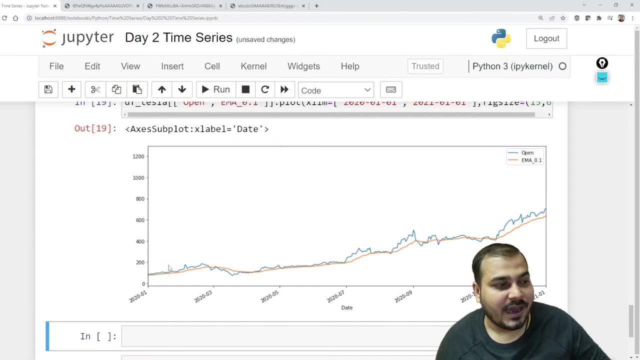 I am going to just make it 2 dash and here I am just going to make ama underscore 0.1.. Now, if I execute this here, you will be able to see that Now, without any lag, I am able to see the entire exponential moving average. Now what is? 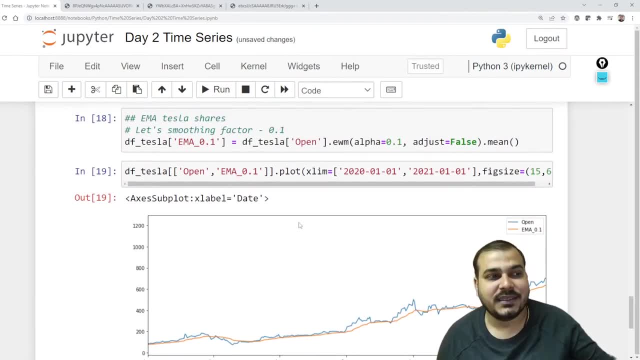 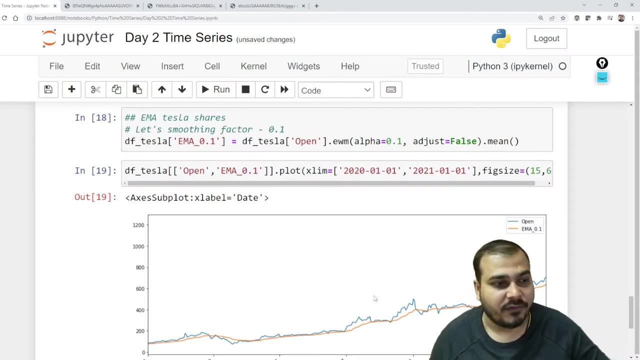 the advantage Understand. you are removing lags and you are also trying to find out the exponential moving average, which was pretty much better than the simple moving average. Now, with respect to that, you will be able to see this kind of data, And here you can see all the plotted data. 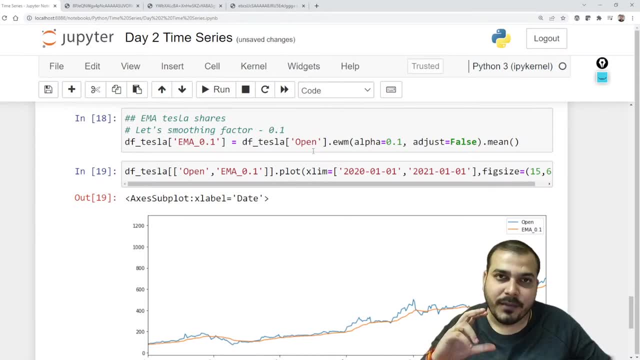 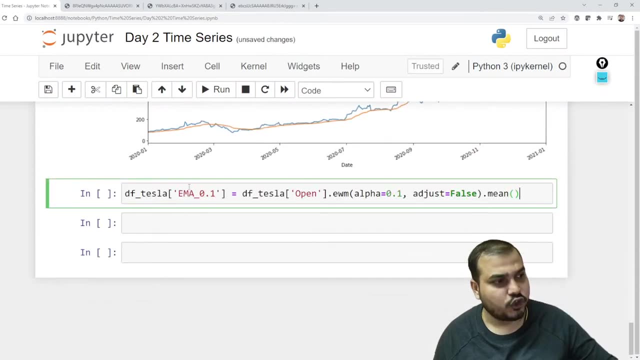 that is basically keeping The smoothening factor. if you want to probably make it more smooth, then you can play with different, different parameters. Let's say that I am just going to copy the same thing and now I am just going to say my smoothing factor. 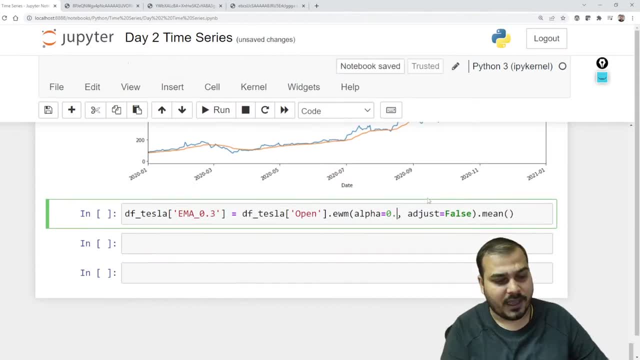 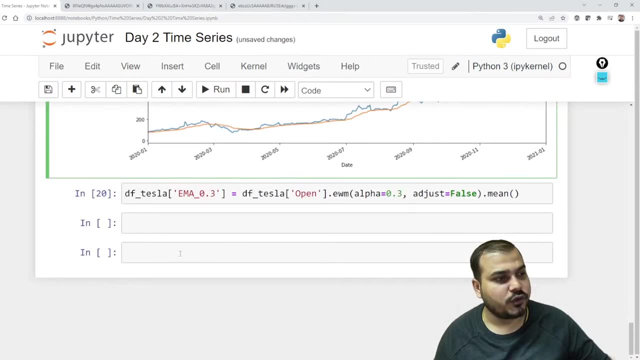 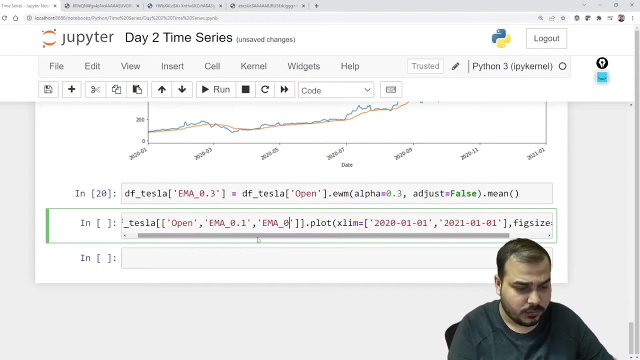 will be 0.3, and here I am just going to set my alpha value as 0.3, and if I probably execute it, you will be able to see that I am just trying to plot it over here with the help of ama. underscore 0.3. 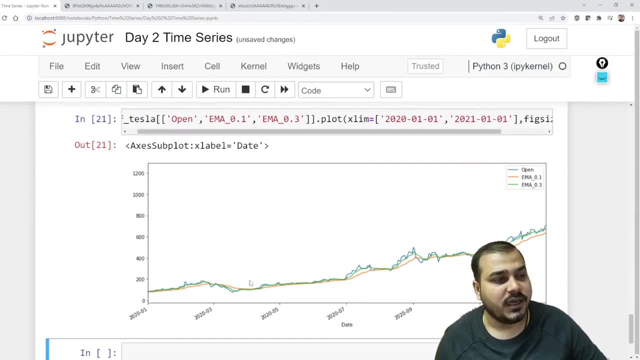 and here. if I execute it here, you will be able to see the other smoothing one, which is with the help of green color and it looks better than the orange one. It is more towards that specific data point. So definitely you have to try with multiple data points to. 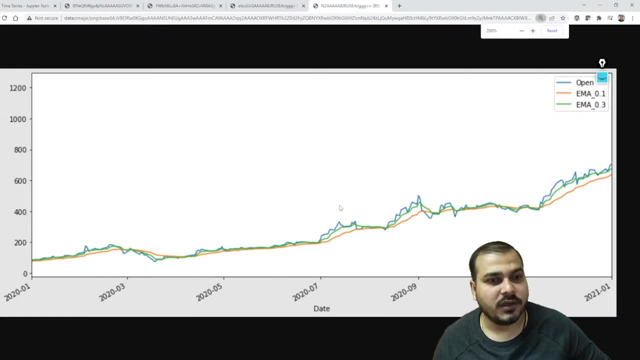 get it in a better way. If you want to see this image in a new tab here it is how it looks, like The green line that you are probably able to see. So alpha is basically a smoothing factor, Right? Everybody clear with this. 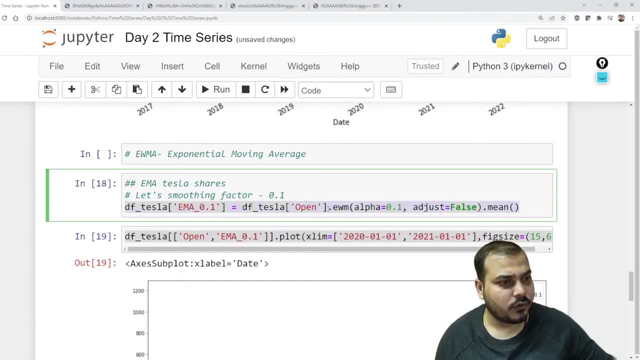 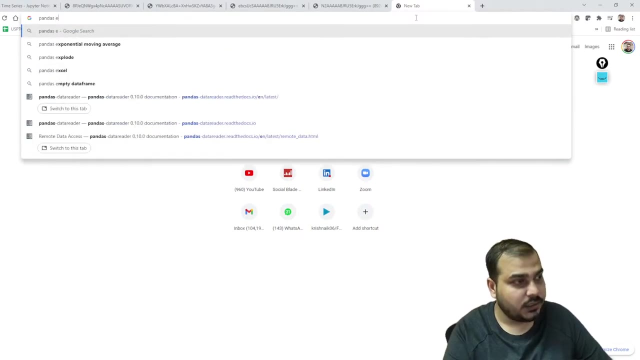 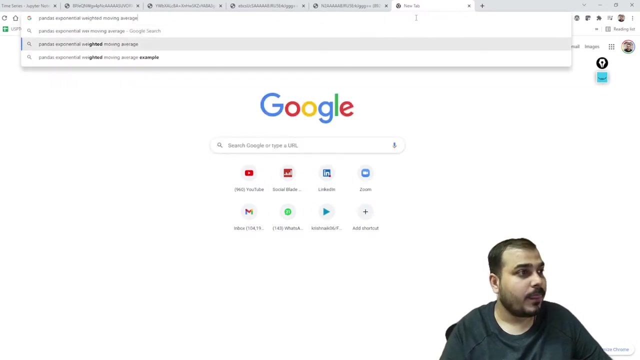 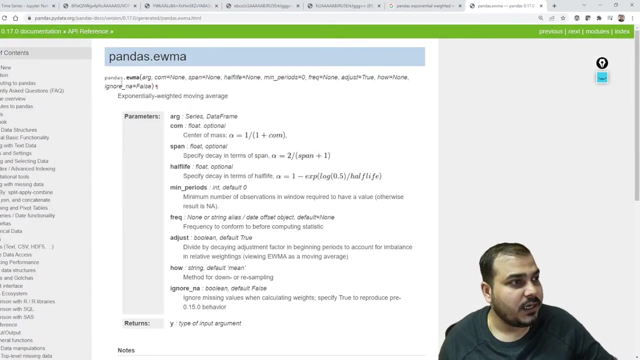 Let me see whether there is also an inbuilt parameter with respect to dot e. Okay, e w ma is not there. so if I write pandas e- exponential weighted moving average- So if I probably be able to see this here, it is. you can see pandas dot e w ma. 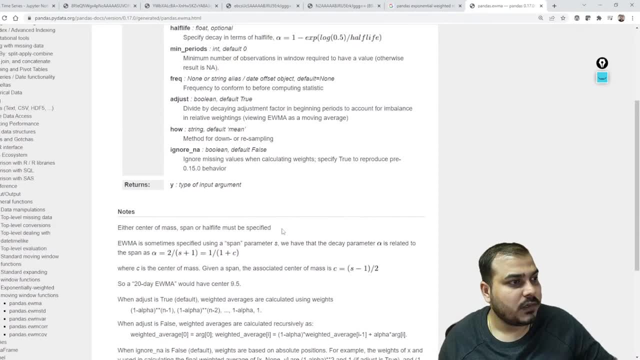 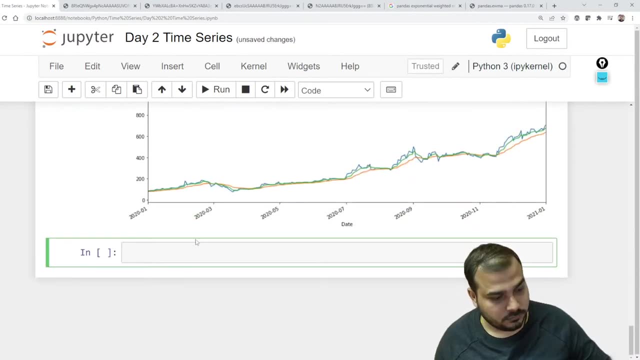 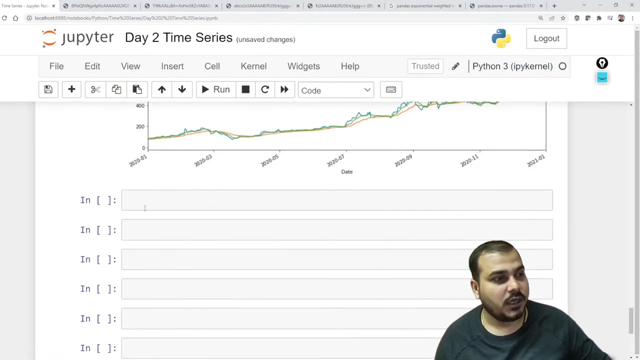 is also there. Okay, e w ma is also there. Let's see, Guys over here always understand there is no such optimal value. You have to definitely try with multiple values. So if I probably see there is something like e w ma, like e w ma. 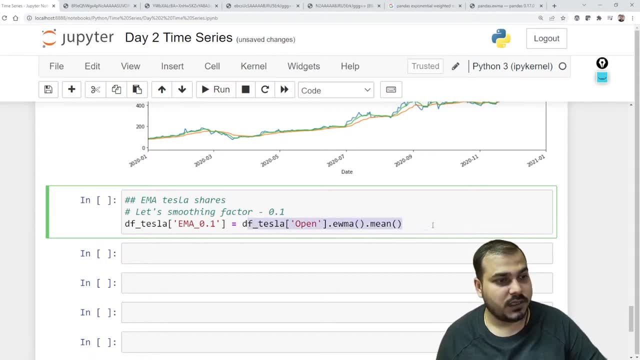 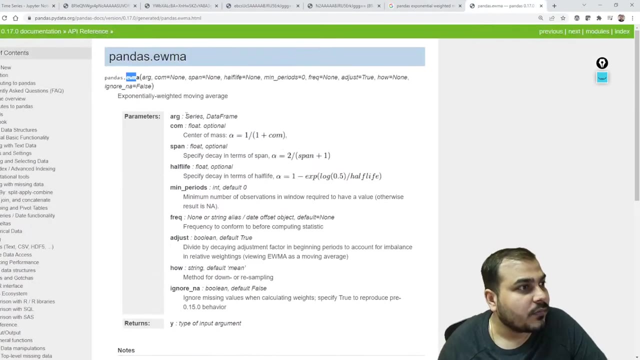 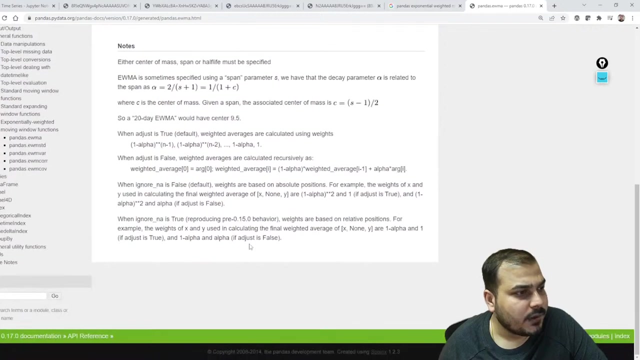 like e w ma. Is there any value like this? Is there any functions like this? I will just copy and paste it over here. I think it will get an error: e w ma is not there, or what pandas dot e w ma. Let's see some examples. 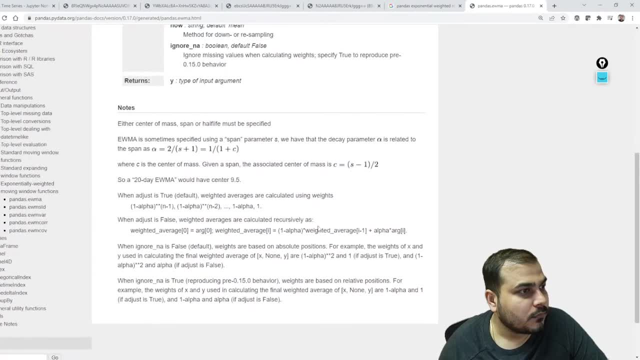 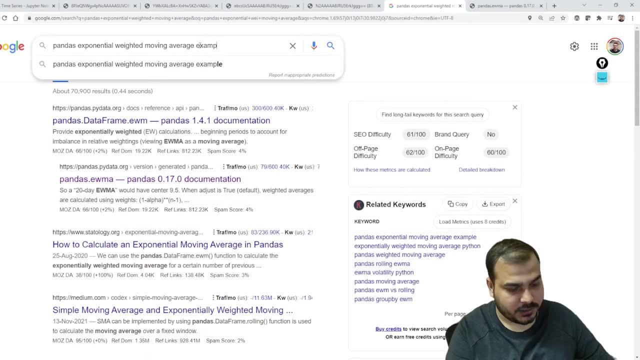 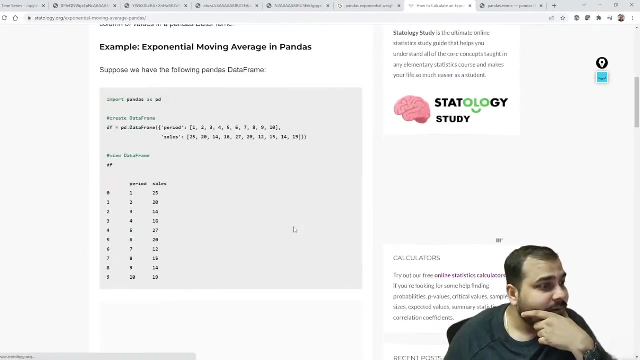 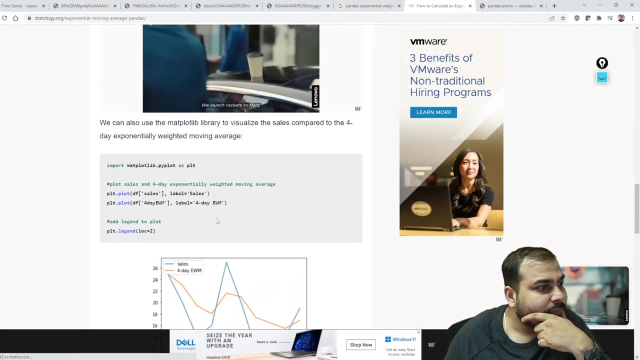 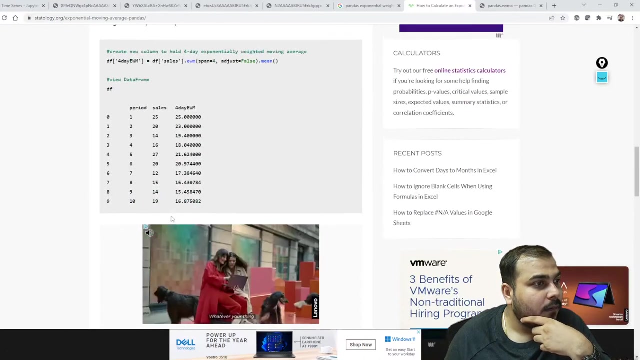 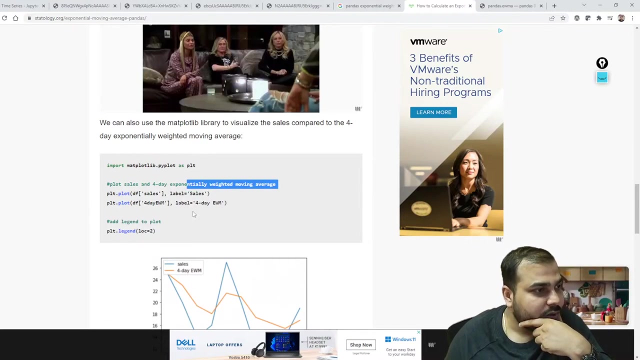 EWM, a EWM, a Example. search for some examples over here. Let's see some. Some solutions will be able to see over here. EWM is only there. Exponential plot 4, soils, exponential weighted moving average, And they have just calculated EWM. Okay, with the help of span we can actually do that. 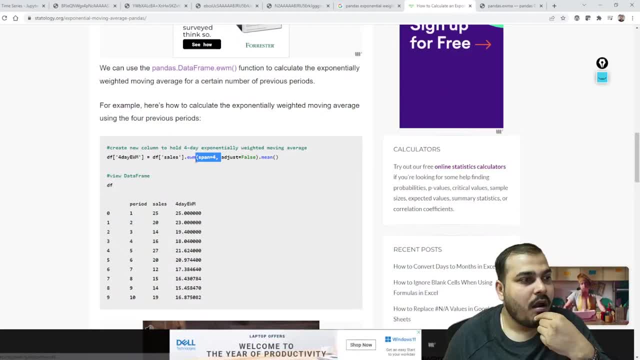 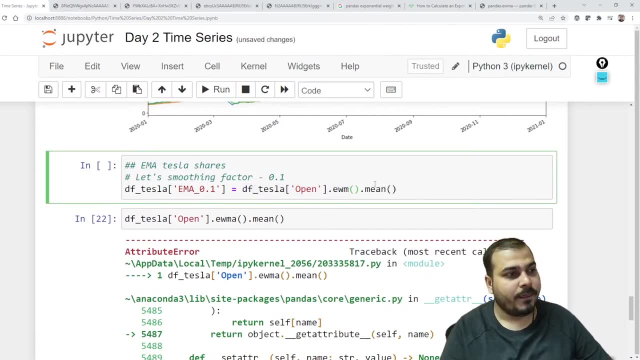 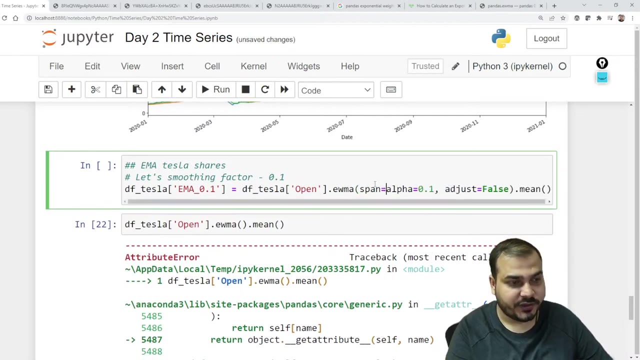 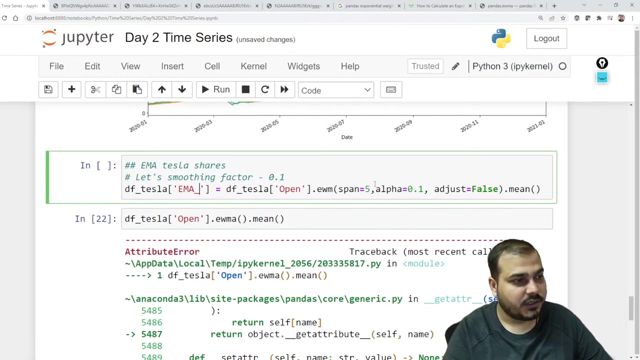 With the help of span we can actually do that. So suppose if I say EWM, And here all the parameters will be almost same: EWM, Okay, alpha, And here I am just going to say span is equal to 5, let's say, And if I try to execute, this will basically be with respect to 5 days. 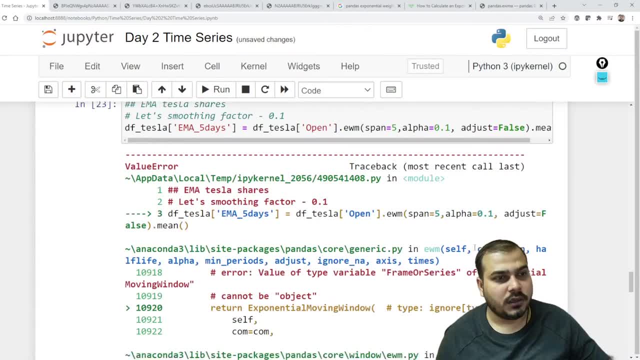 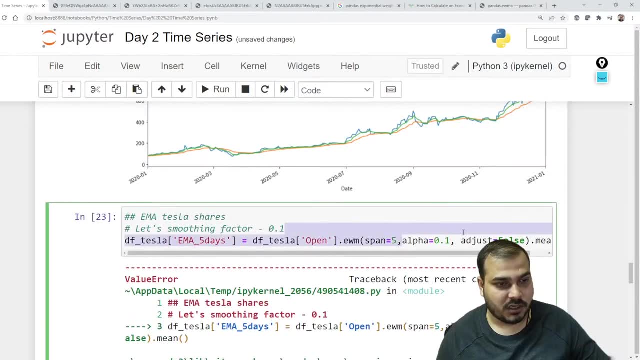 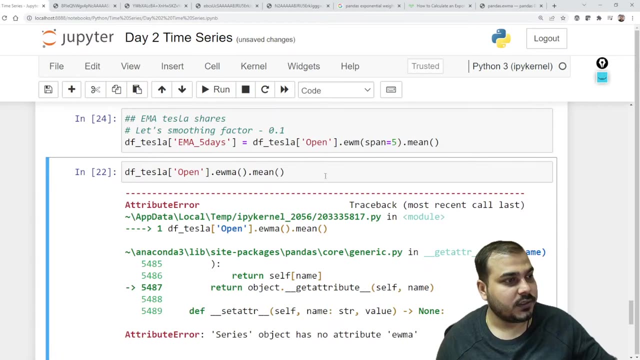 So here you will be able to see some example: Comma span, half-life and alpha mutual exclusive. Okay, Let me remove this. Let me execute it. So if I probably Just plot this, everything Comma EMA, Underscore 5 days. So here you will be able to see dot plot. 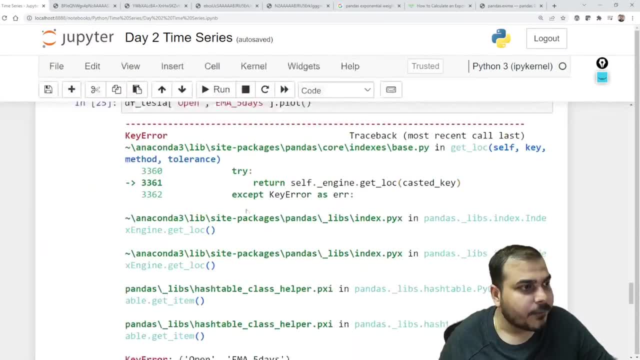 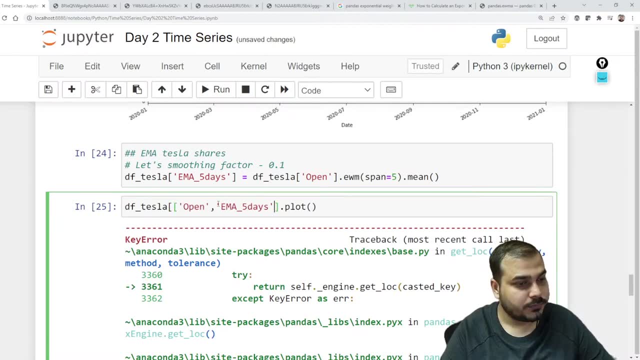 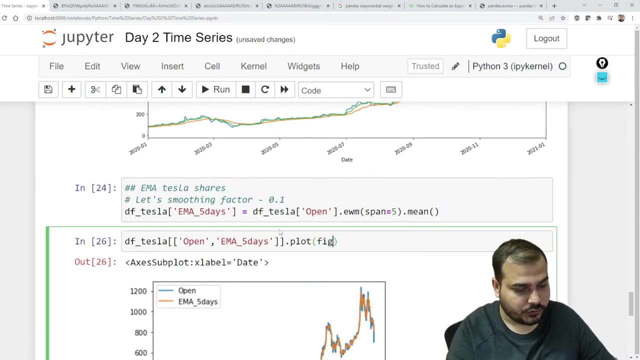 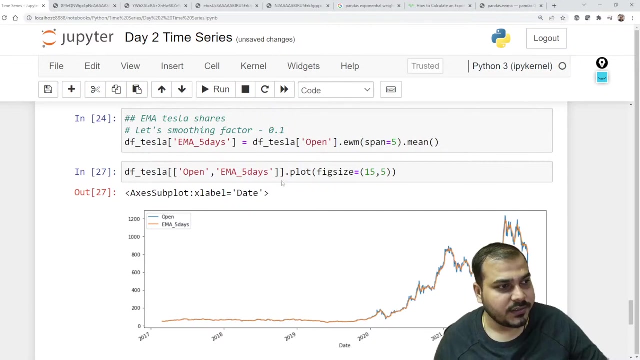 Okay, 2 brackets I have to use, So It looks better. I guess this time I'm just going to use fig size is equal to 15 comma file. Does this look good guys? Let me plot one more thing here. Also, there is no lag. 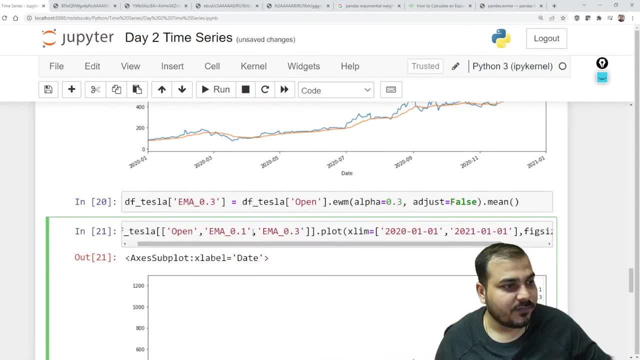 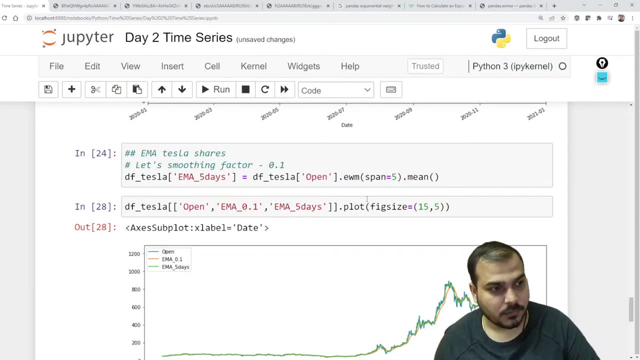 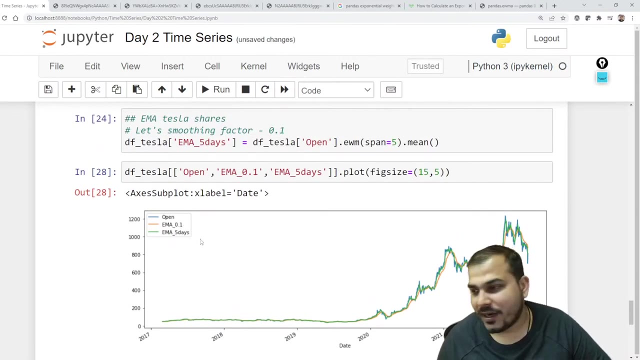 Here also there is no lag, and let me use some smoothening factor also like this. So Here you can see, with respect to green line also, EMA five days and EMA 0.1 with smoothing factor. you can basically use this In general why it's got a span. okay if I write PD dot. 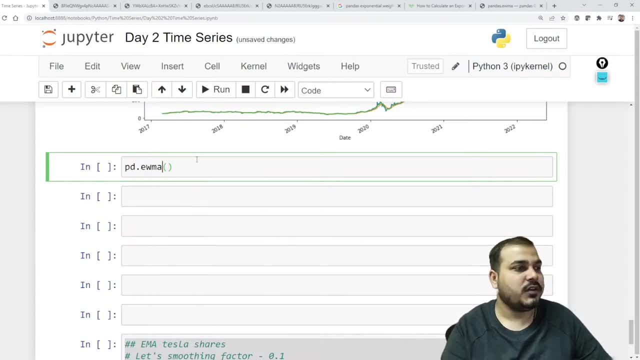 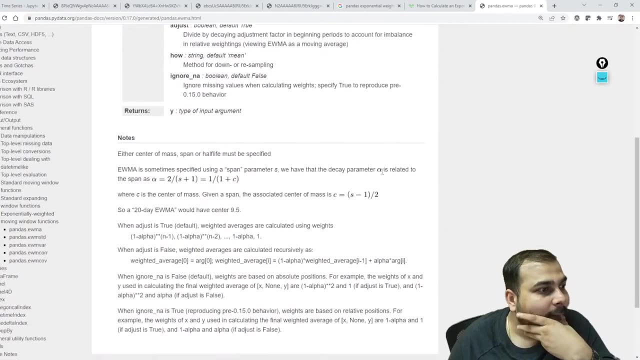 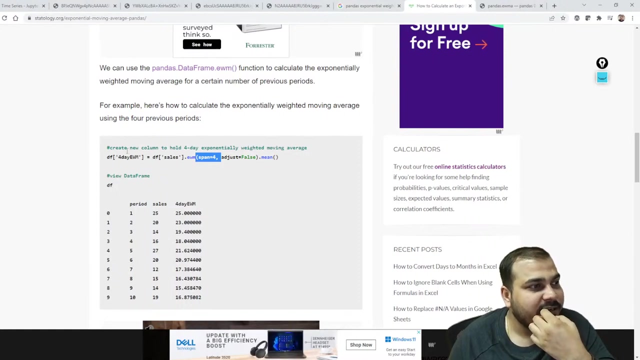 EW. No, PD dot EW, EMA is also not there. I don't know why in the documentation they have given this. how to call this then? Pandas EW, EMA. Okay, fine. So I hope from this article you can definitely see create a new column to: 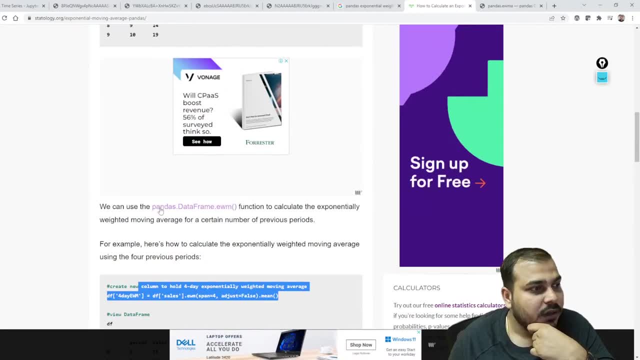 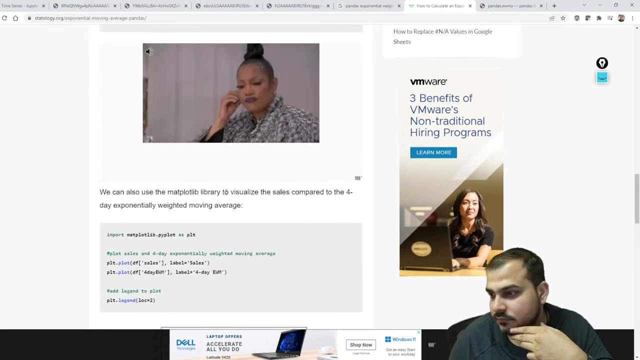 hold four-day exponential weighted moving average. We can use pandas, dot data frame, dot EVMA Function to calculate the exponential weighted moving average for a certain number of periods. So here is given some example. Fine, But I hope you are actually got this idea. if you don't understand what exactly span just for a shift tab. 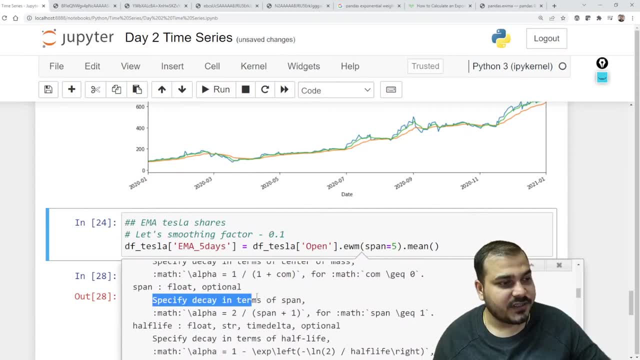 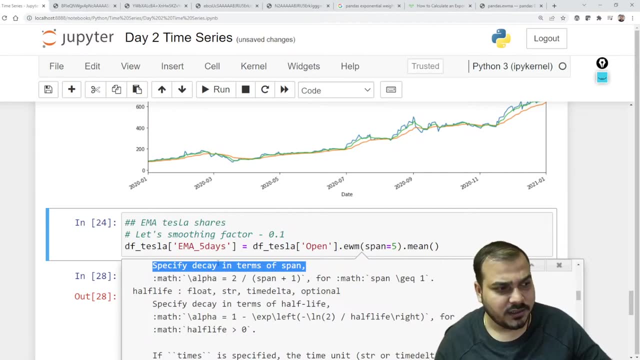 Here you'll be able to see: span. span says specified decay. in terms of span. Alpha is equal to 2 by span plus 1. same thing, the multiplier effect, the same thing. here you are saying, right? That basically means I'm giving the rolling window type as 4. 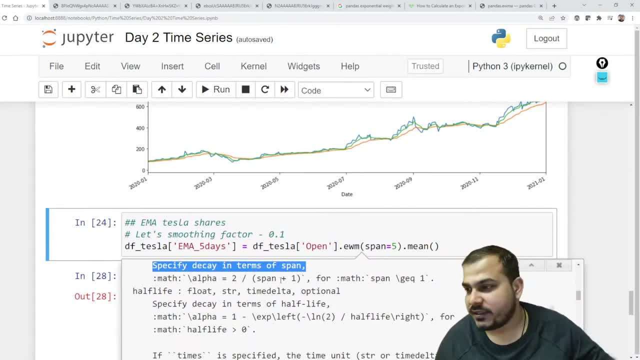 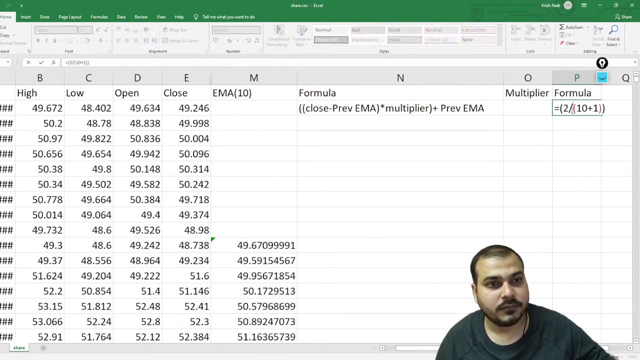 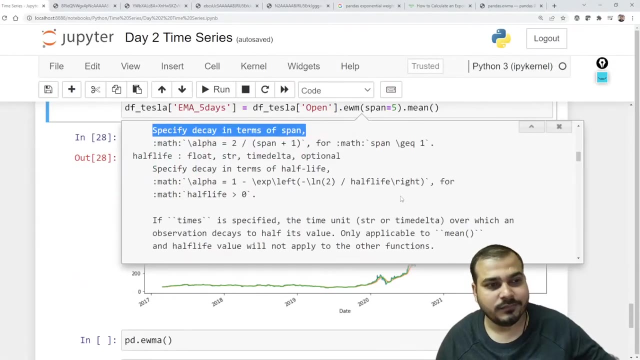 Okay, 2 divided by span plus 1, Which I had actually discussed in the excel sheet. right, This excel sheet does just now we discussed, right? Right, if you want to calculate this, right, everybody, clear Guys, I know This is not that easy. 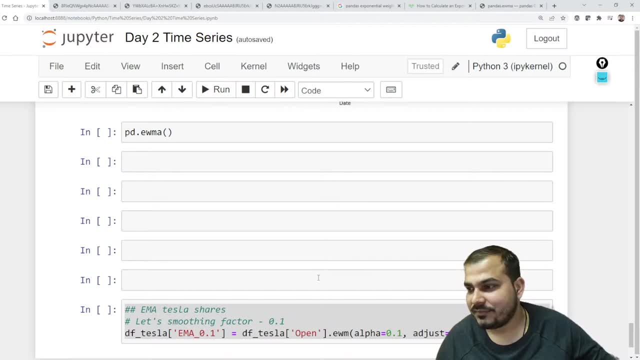 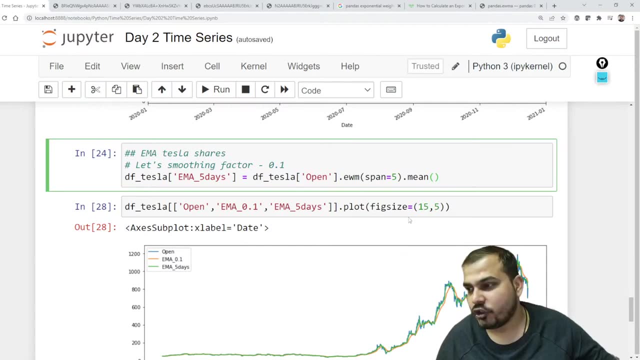 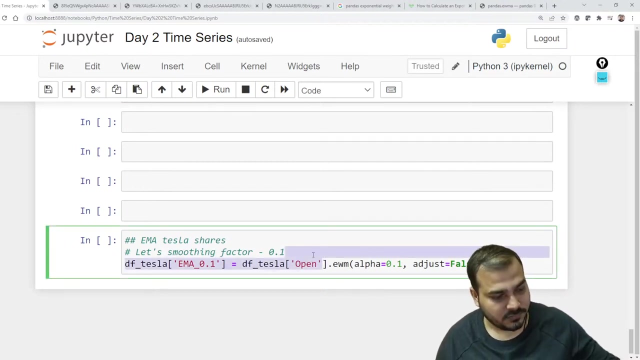 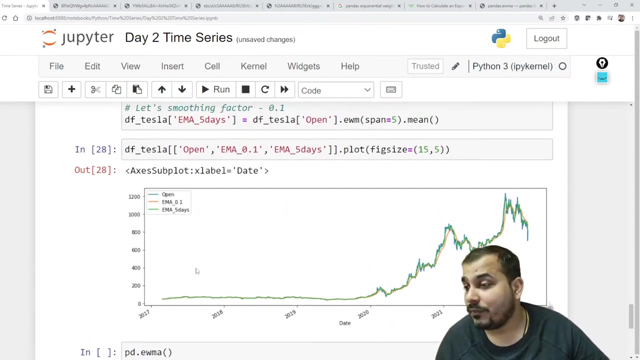 But you have to learn it. Yes, it will be average only when you apply mean right. So, overall, how was the session? guys still here? now we will discuss the most amazing part, Which is the most, which is which moving average is the best. okay, guys, which moving average is the best? tell me. 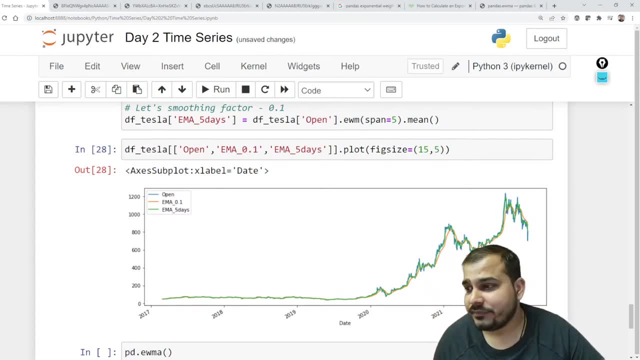 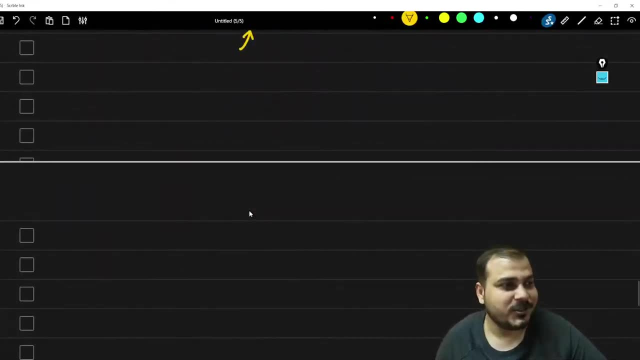 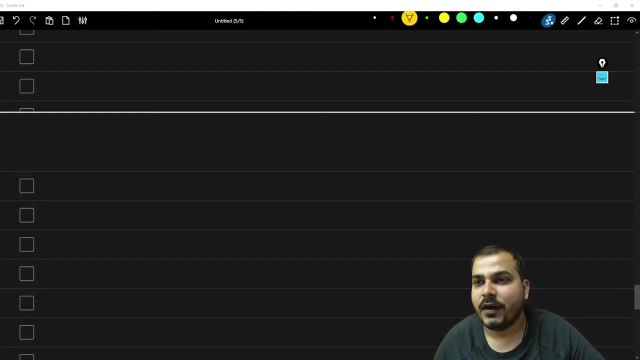 Obviously, Exponential weighted moving average is the best. Right, I know it is difficult, I know you'll scold me for that, Chris, what you're teaching, but through this tool, something is very good. right, You really need to know all the sticks. Okay, Now what I'm actually going to do is that I'm going to talk about moving average model. 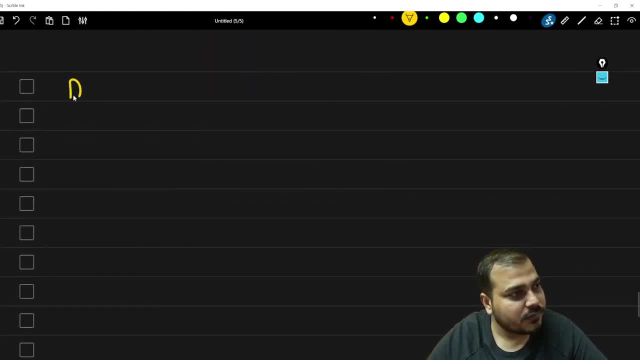 Now in Arima, let's say, in Arima, There are so many important concepts, right? The first thing is AR, The second thing is MA and the initial thing The middle thing over here. I'll talk about this also. Okay, AR is nothing but auto regressive. 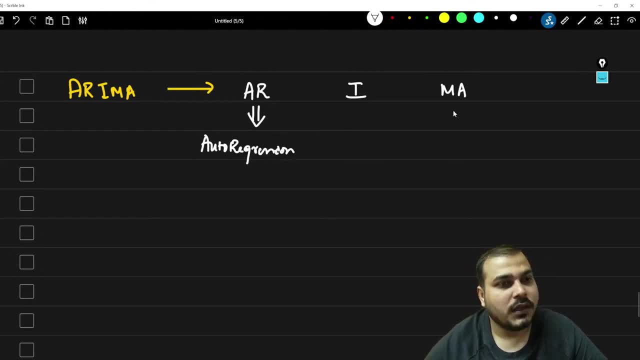 Or I can say auto regression. This is nothing but moving average. If I combine this two, only this two, then it will basically become Arma model. Arma model is good for forecasting Right, probably in sales, Probably in- probably monthly productions- Let's say something. But this will definitely not be helpful in stocks. Okay, don't do it. 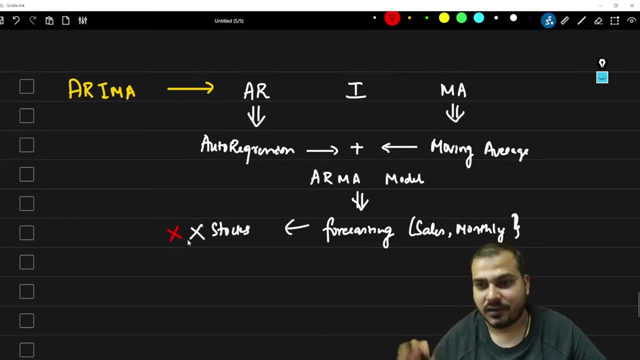 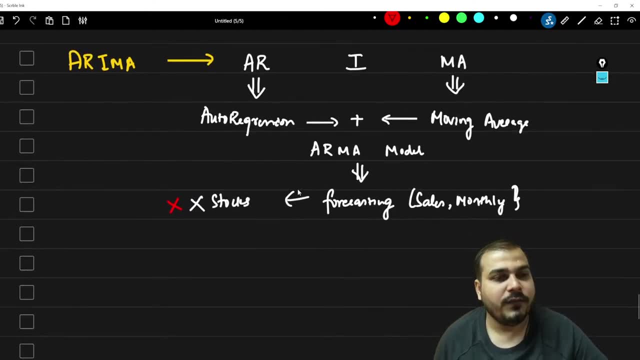 Waste, waste of time, I'd suggest. any model is waste for stocks. Okay, you cannot. if there is any specific model, I do everybody who had become a billionaire at in, Okay. So first of all, what we will do is that we will try to understand what exactly is moving average. 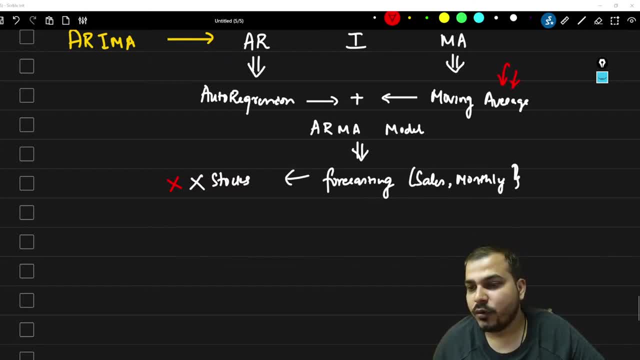 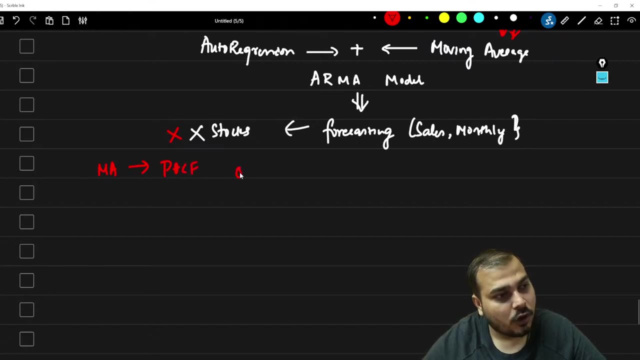 Okay, so what exactly is moving average and how do you basically calculate the moving average and which plots you specifically use with respect to moving average? Okay, one one interview question. They'll say that for moving average Do you use PACF plot or? 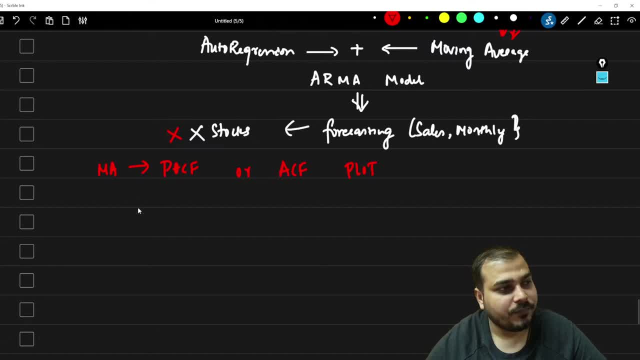 ACF plot. Okay, this can be a question, or they may say you that: okay, Clearly, tell me Where is PACF used and Or where is ACF plot used, whether whether PACF is used for moving average or whether ACF is used for auto regression. 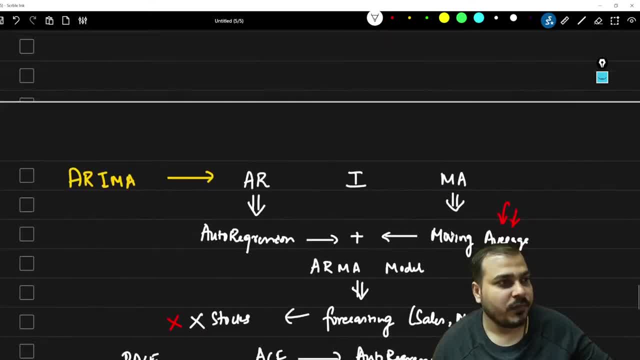 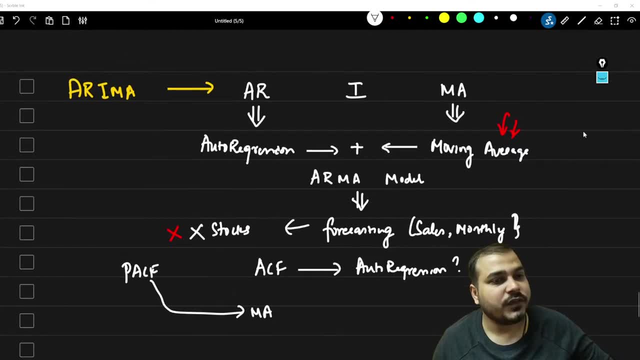 Okay. so this kind of questions may definitely come Okay and probably, if you're working in one, any kind of financial data sets and all okay. So let's go ahead and let's first of all discuss about moving average models. What exactly is moving average models? 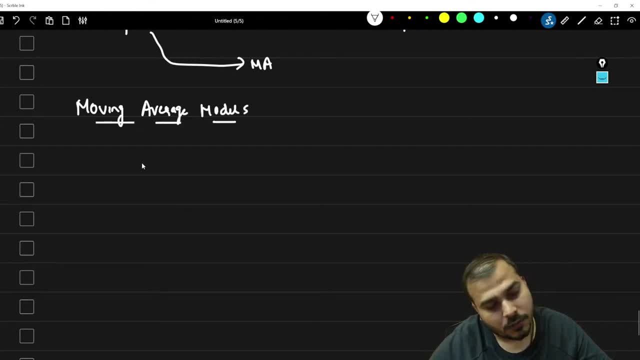 Okay, Everybody shall I start. Yes, You, You, Okay. So moving average models. what exactly it is? Let's say right now what session we are doing it. I'm doing time series, live sessions, right, What I'm actually doing- time series, live sessions- and Obviously, I want many people to join on my life sessions, but people don't understand the importance so they will not join. 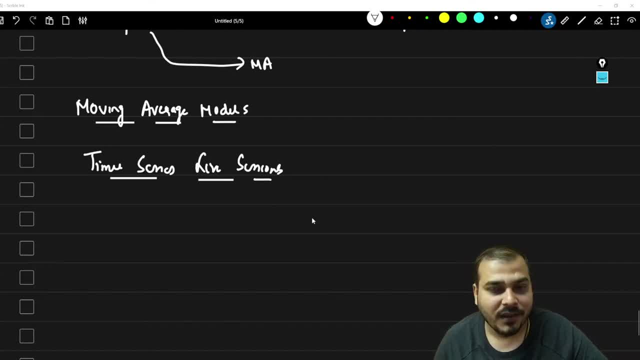 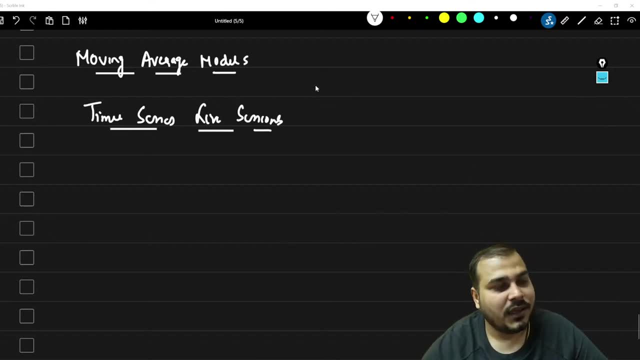 Oh, probably they may be busy in some of the other things. Okay, let's say that my Expectation- if I probably say my expectation in in- with respect to the people attending the live session, let's say it is thousand. Okay, let's say that. 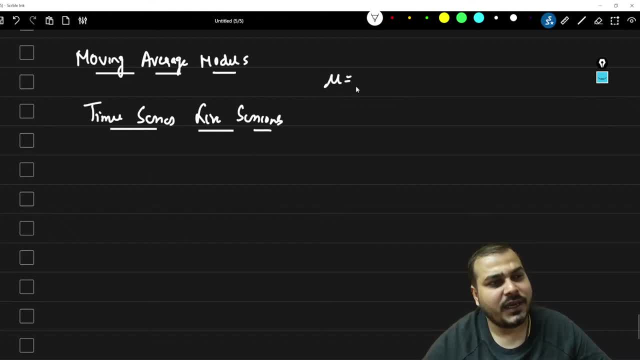 Let not just take such a huge number. Let's say my main expectation, an average expectation of people visiting in everyday's life session, is 10. Okay, just considering an example. so if I really want to Calculate or create this moving average models, My formula will look something like this: everybody focus over here, okay, so I'll say my moving average is: 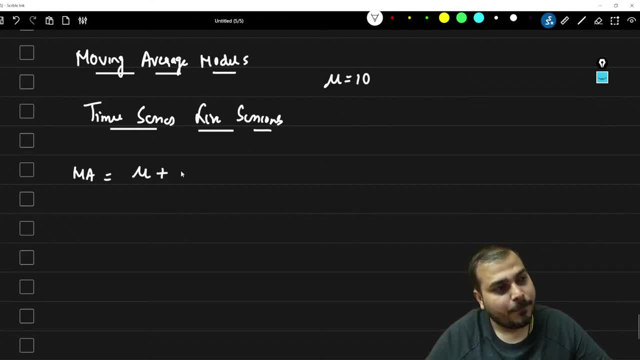 equal to mu plus my one coefficient. I'll write this coefficient as this symbol and I'll say: there will be an error term with respect to the previous timestamp. okay, previous timestamp, there will be specifically one error. now, this is basically my average moving average formula here. you see this, my mean is nothing but 10, okay, I'm saying that. okay, 10 people should come and 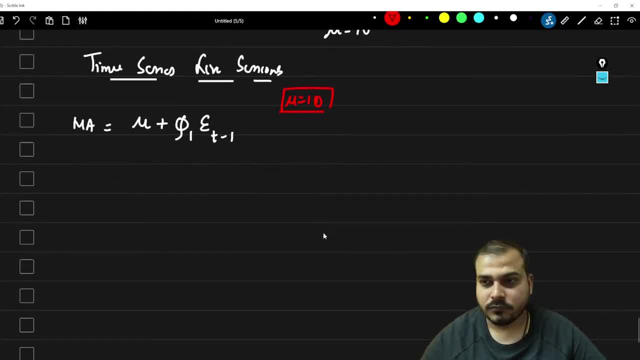 join. that is what is my expectation. let's say here I'm just going to create a specific table. this is my timestamp with respect to day 1, day 2, day 3, day 4, day 5. okay, and here I am just saying that this will be my moving average, because I need to calculate by using this formula. okay, 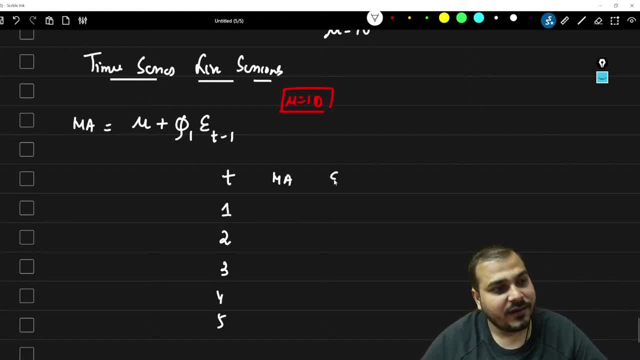 moving average. I need to calculate it, and let's say that my error term is obviously over here, which is specified by this and finally, this entire calculation that I'm actually calculating, let's say that this is my real ma value and this is my predicted ma value. predicted ma value basically means what I'm. 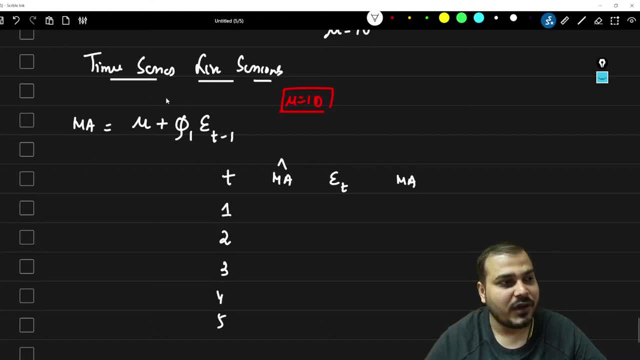 just going to calculate. and now, in order to calculate my predicted ma value, I need to apply this specific formula. okay, very simple. now. this is my real ma value, real moving average value. okay, now let's say that my error term over here is minus 2. it is probably 1 over here, it is. 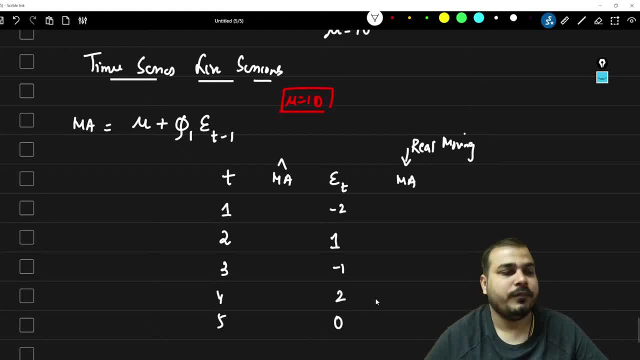 again, minus 1, it is 2, it is 0. okay, now, this basically means what? okay, and let's consider that my initial coefficient that I am assigned is 0.5. okay, so this all I have actually initialized this parameters and all, and always remember this, this values that you'll be seeing, okay. 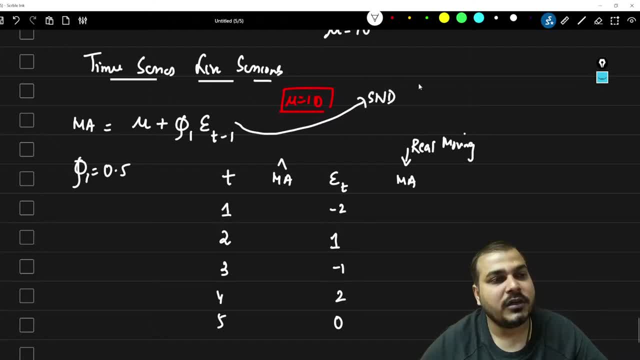 this value. it will belong to a standard normal distribution where your mean will be specifically 0 and your standard deviation will be 1. okay, so this error term that you are able to see. it belongs to a standard normal distribution where your mean is equal to 0 and standard. 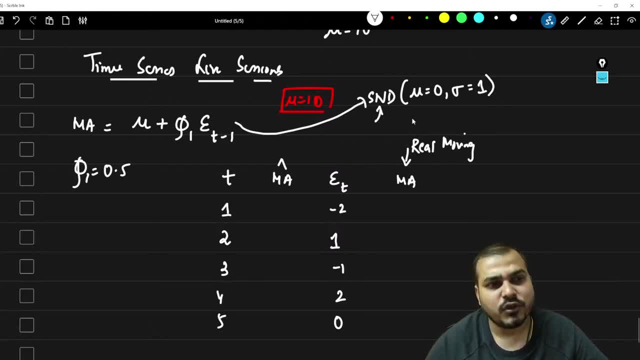 deviation equal to 1, so you will be able to see this specific data, mostly similar to this: everybody clear till here. everybody, yes, yes, yes, everybody clear till here. yeah, yes, everybody clear till here. yeah, yes, yes, guys clear till here. just give me a quick yes so that I further do the calculation with. 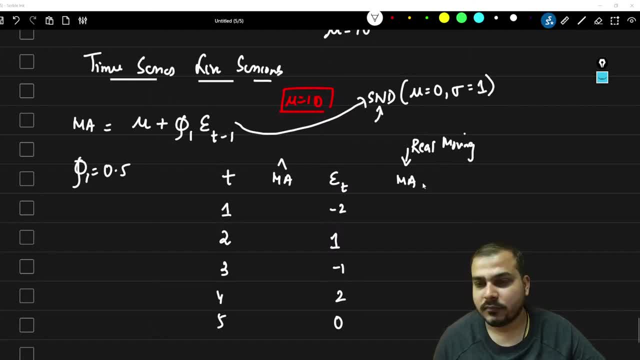 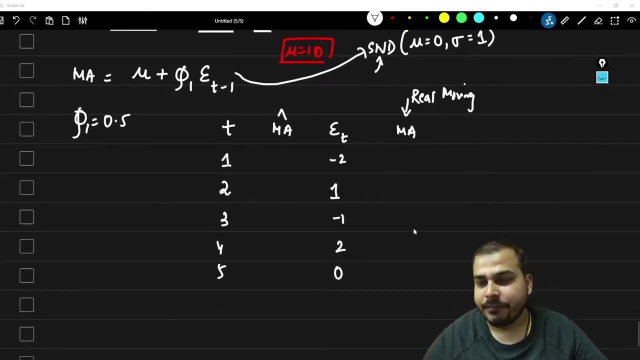 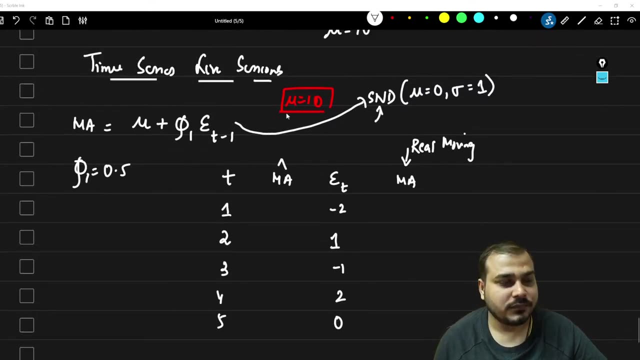 respect to moving averageima L moving average. ok, now tell me, suppose I was expecting 10 people to come. probably 10 people to come, probably. ok, now tell me I was expecting 10 people to come. but let's say the real, real value that came was somewhere around. 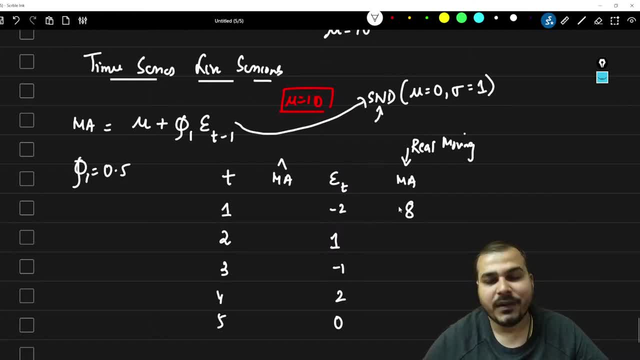 8. if I'm getting 8 people who are attending day one live session, then what will be my this value? think over it. it will be 8 plus 0.5. the error term will be minus 2 right, because I was expecting 10. 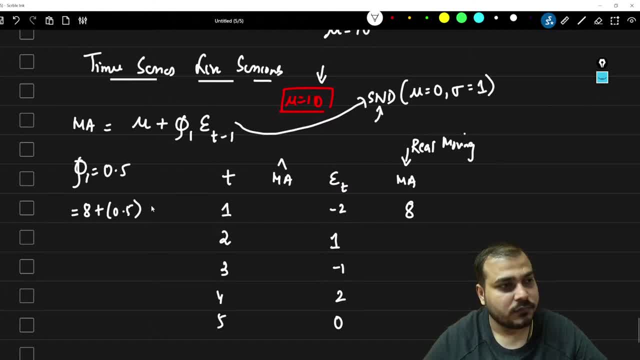 so 10 minus 8 is nothing but minus 2. sorry, 8 minus 10 is nothing but minus 2. so here, if I calculate it, so here you will be able to see that I'm actually getting how much. how much I'm getting 8 plus how much I'm actually getting guys. 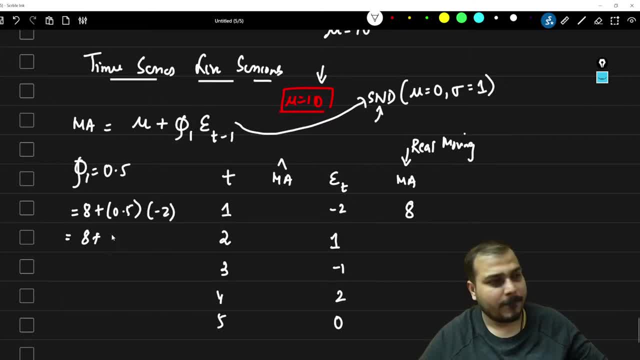 8 minus 2. that is for this specific term. okay, just a second. okay, okay, just a second. so my initial prediction was that I should be getting 10, but I got 8. and here I'm: the error term is minus 2. okay, now, in order to calculate the moving average. 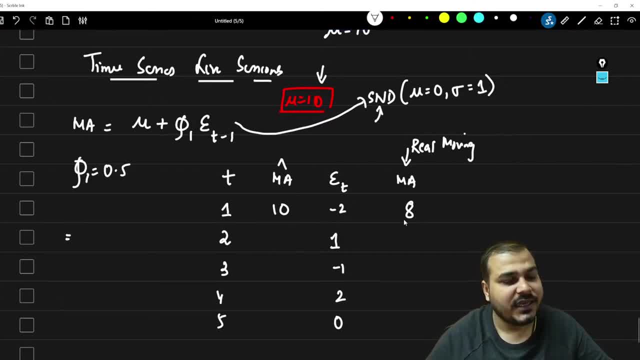 based on the moving average model for day two, I will just say that, okay, fine, my moving average mean was basically 8. okay, just a second, should be 10, 10 plus 10, 10 plus. what is this value? this value is nothing but 0.5 and this value is now error, of error of. 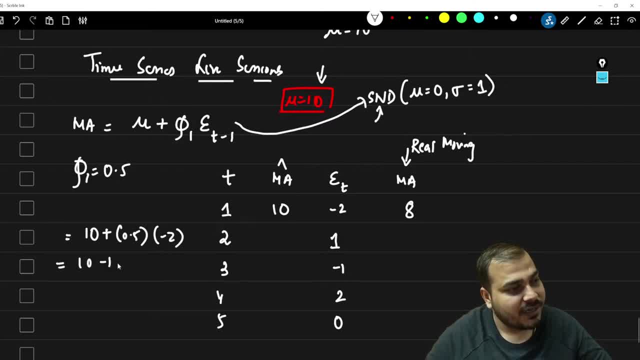 this specific value. so it is minus 2, so 10 minus 1 will be what 9? so am I getting 9 over here? everybody just see this. am I getting 9 over here? yes, now, since I'm getting 9. okay, but I was. 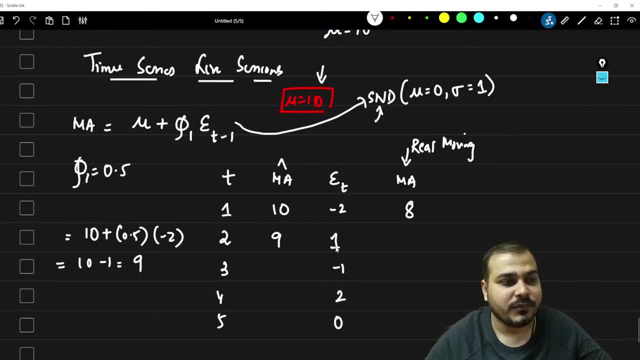 expecting still 10 value. so if I probably do 10 minus 9, I'm actually getting the error value as 1 right. so here my real moving average should be 10, but I'm actually getting 1 over here as my error difference. is everybody clear with respect to this? 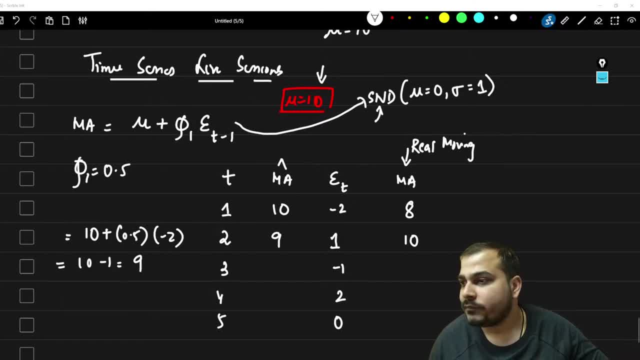 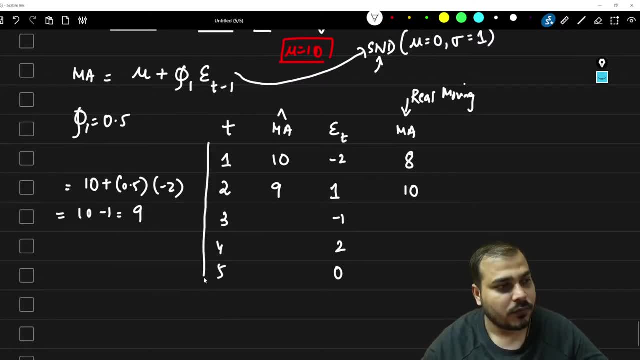 yeah, coefficient is just initialized. don't worry, right now I'm just trying to calculate this. now, do this similar calculation for all the other things, guys. okay, if my error is minus 1, what does this basically mean? if my error is minus 2, that basically means that I'm getting 10 over here. 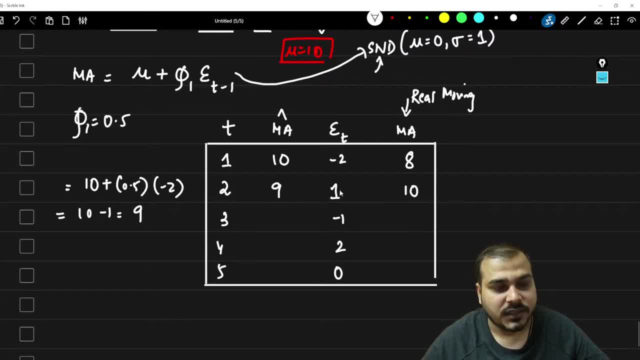 basically means 8, right? see this. if my error is 1, what does this basically mean? this basically means my value that I am assuming, right? you will be able to see that over here. it is 9, right? if I'm value is minus 1, what do you think by this? how much value will probably? 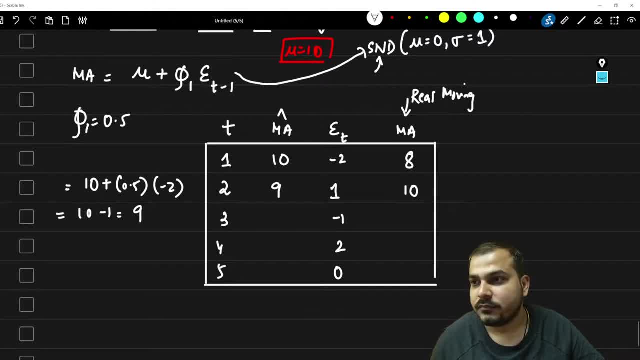 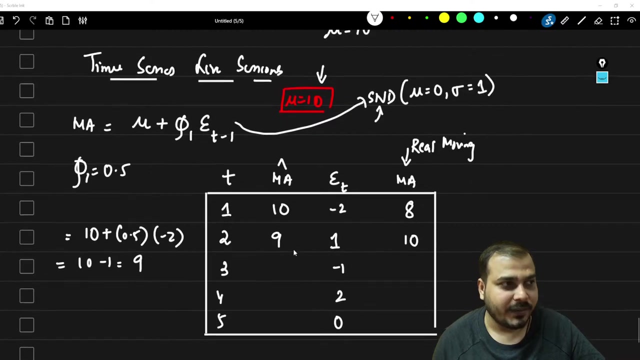 be, I'll be getting in, ma just tell me ma prediction. okay, okay, just write in it. so, as of specific table, I'll repeat it. just write it down, this specific table, I'll repeat it. I'll repeat it, don't worry, I'll repeat it. okay, let's. let's do the one. We can do our experiment. 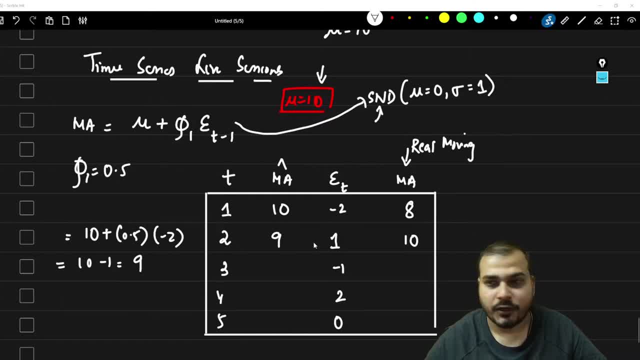 thing. let's do Maserati vendetta, two, three dollars point chargefeett, 10 to 10 digamos, to let's do this thing that I'm actually trying to do. Okay, just a second, Don't worry, I will do it again. 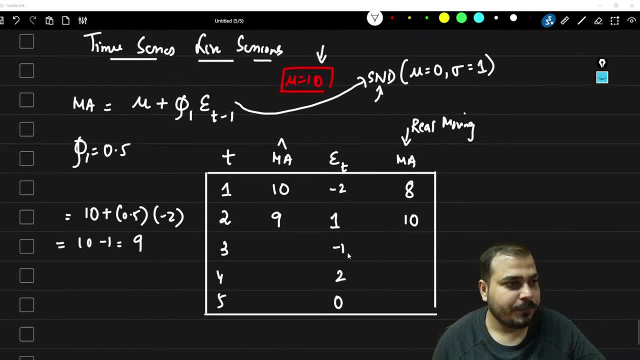 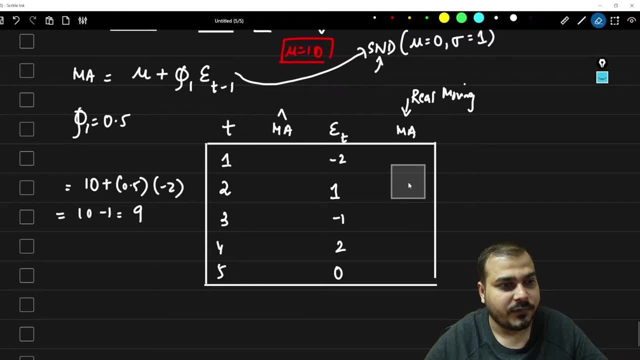 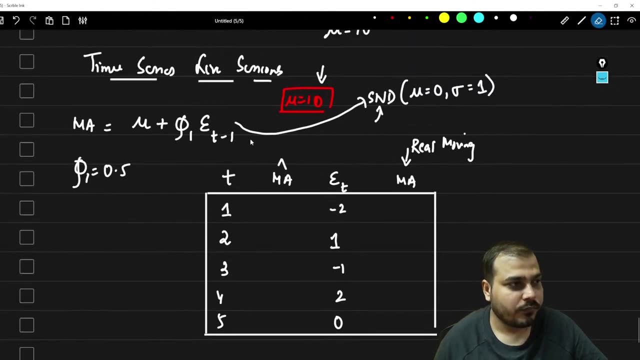 Okay, everybody's ready. now, Again, I will try to do it for you, okay, Okay, let me rub this again. Let me rub this, let me rub this and let me rub this, Okay, Okay, now let's calculate these values, okay. 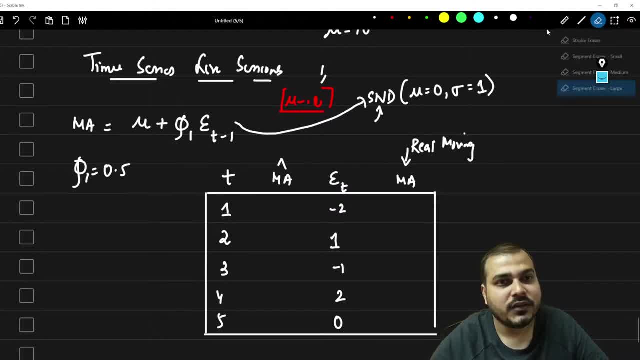 Initially, you know that I'm expecting that I will be getting- mean is equal to 10,. right, Let me rub it again for you. Let's assume that my initial value that I want to calculate for m a hat- m a hat basically means predicted one, okay. 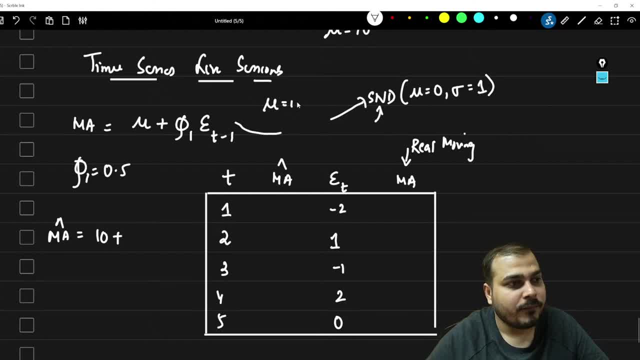 Let's say, my 10 value is there. obviously I'm expecting 10,. okay, I'm expecting 10, but over here, my error is minus two. okay, If it is minus two, then what will happen? 0.5 multiplied by minus two- right? 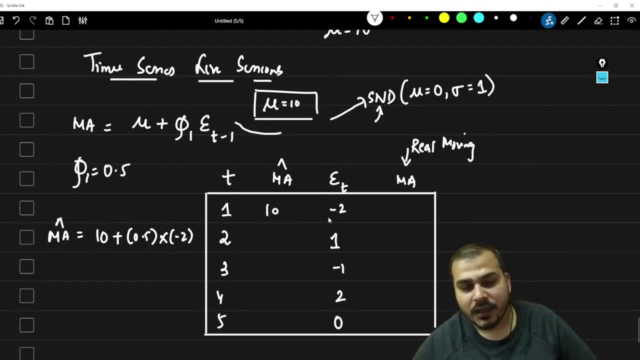 Over here. if I see this is my 10. initially I want the 10 over here, But since I got as minus two as my error, obviously my moving average will become eight, because 10 minus two will be eight, right. 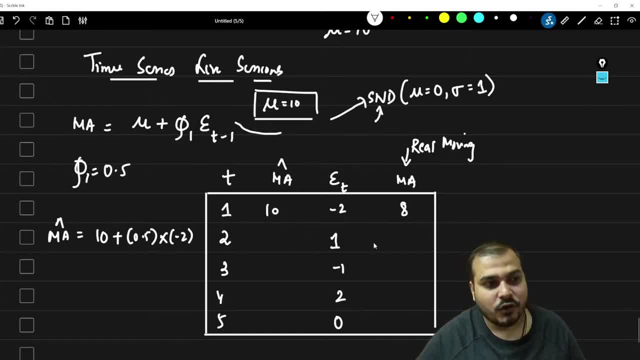 10 minus two will be eight. Now, in order to calculate this row, 10 minus two will be eight. right, 10 minus two will be eight. Now, in order to calculate this row, m a hat, I will be using the previous m a hat values. 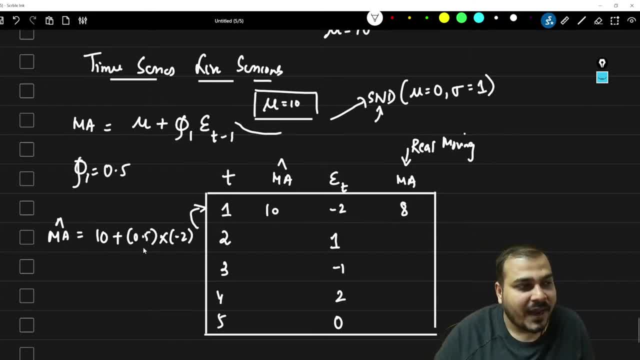 And in order to use this, what I will do: 10 plus minus 0.5, 0.5 minus multiplied by minus two. So if I do this, this will basically get- I'll be getting- as nine right. 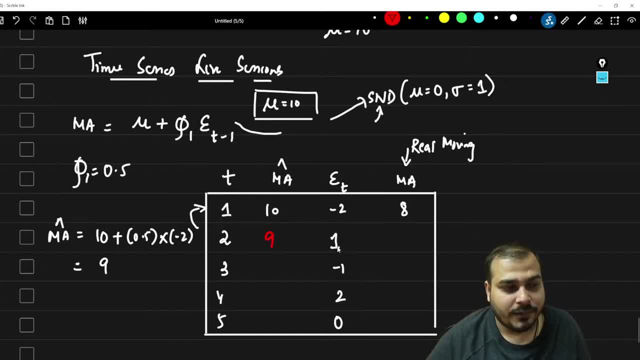 So if I probably get nine over here, but my error rate is one, So if my error rate is one, nine plus one will basically be 10 over here, right? So this will basically be my moving average. It would have been 10,. 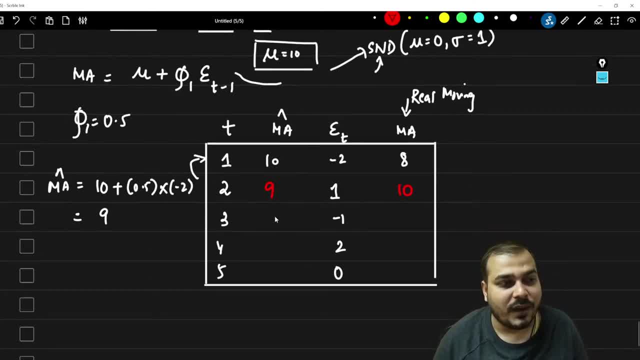 but because of this specific error, I'm getting this Now in order to calculate the third one. in order to calculate the third one, what I have to do, I can do it for m a hat for third row. So, in order to calculate it for the third row. 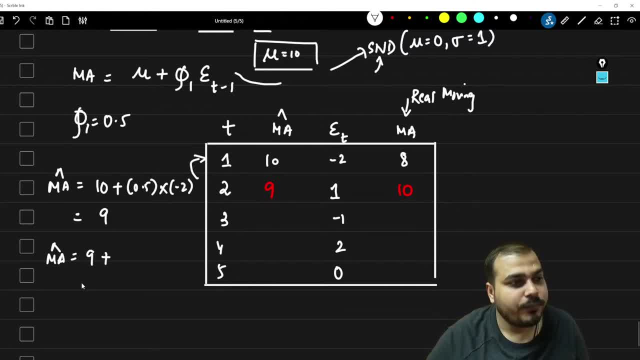 what I have to specifically do is that I will take this nine value plus minus 0.5, sorry, 0.5,- multiplied by the previous error. The previous error is one, So this will basically be 9.5.. 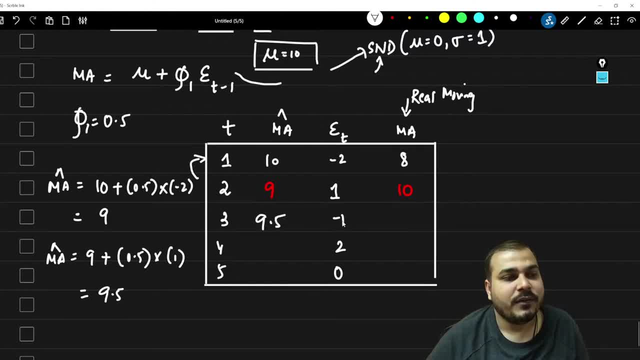 So if I'm actually getting 9.5 over here- 9.5, 9.5 minus one- how much it will become? then? How much it will become? Tell me, 9.5 minus one, Is it 9.5?? 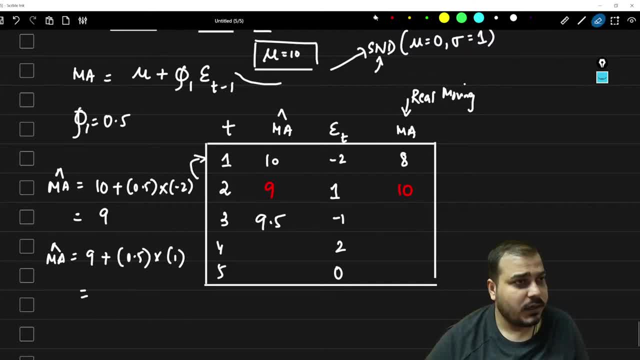 Sorry, it is 10.5.. My mistake, It is 10.5.. So 10.5,. so here I'm actually going to write it as 10.5 minus one will be nothing but 9.5, right. 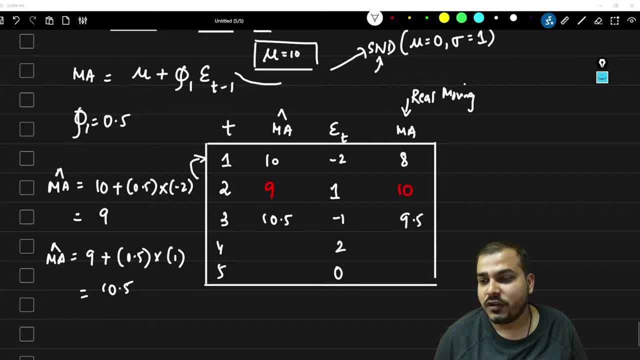 Based on the error. okay, Based on the error. Everybody, focus on the error and based on that, I'm actually going to write it as 10.5.. That's what I'm actually trying to calculate right Now. similarly, if I want to calculate the fourth row, 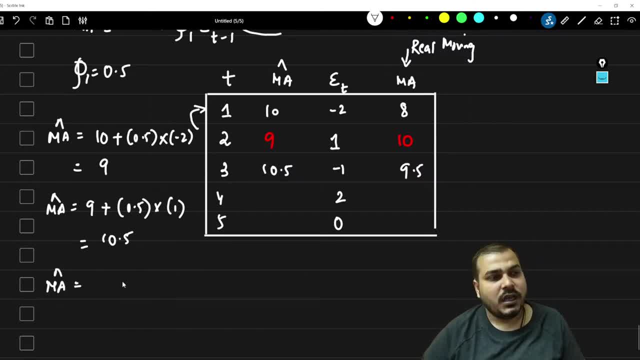 of the moving average with the help of moving average model, then what I'm actually going to do? I'm going to basically take 10.5 plus 0.5, multiplied by minus one- This was the previous error, So if I probably write 10.5 minus 0.5,. 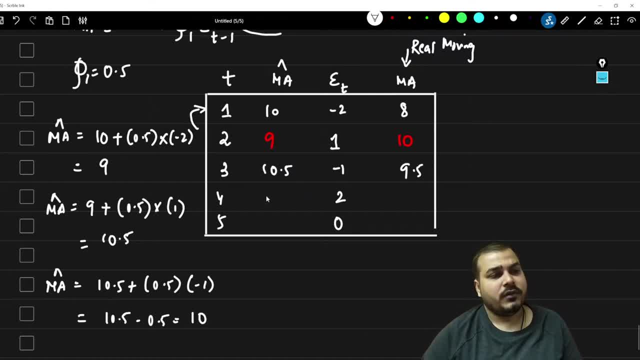 which is going to become over here as 10.. So 10, if I'm actually getting prediction. so the error term is basically two. So 10 minus two will basically become 10 minus two will basically become sorry. 10 plus two will basically become 12, right. 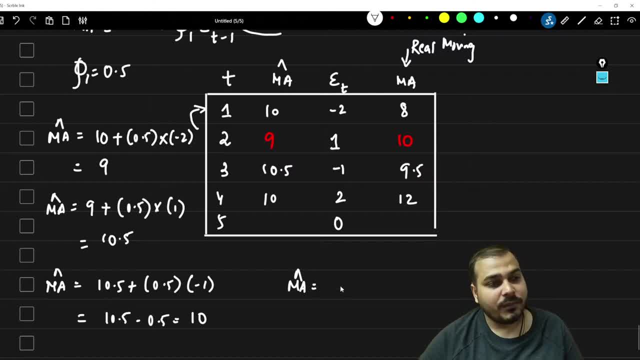 And similarly, if I try to calculate the last row, so here you'll be able to see, the previous value was 10 plus 0.5 and multiplied, by error as two. So 10 plus one is equal to 11 and 11 plus zero is equal to 11.. 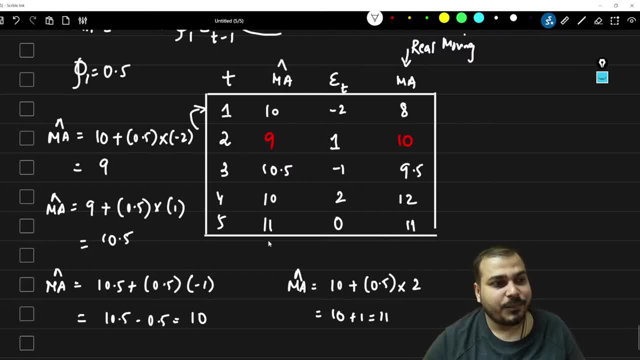 So this is the expected and this is the predicted right And this is the error term. This is the error term. If we are getting minus, that basically means the expected was 9.5, but we got 10.5, okay. 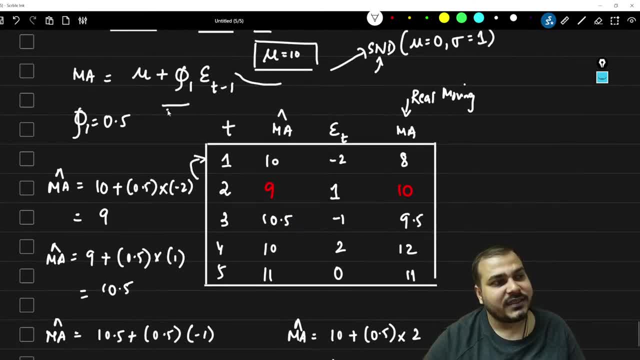 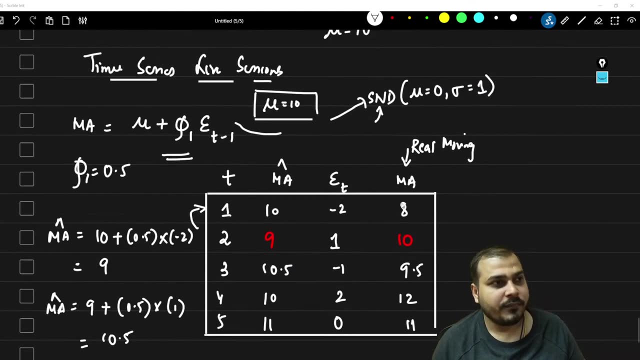 I hope everybody's able to understand- And this is the same formula that gets applied with respect to finding the moving average. A calculation mistake where guys- Let's see this, Let's say I get a 10, right Initial error rate is mostly about initializing. 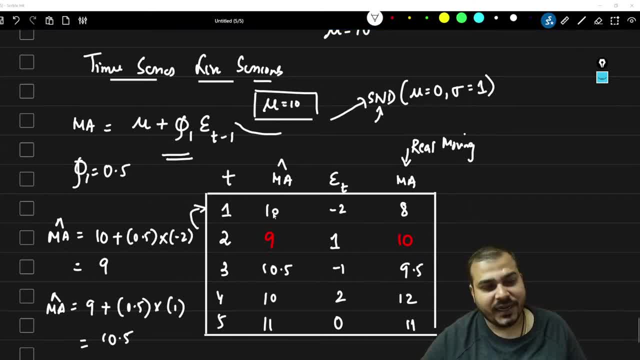 See, I was expecting 10,. okay, I was expecting 10, but over there, what happened? People- probably people came as eight. See, I was expecting that 10 people will basically arrive in my live session, but only eight people came. 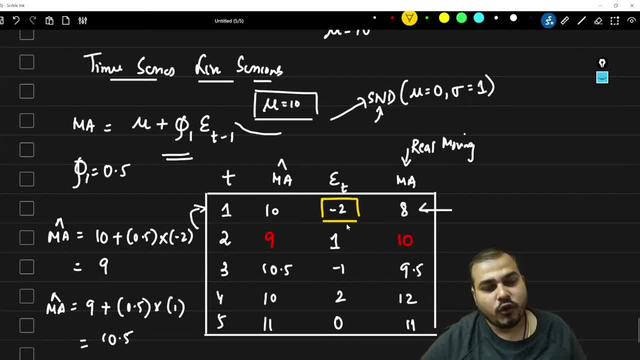 So I'm getting an error rate of minus two right Now, tomorrow's. if I want to calculate the moving average with the help of this moving average model, then what I will do, I will just apply this formula. So I have applied this formula for this. 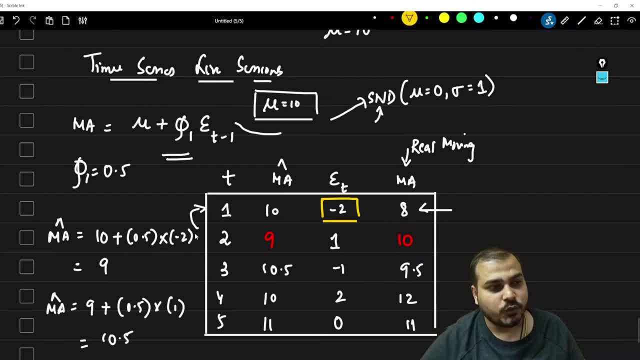 See 10 plus 0.5 multiplied by minus two. So this will be 10 minus one. 10 minus one is nothing but nine. So tomorrow I'm expecting that at least nine people will join Now, if I get an error rate of one. 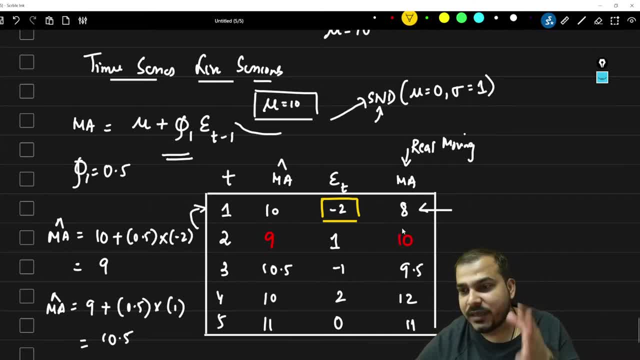 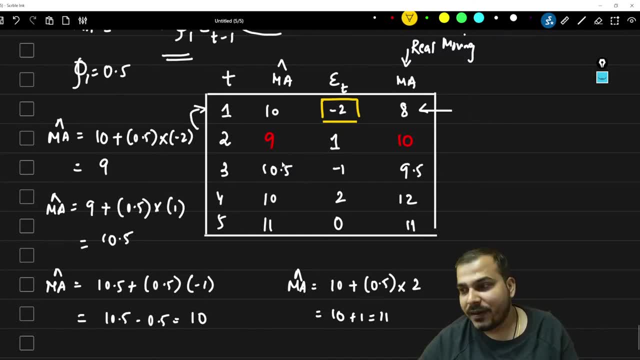 this basically says that 10 people had actually come to see my live session. okay, Then, similarly for the third place, what I'm actually doing, again, I want to see that how many people are going to come. So, again, I'm going to calculate the moving average. 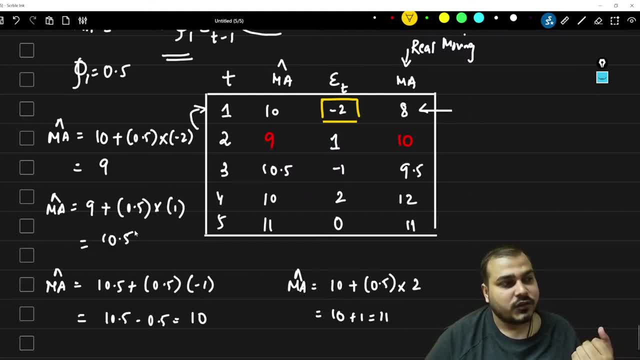 Now it'll be nine plus 0.5.. I'm going to calculate the moving average of 10.5 multiplied by one. So here I'm actually getting 10.5.. I'm predicting that 10.5 people will come. 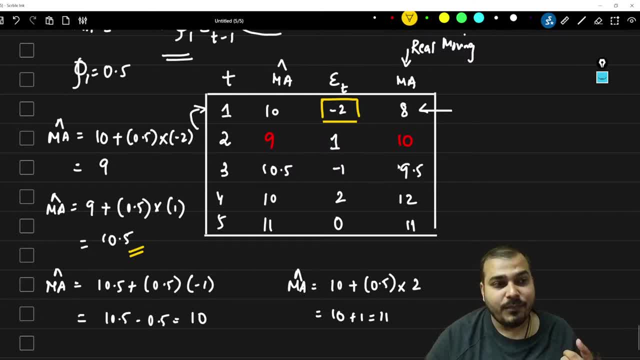 but how many people actually came because of this error rate? Only 9.5, right, 9.5 people had actually come over here Now, when 9.5 actually people had come. obviously it is sorry this should be 10 minus one. 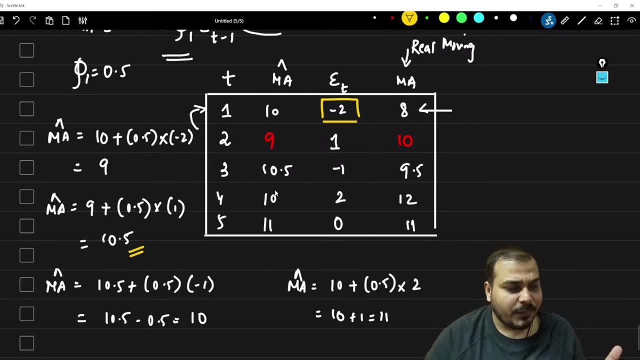 Okay, 10 minus one- 9.5.. 9.5 people had actually come. Then, coming to this next one, I need to calculate this, So I'll be using 10.5.. That's 0.5 minus one. 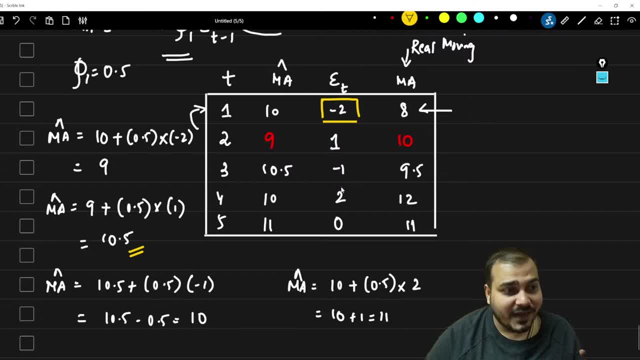 So here I'm actually getting 10.. So if 10 is, then if the error rate is two, that basically means I was expecting 10 people are actually going to come, but 12 people actually came And similarly, I'm going to calculate this similarly right. 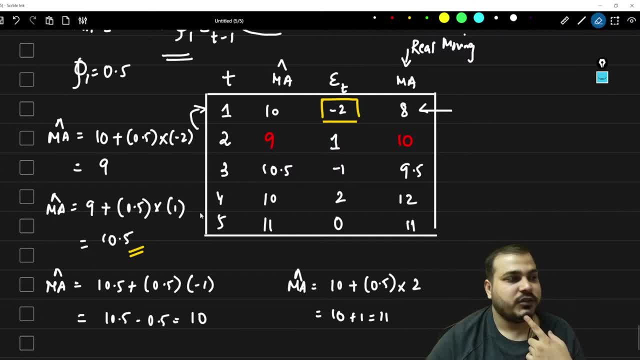 Nine. okay, So one calculation was wrong. you said right 9.5.. Okay, fine, my mistake. So here I have 9.5.. So 9.5 minus one, it is nothing but 8.5.. 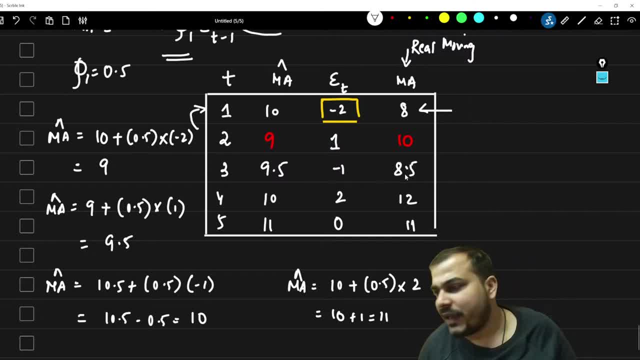 This is 8.5.. Now is it clear. I think now the calculation is perfectly fine. Here I made one mistake: It could be 8.5.. Yes, 8.5 is here. no How to know value of ETA1.. 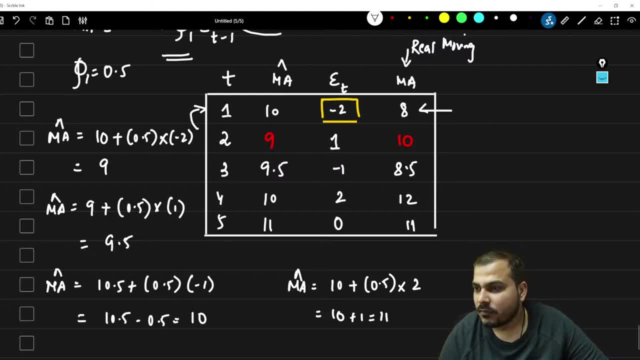 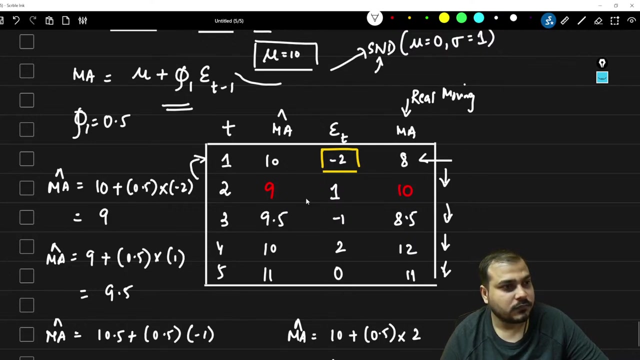 What ETA1?? Okay, Yes, To calculate the next data point with respect to moving average. we are focusing on calculating this. okay, With respect to this moving average model. So we basically say, right, This is the moving average, But don't worry, tomorrow again I'll repeat this. 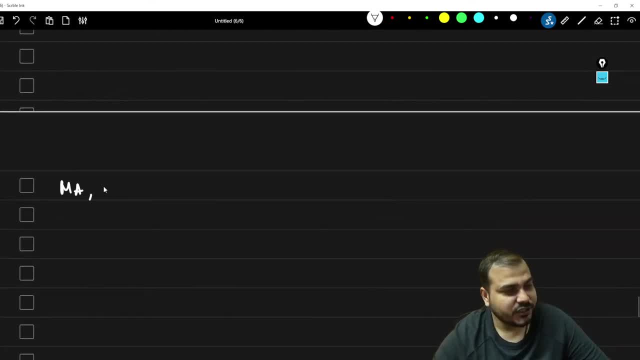 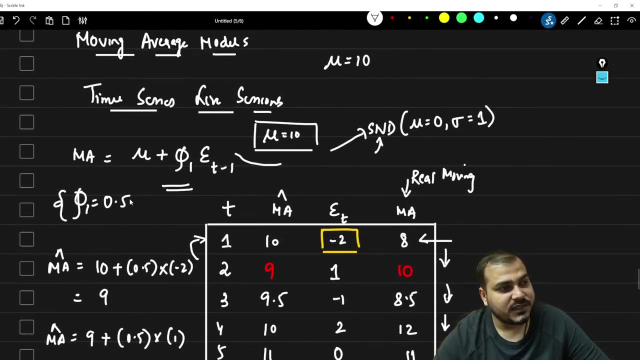 because I really want to consider taking moving average autoregressive and that I value This three. I will define it theoretically and probably give you a lot of problem statements to solve. Okay, Why this particular value is 0.5?? 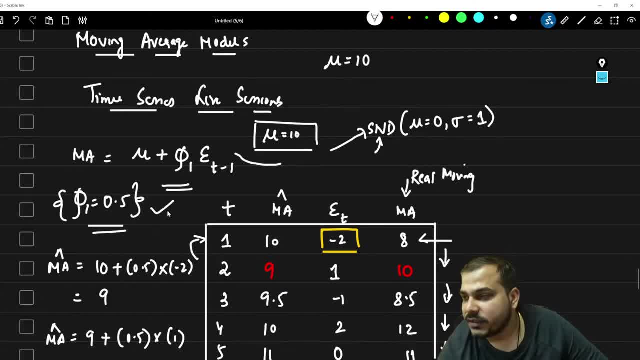 This is just like a hyperparameter you can consider, And I'm actually going to consider this. Go and call the support team, okay. Go and check the support team. The number is given in the description. Go and check it out, okay. 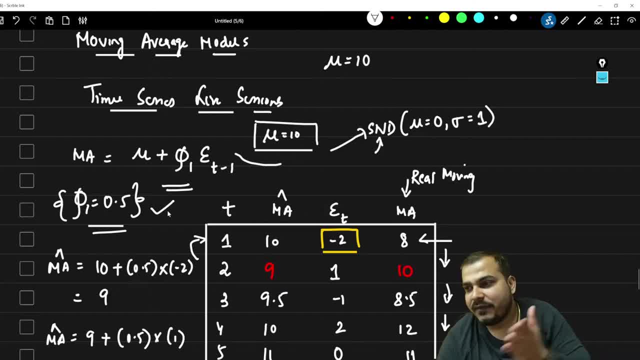 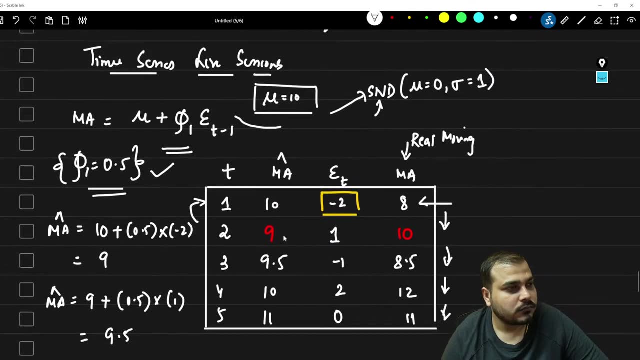 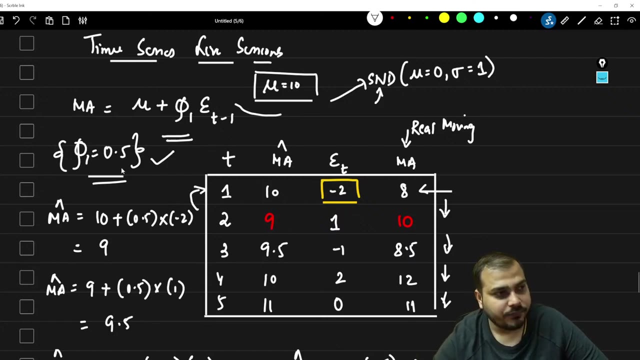 Go and ask the team. They will let you know everything. Every time the same person is asking the same question in the live session. Yes, Anurad, You're absolutely right. Okay, So I hope everybody has understood this. it is a hyper parameter, guys five. okay. 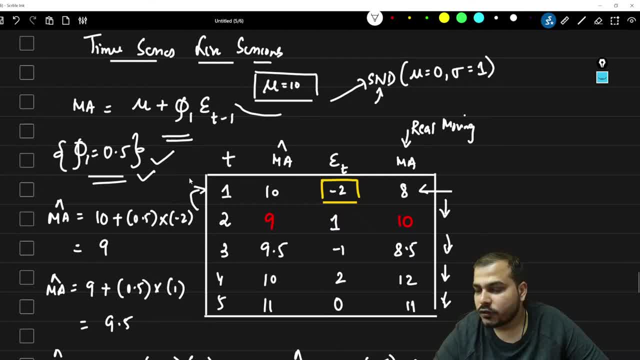 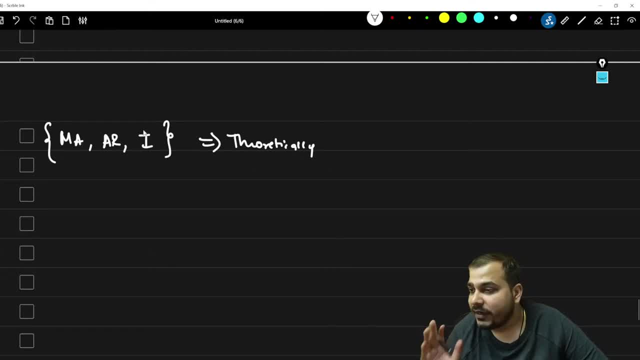 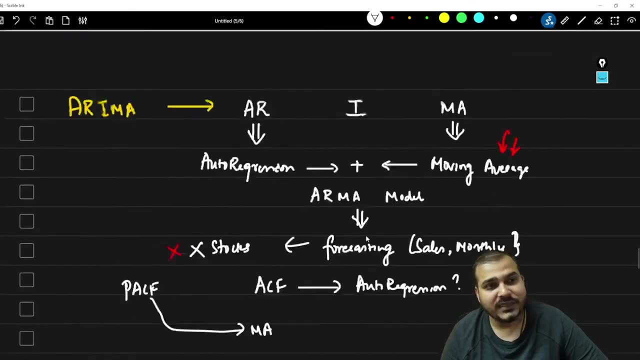 so let me do one thing. tomorrow, uh, we will again repeat this moving average auto arima- and this i value. we will try to find out, in an amazing way, what exactly it is and how we should basically go ahead with okay, so today i'll just end the session, because we have discussed many, many 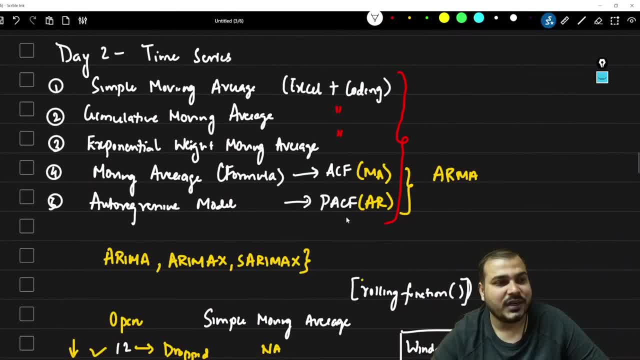 things today and we are just in starting things. i thought that i'll try to cover this acf, pacf, you know, but don't worry, till here we have covered completely. i've given you the introduction. introduction of moving average models. all right, so moving average models, again tomorrow will be.